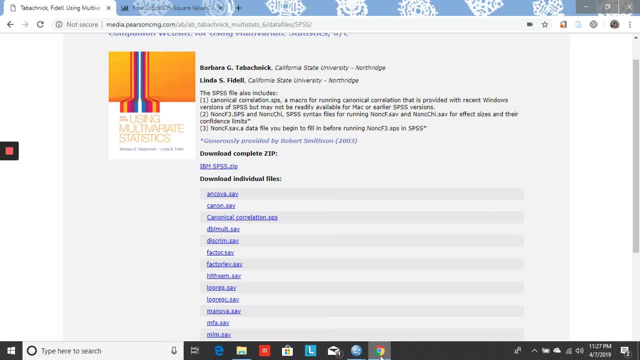 Hi, my name is Kristin Kinsevich and I am a doctoral student at Regent University. Today we're going to be walking through the complete example in chapter 13 of Tabachnik and Fidel, using multivariate statistics. I am using the 5th edition, so the page numbers, if I 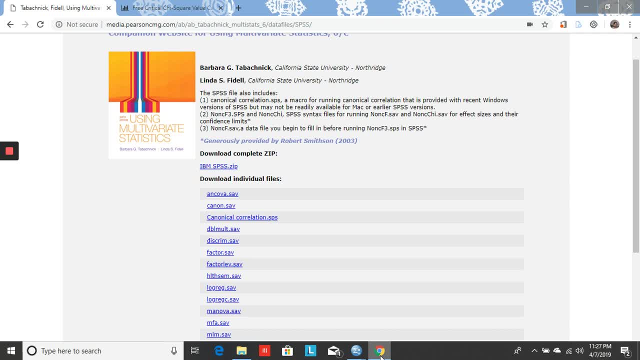 refer to them will be from the 5th edition, and I'll try to refer to sections as they might occur in the 6th edition as well. Today we're going to be using the factor data set, So it's listed right here. You can see. this is the website that goes along with the textbook. 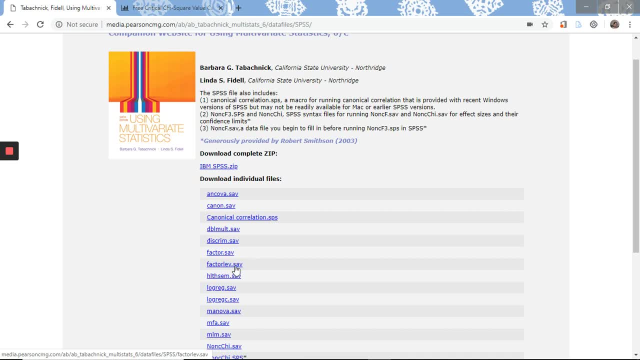 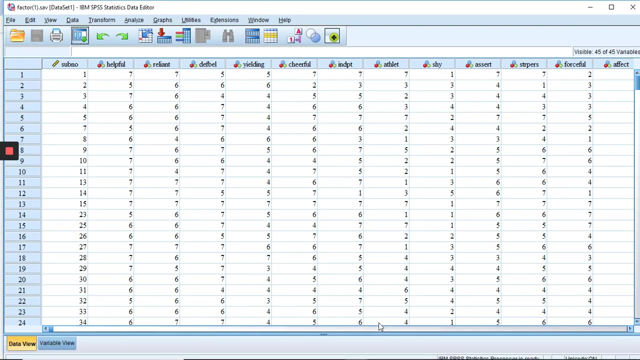 And this factor L-E-V is ones with the leverage values saved and that we're going to get there eventually. So I'm going to just do this one that says factor. So I already have that open. and so first just to think about factor analysis for a minute. this is still looking at the 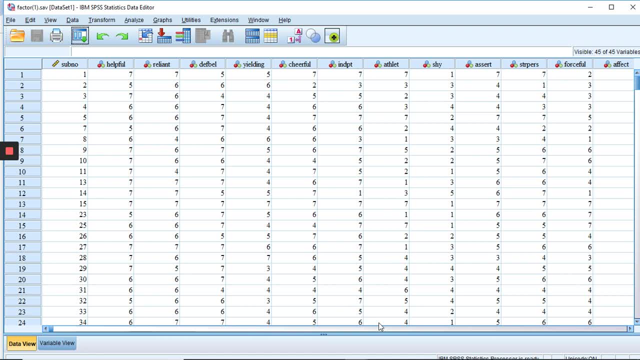 same data set that we have been looking at in the previous examples. It's looking at the BEM sex role inventory and in this factor analysis we're aiming to group 44 inventory items into larger categories called factors, And it's really helping define. 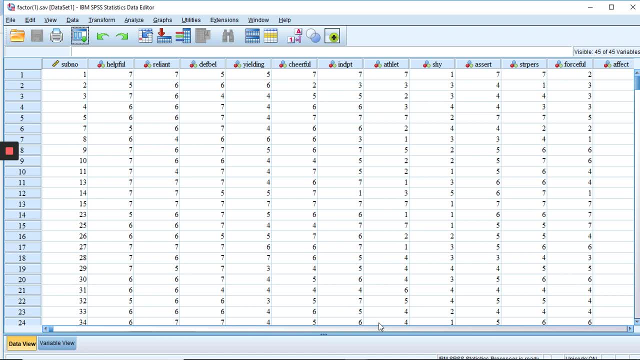 some constructs and seeing what this inventory might measure. Of course, one downside is that we can't change this inventory because we're not developing it. It's already published and has been in use, so it's not something we can manipulate as much as if we were creating. 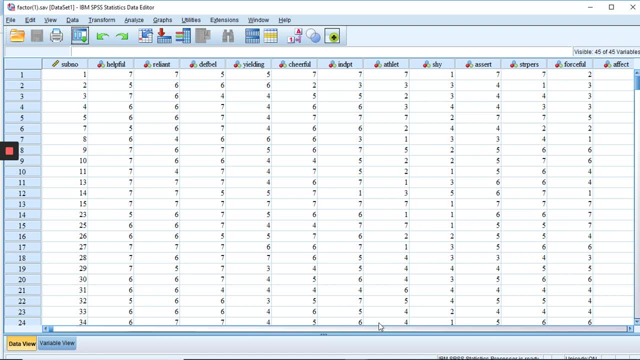 our own inventory, But we are in general looking for correlations and a factor analysis does require at least 300 for a sample size which we do have in this data set. So the research question is- and you can put this in your own words if you like, but the 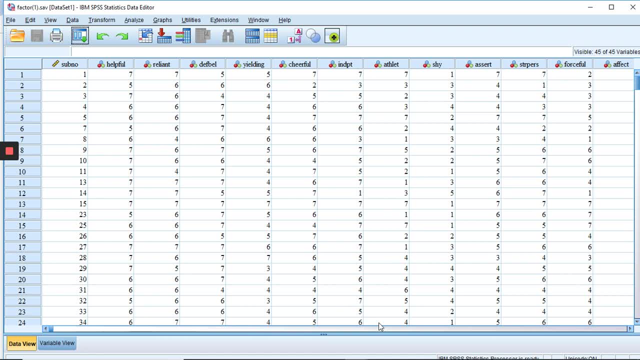 way that I phrased it was: can a set of factors be extracted from the 44 items on the BEM sex role inventory measuring masculinity, gender and gender identity? So this is a very simple question. You can put this in your own words if you like, but the way that I phrased it was: can a set of factors be extracted from the 44 items on the BEM sex role inventory measuring masculinity, gender and gender identity? 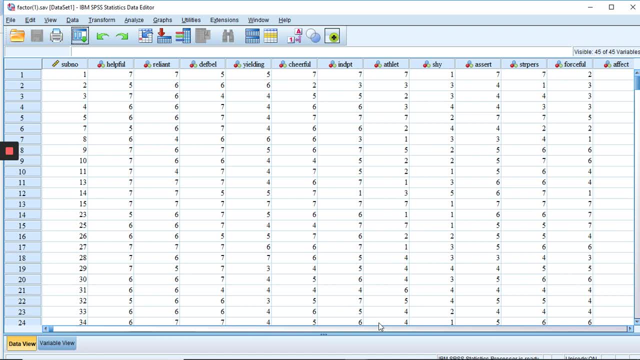 So the research question is: can a set of factors be extracted from the 44 items on the BEM sex role inventory, measuring masculinity, gender and gender identity? The answer is yes. Let's take a look at the number of women and, in general, what we're looking at here is 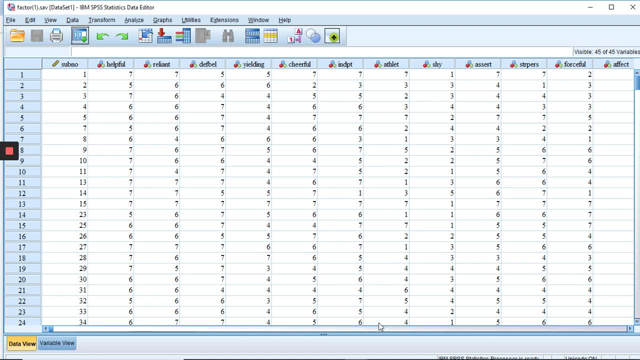 a number of women. so a sample of women and a number of women. Now this number will change. for you It's 369 women that we're starting with. My research question. when I wrote it up, said 344 women, because I deleted some outliers. 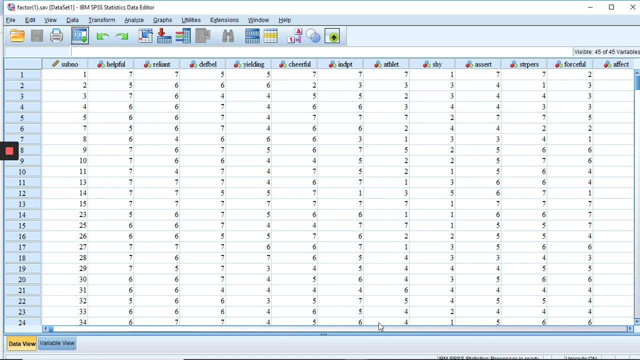 and we're going to cover that. So if you make the same decisions that I did, then you will also be writing a sample of 344 women. So first this, by saying that this chapter of the book uses SAS instead of SPSS, And so a lot of what they 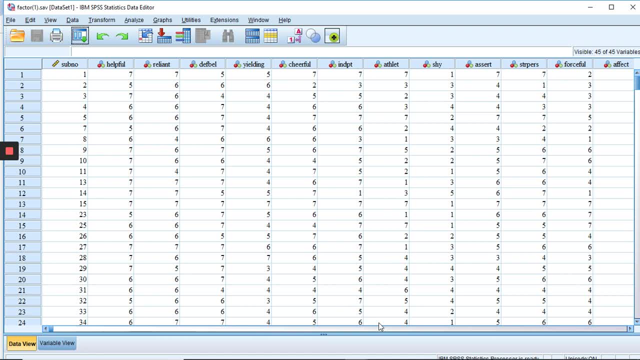 talk about and the way that their outputs are structured is totally different, And so you do have to ignore a lot of the book if you're using SPSS, as I am. But the evaluation of limitations is still the same, And we're going to be going through the checklist that is on page 670 in the 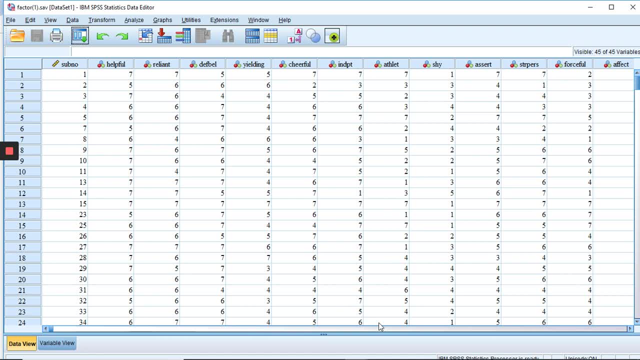 fifth edition, That's table 13.21, or in the sixth edition they may call that table 21.. And we're just going to go through the limitations as they're listed there, the major analyses, and then we'll talk about some of the additional analyses. 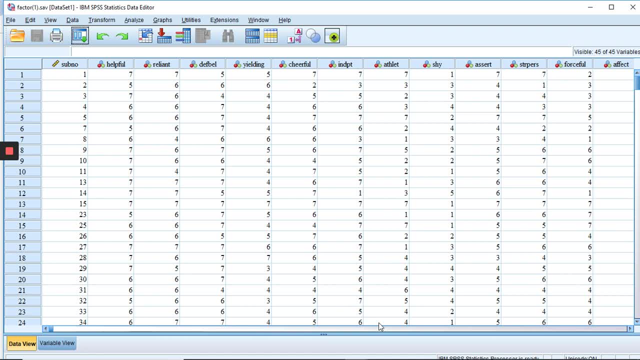 So first we want to look at outliers among cases. We're going to look at outlier variables later on, But first we just want to see if there's any cases that would be considered multivariate outliers, And so recall that finding multivariate outliers requires running a regression with 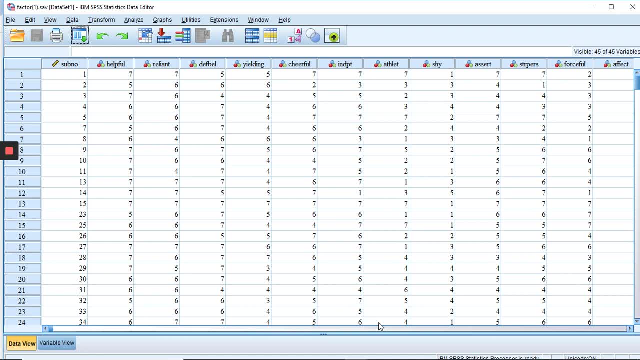 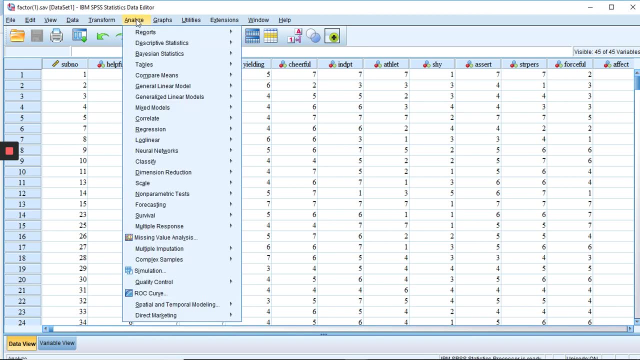 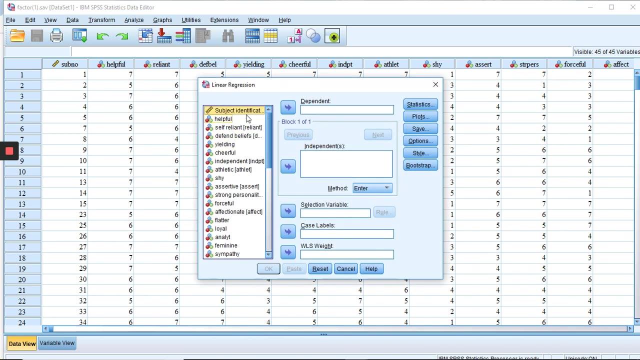 an insignificant variable, And so we're going to go ahead and click on analyze, regression and linear, And we're going to put subject number in the dependent And then, if you want to select all these at once, click the top one, go all the way down. 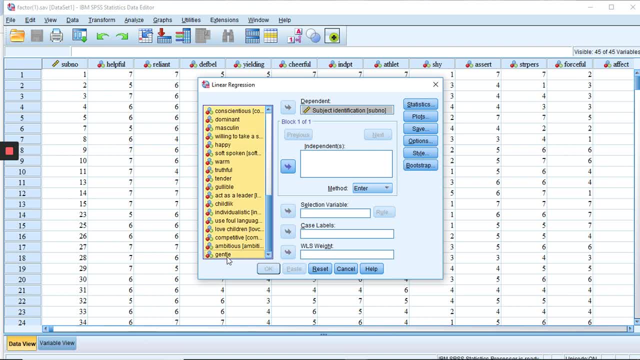 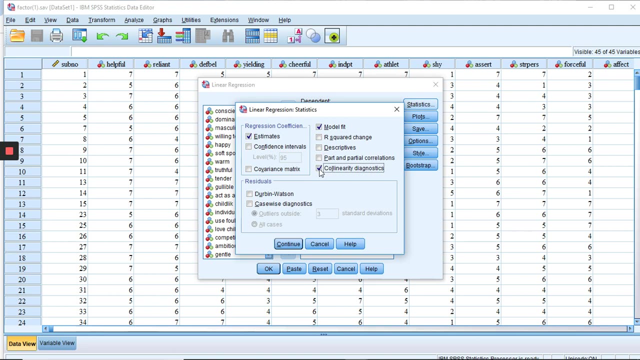 hold down shift, click the bottom one and then they all get selected and they all go into the independence. Now let me just see Which statistics we want here. We're going to want the collinearity diagnostics later, So go ahead and check that off. I think everything else. 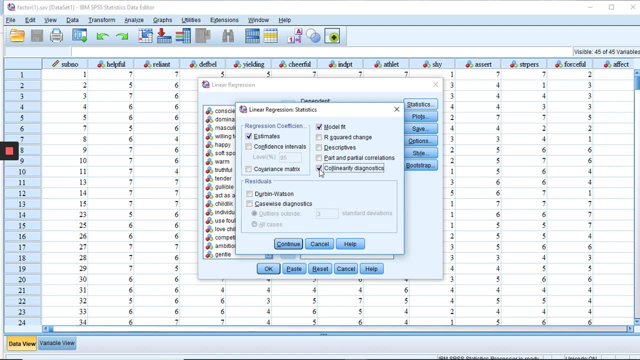 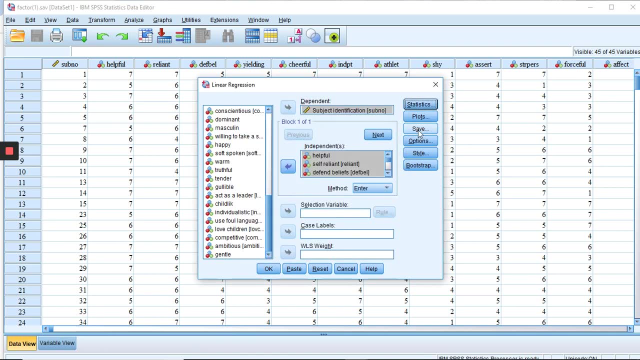 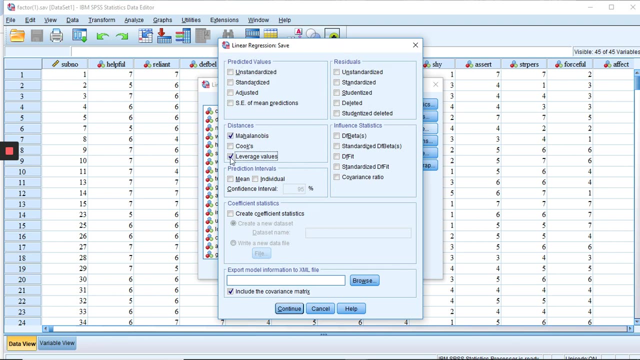 is about the same. I don't think we need to check off anything else. Oh, actually we are going to need to click on save. Good thing, I wrote notes And I wanted to save the Mahalanobis distance and the leverage values, So I 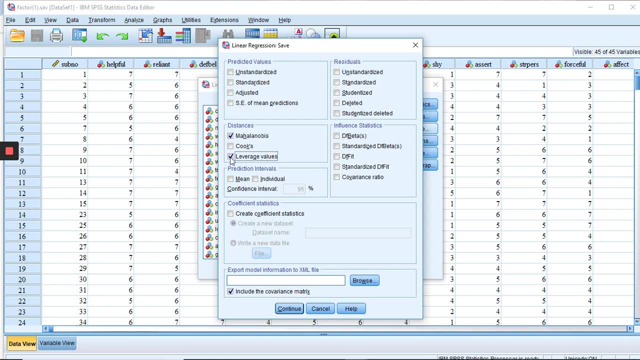 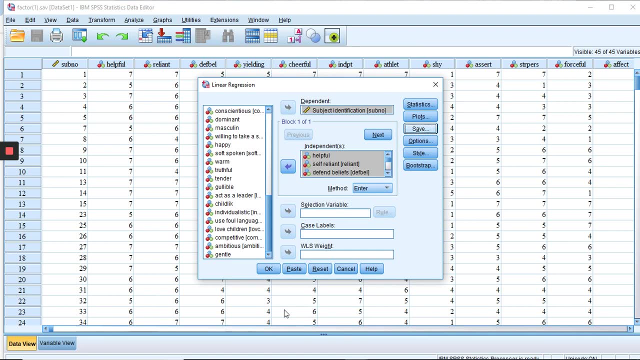 I kind of liked to look at both. They just talk about the leverage values in the book. All right, So click continue. Let me just make sure I'm not forgetting anything else. That's it Okay. So we can go ahead and click Okay. 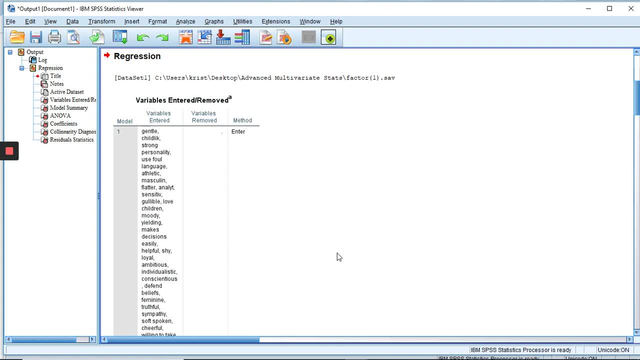 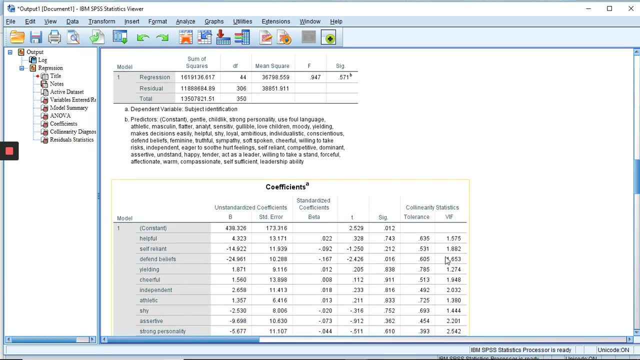 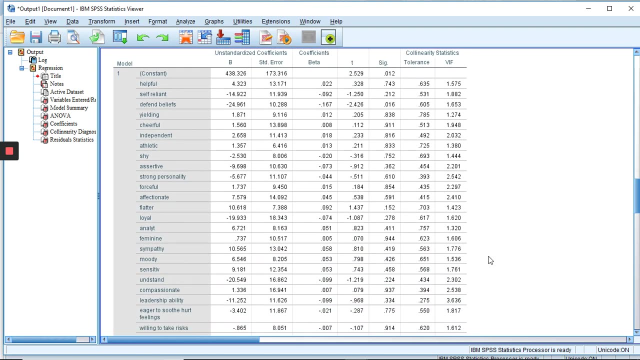 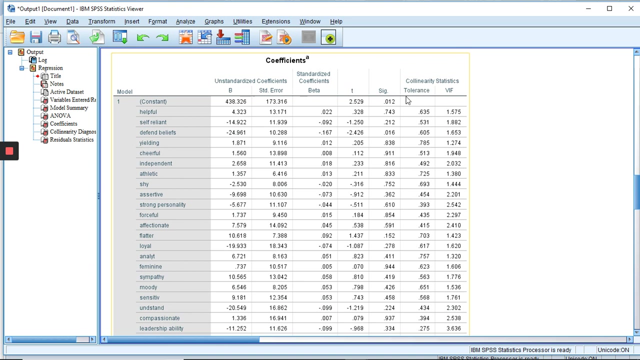 And here we have our regression output and what we are looking for. Okay, Okay, Okay, Okay, Okay. This is really actually not in the output, So we'll go back to our dataset. I'm going to point this out, though, while we're here, where it says collinearity statistics- tolerance. 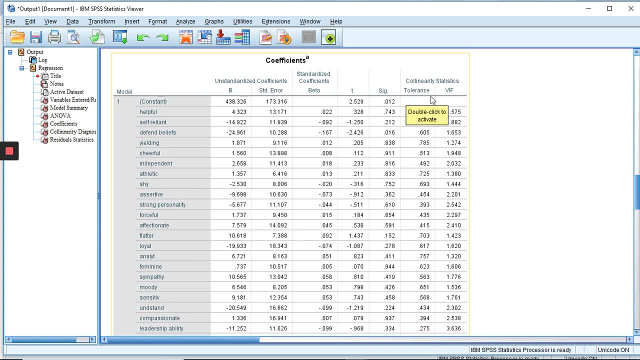 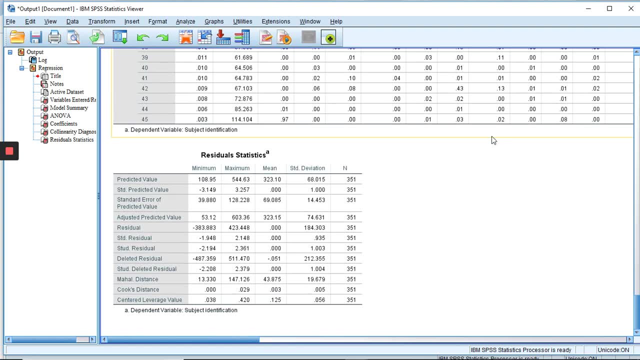 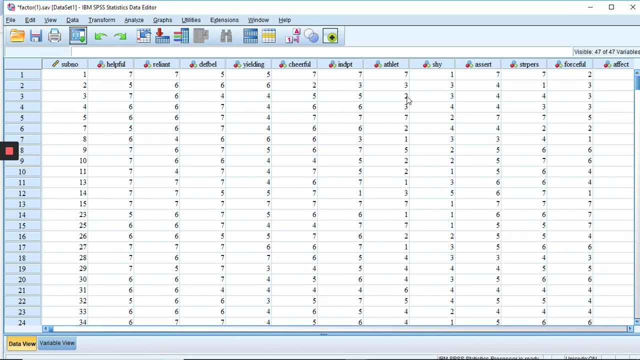 We're going to come back to that later, when we were looking for outliers of variables. So we'll come back to that, but actually I don't think we really need any of this output, So we can minimize that. what we really want to look at now. 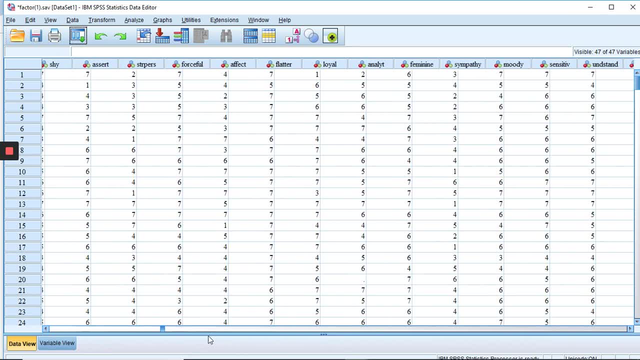 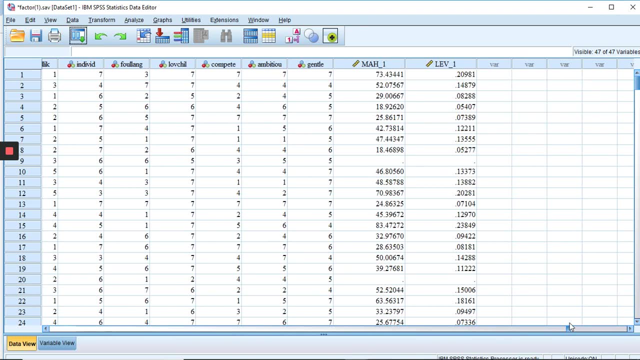 is our data, because we saved the Mahalanobis distance and the leverage. So there they are. You can see that they are calculated here, And what we want to do is sort by descending. That way, the biggest values are at the top. 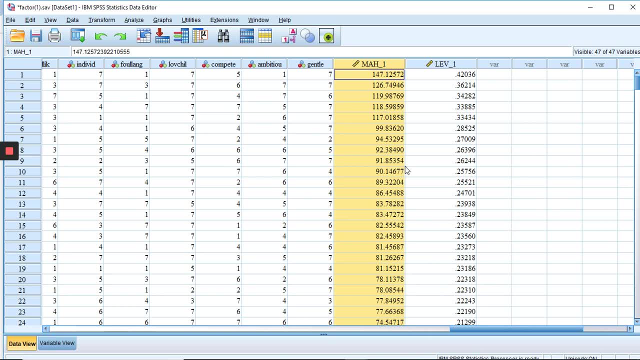 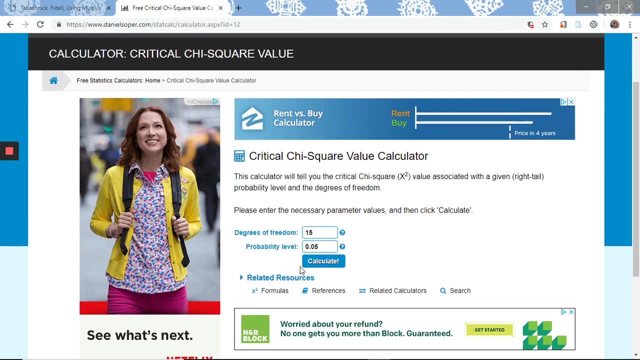 And now what we need to do is, well, click save, because we just added two new variables, So save that. What we need to do is go to our chi-square critical value calculator, And this is on danielsopercom, And there's 44 degrees of freedom. 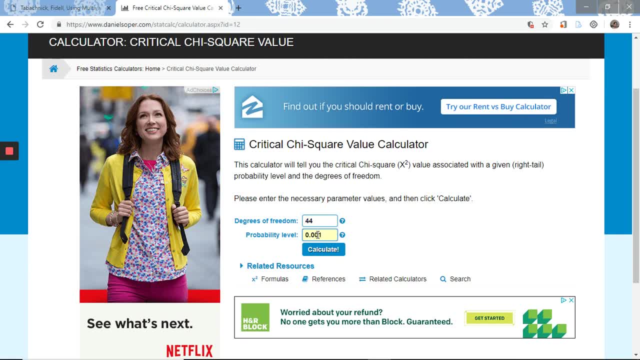 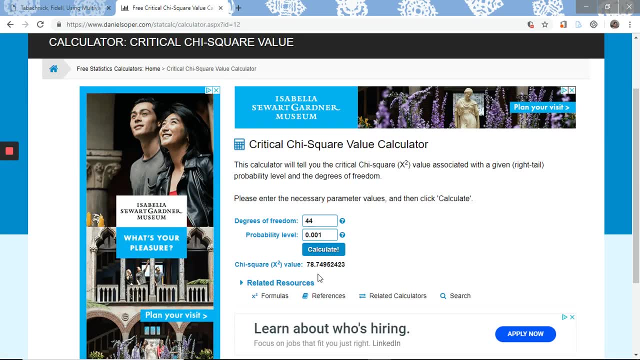 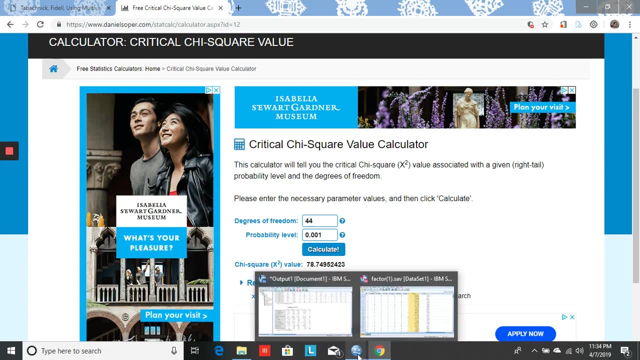 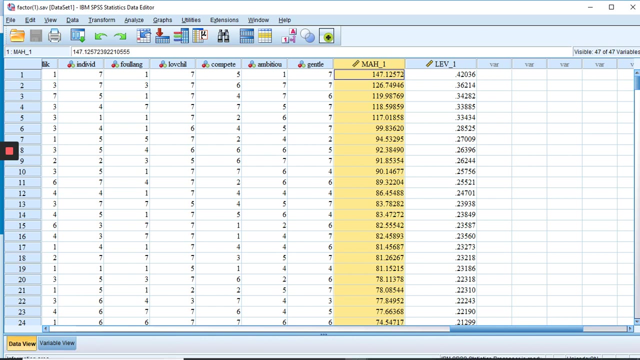 And we're using point 001, as they did in the book for the alpha level, And we hit, click, calculate And we get seventy eight point seven, five, rounding, which is what they had in the book as well, And so we'll go back to this, And so our critical Mahalanobis distance value is what we just said, which let me look at again. 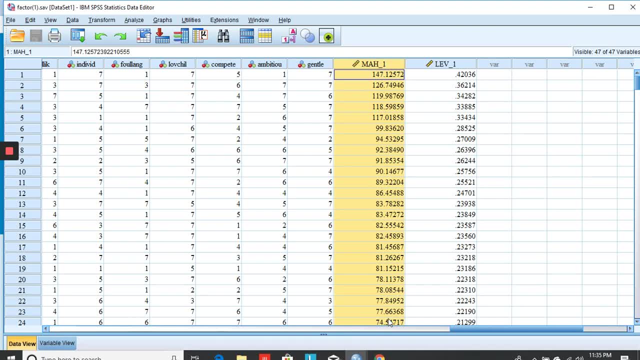 Seventy eight point seven five. So anything above seventy eight point seven five could be considered an outlier. So here you see, on case nineteen, right here there are nineteen cases that are above that number. So that's kind of our first indicator, But the leverage statistic is a little bit more accurate. 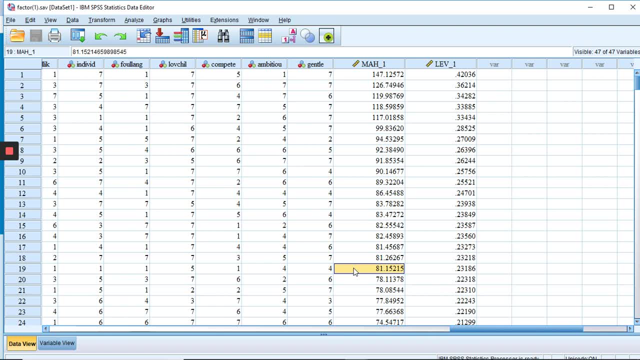 And in order to get that, you have to follow an equation that they have in the book, And what you do is you take that Mahalanobis distance critical value, which was seventy eight point seven five, Divide that by the total number of cases minus one. 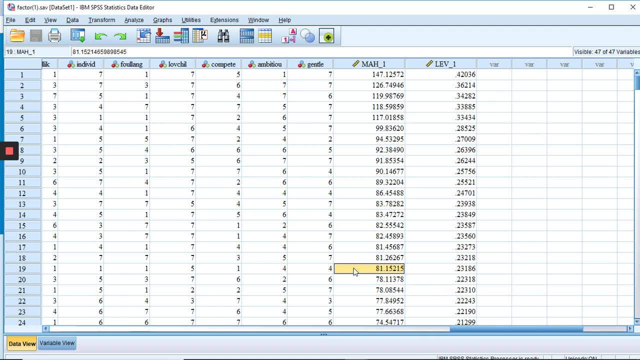 So that would be three, sixty nine minus one or three hundred and sixty eight, So seventy eight point seven, five divided by three, sixty eight Plus one over three sixty nine. So if you calculate that it equals point two, one, six, seven, which is the critical leverage value. 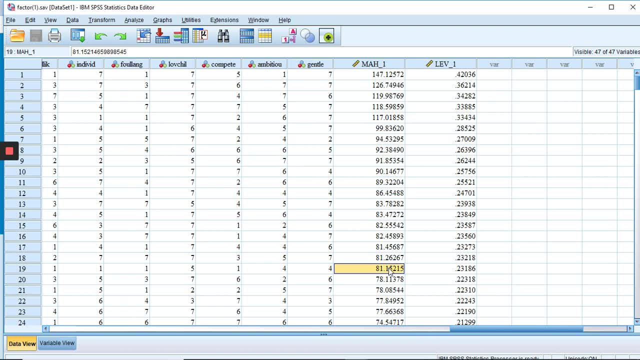 And so we're looking for anything above point two, one, six, seven, which, if we scroll down here, you can see that this is point two, one, two. So right here is where we have a critical value. Let's scoot on over and you can see that that is twenty three cases. 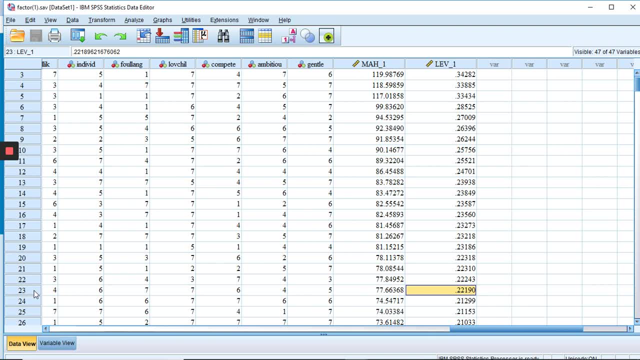 The book says twenty five at this point, And again I don't know if that's a difference between how the SAS is calculating the leverage values or what, But I never did figure that out. But twenty three cases right here. So what we're actually going to do is rerun the regression. 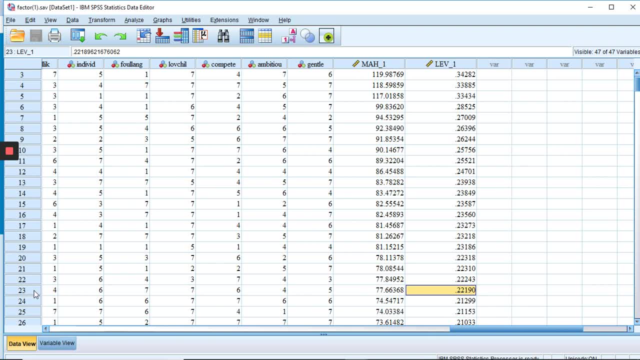 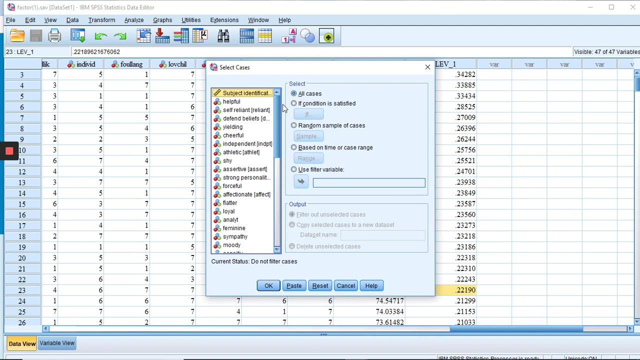 But we're going to first move, take these cases out, but we don't want to delete them yet because we're still trying to decide what to do with the outliers. So what we're going to do is go data Select cases If the condition is satisfied. now it's going to. selecting means it's going to use those ones. 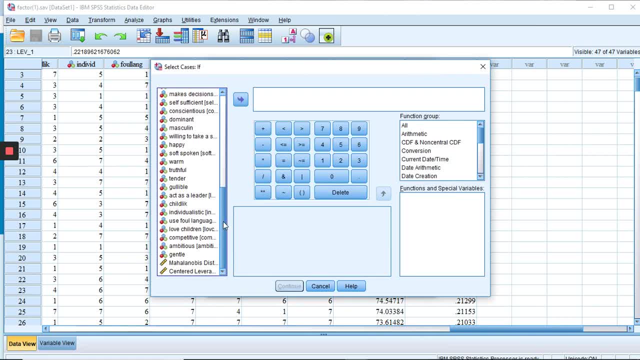 So we actually want the leverage value down here To be less than our critical value, because that's all the ones it's going to keep. So it was less than point two, one, six, seven. That should cross out twenty three cases where the value is above that. 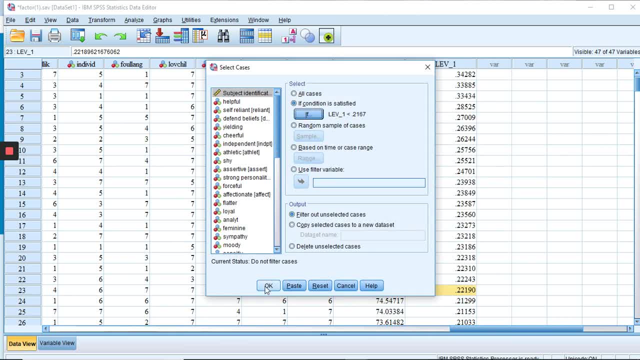 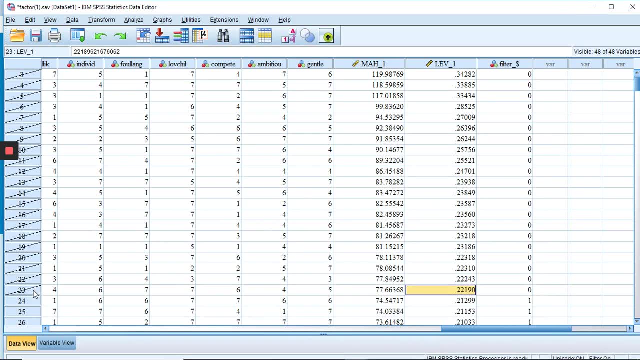 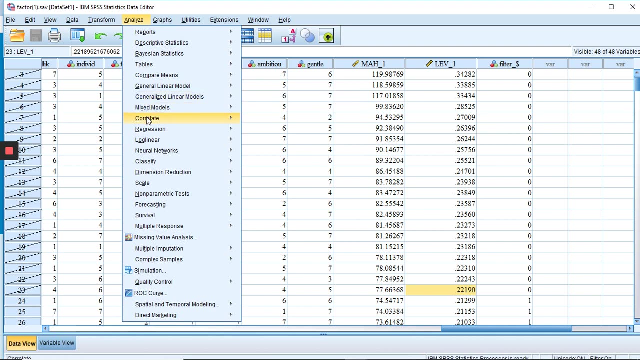 So let's make sure that that happens. Click OK, Minimize that. And here we have yep, twenty three cases that have been crossed out. So let's save that for a minute And run that regression again. Analyze regression linear. 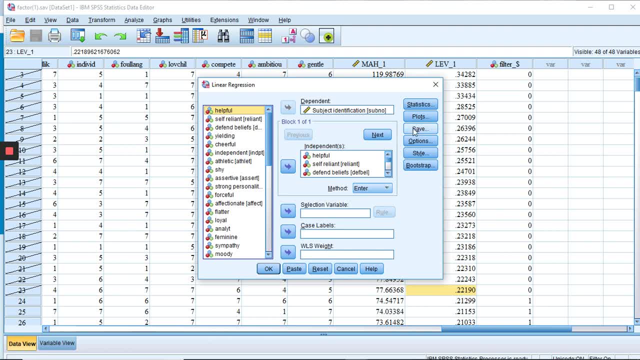 Now we do still want all our options to be the same, Although I think when we look at the collinearity diagnostics, do we need them for the full set? Yeah, So you could just not get the collinearity diagnostics This time? sorry, because then you'll have two that you're looking at your output. 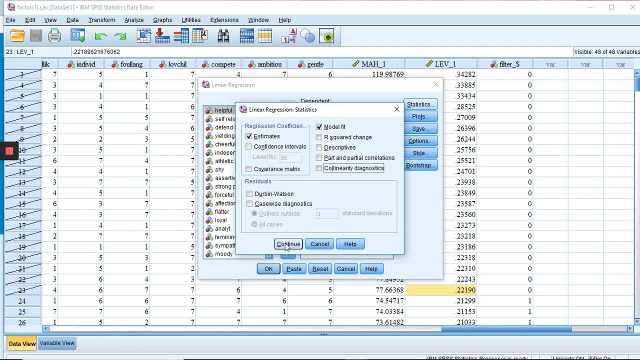 And that might be confusing. I guess I would look at the first one. That's a question I would have to think about. It might be better to rerun it after we've deleted all the outliers, So we may just do that again. But I'm not sure I did that when I did mine. 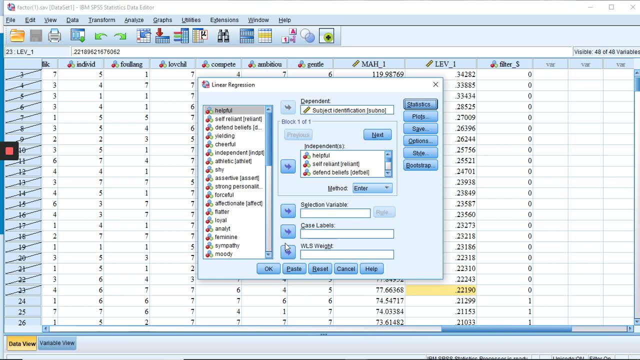 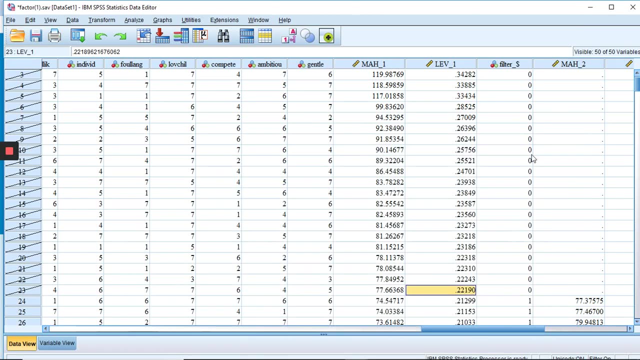 Either way right now. Now what we're looking for is kind of a recalculation of leverage values, with those cases removed, Just to see and recalculate a critical value. So I'm going to click OK And again we're just going to look at our data set here. 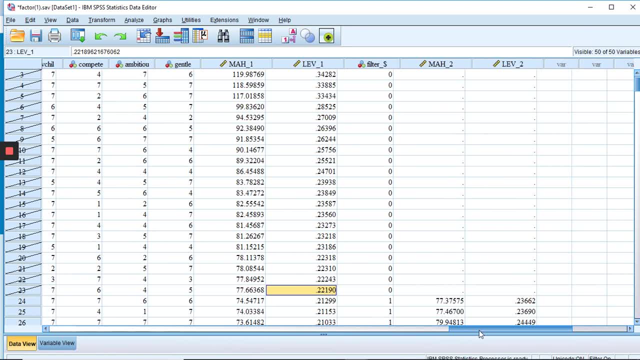 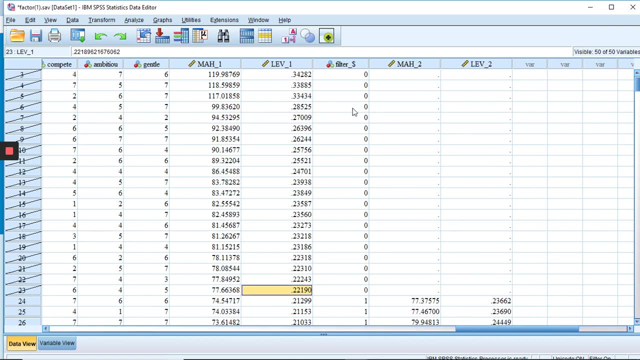 Now we have Mahalanob, assistance two and leverage two, And so here's our new values. And Oh, I just realized something sort descending. Maybe I didn't sort it right before, No, I did. OK, Just a thought. I still can't figure out how the book got 25 the first time. 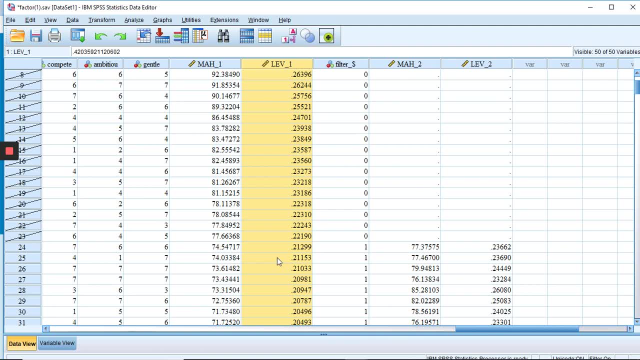 So I thought maybe I made an error. but nope, I don't know how they did that. OK, so now what we're going to do is we're calculating a different critical value And the book, on page 653.. Describes the London board London board criterion, which their calculation is to open, with open parentheses, K over N. 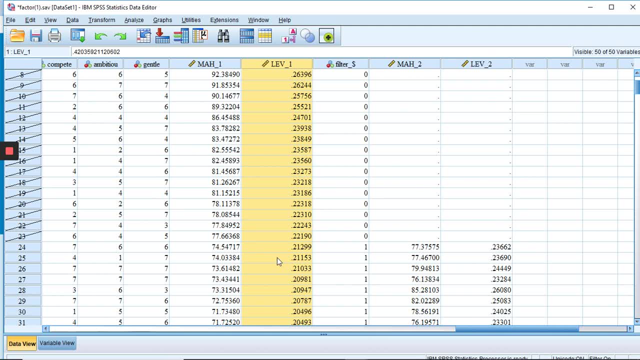 That's their formula, Close parentheses- And so I honestly don't know what K is. But what I did was I used the book's values around this to calculate for K And then used K in in my own. So in this case I'm eliminating 23 of the cases. 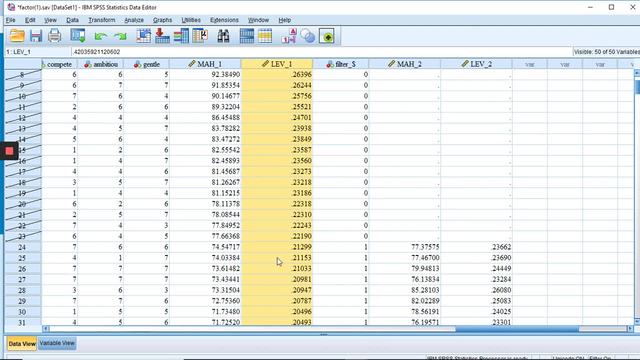 And so the new N right now is 346.. And I will just tell you that if you solve for K in their equation, then using their values, K equals forty three point nine, nine, seven, six, And so Plugging that into the formula. 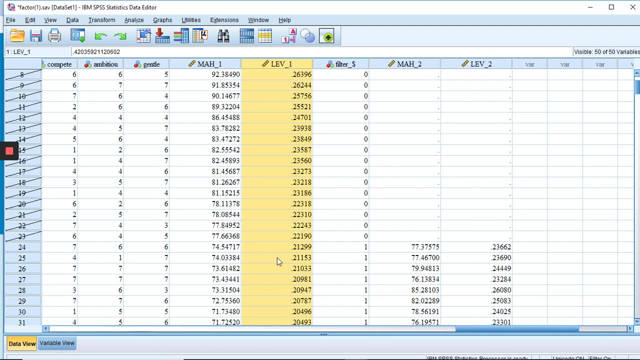 Two times open parentheses: Forty three point nine, nine, seven, six Divided by three hundred and forty six Equals point two, five, four, three. So now, in our new assessment, Which we're trying to be conservative, We are looking for leverage values. 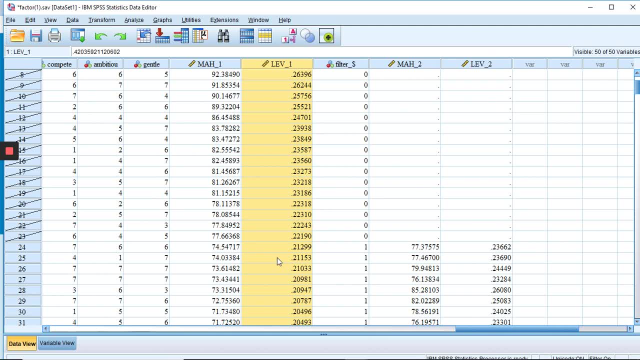 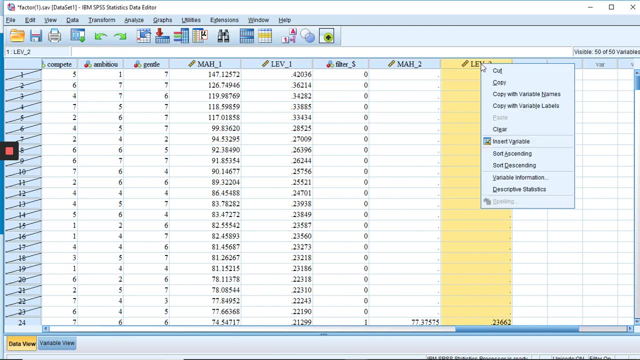 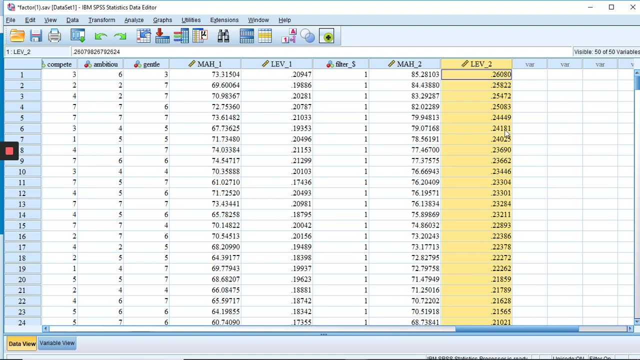 That are above point two, five, Seven, four, three. point two, five, four, three. And so let's sort the leverage By descending. It's going to shoot all those empty ones down to the bottom, And here we can see which ones are above. 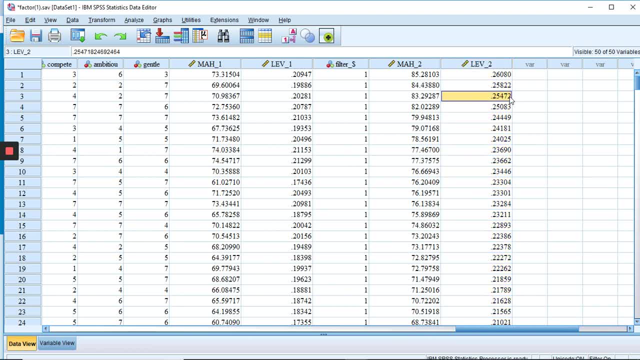 Point two, five, four, three, And right here you see, that's the cutoff, That's the threshold. right there There's three additional cases That exceed that number, And so I also Chose to delete those cases. So When we don't delete yet, 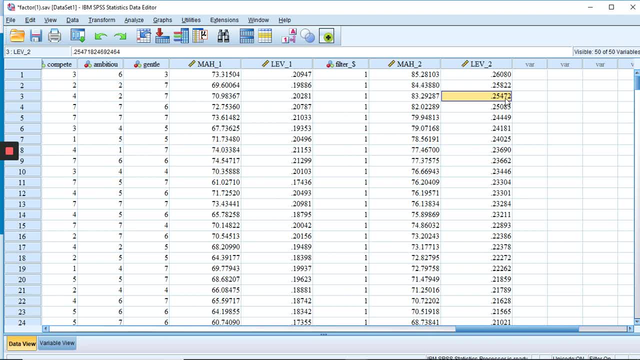 Because we need them still. But basically we're going to do one more test, using a discriminant analysis, to determine if we should really delete them. But these three cases plus the twenty three others Is what I did end up deleting- is twenty six cases. 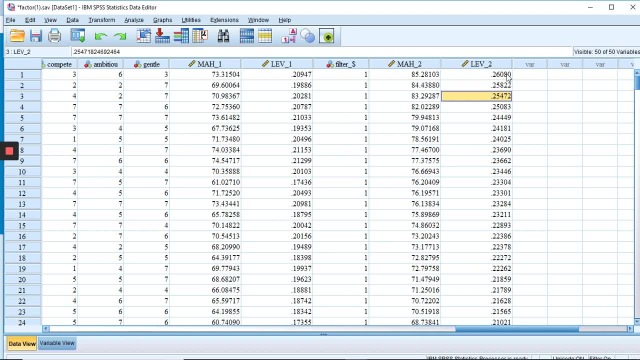 So what we're going to do Is create a new variable, Essentially a dummy outlier Variable, where the outliers are labeled with a one And the non outliers are labeled with a zero. So, if we go to Data or no, transform compute variable. 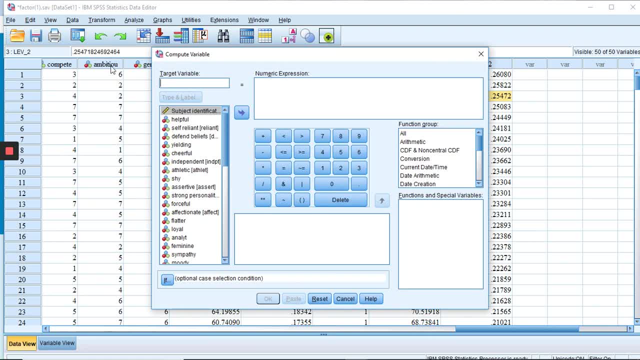 And you can put in Your target variable ID. And you can put in Your target variable ID, Your target variable. I call it Dummy Variable, Or what did I do, Dummy outlier? That's what I called it before. 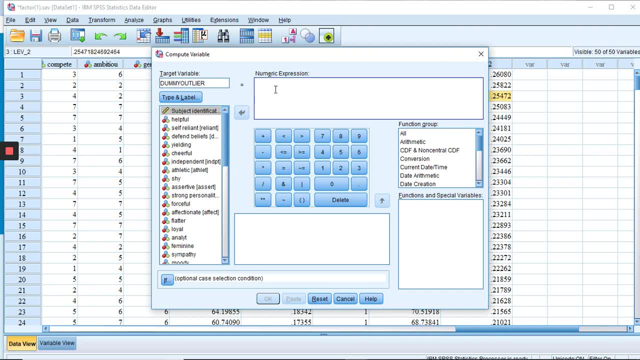 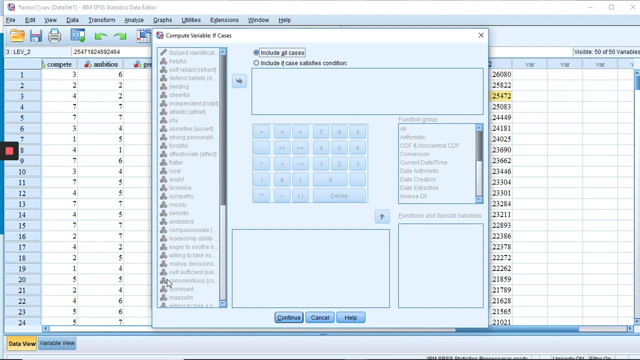 Dummy outlier. Now here's your numeric expression. You want- Let's see If Case satisfies the condition. And you want Two things. One is leverage one right here. Put that in If that is greater than 0.2167,. oh, hold on a second. 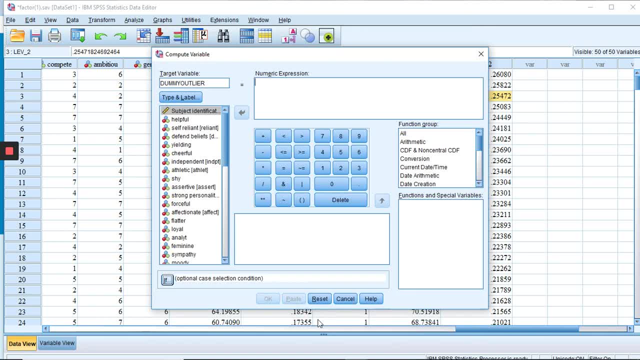 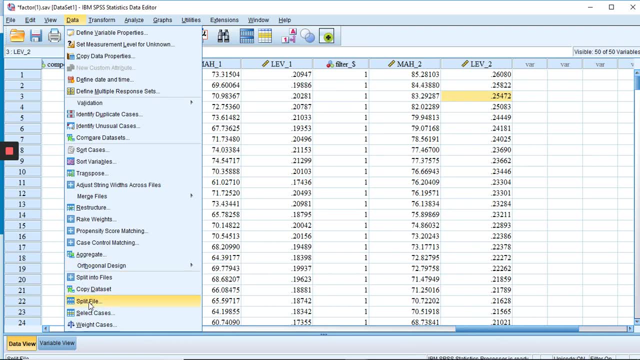 Cancel this. We have to turn off that split file on the data first, or it's not going to include all of them, Okay, so hold on. So data split file. we need all of our cases for this. Oh, analyze all cases. 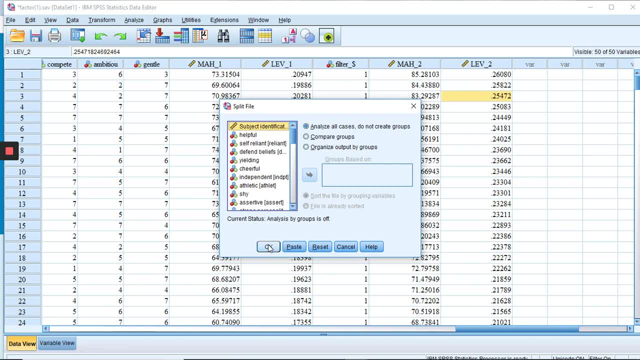 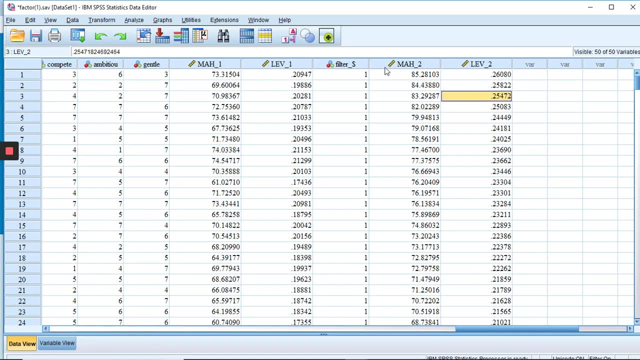 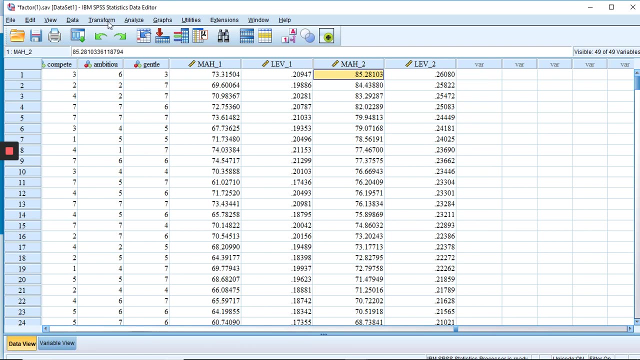 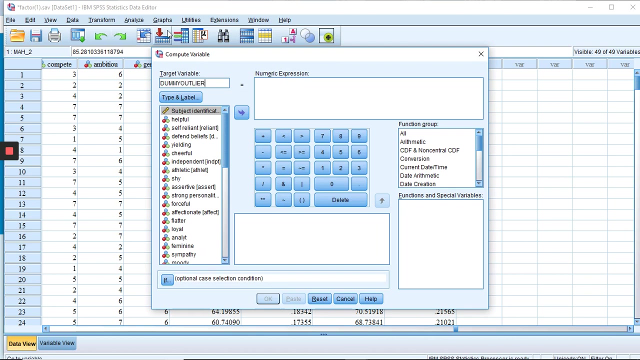 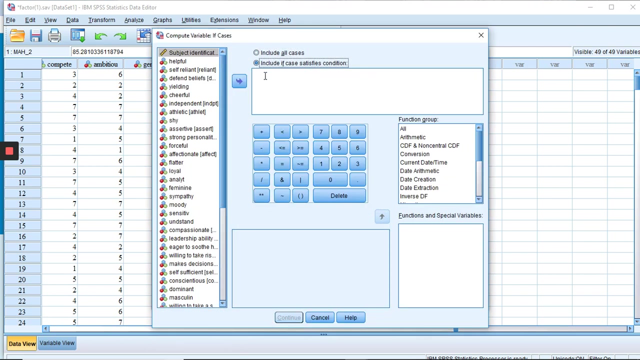 Did I take that off somehow? Okay, I don't know how that happened, because this filter is still on. I'm just going to delete this just in case. Okay, that should work. Sorry guys. So transform: compute variable dummy Outlier. and that's going to be if include case: if the first leverage value is greater than 0.2167. 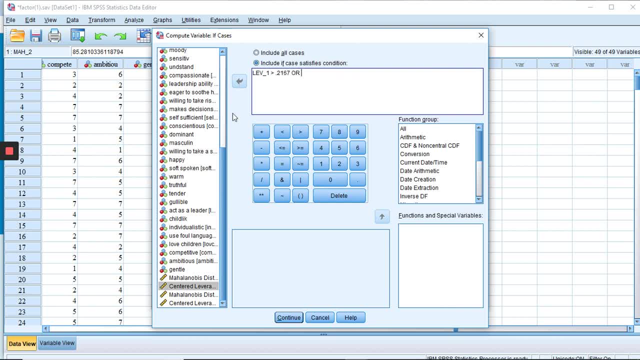 or the second leverage value is Okay, greater than 0.2543.. We say the or because we don't want them. If we said- and then it would look only for ones- that was true in both and that would throw it off. 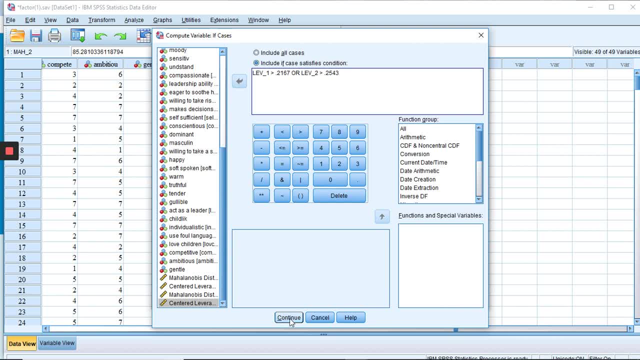 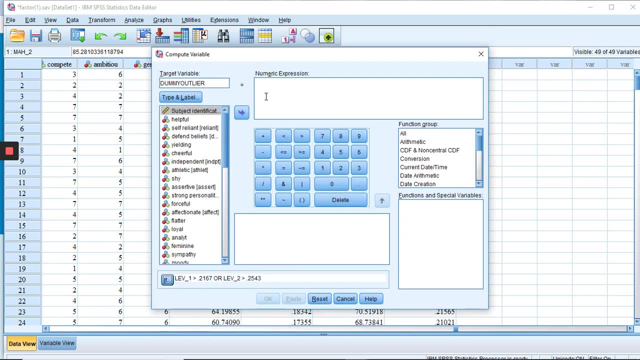 But we want one or the other, and that should give us 26 cases that they put in a one, And so we click continue and then that will equal a one. So if this is true down here, Okay, Okay, Okay. 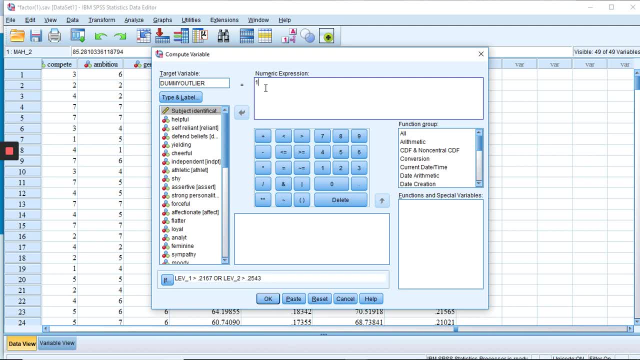 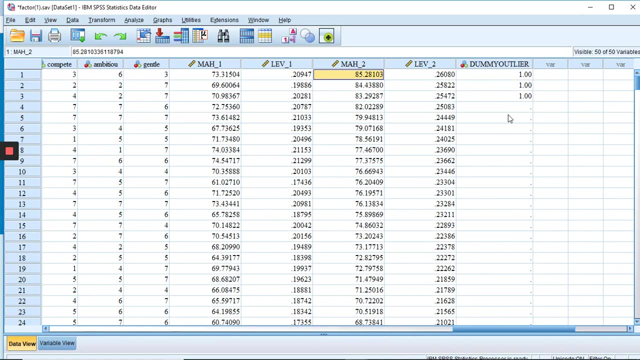 Okay, our if. for us then it's going to equal a one and the non outlier group will be zero. right now it'll be missing, so we will have to turn those into zeros in a minute, but click OK and then close that output and here you have let's, let's. 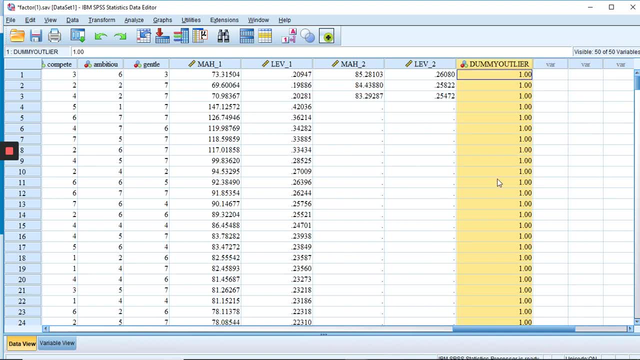 sort these descending. let's just make sure we have 26 cases, and yes, we do so. that was correct. our formula worked. here we have 26 cases that are labeled and now we need these to be zeros. so we're going to go ahead and transform and recode into the same variables. we're going to go down and choose our dummy. 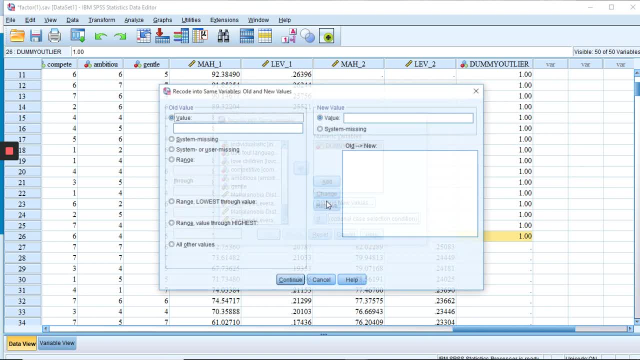 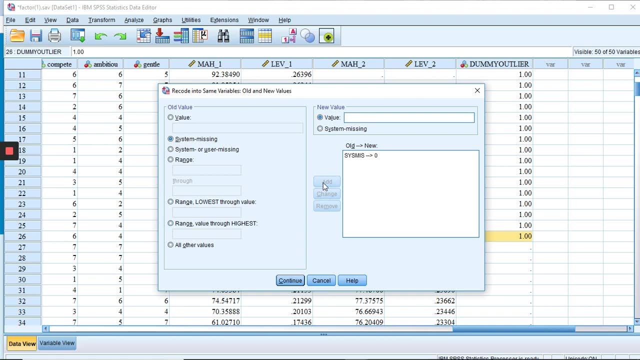 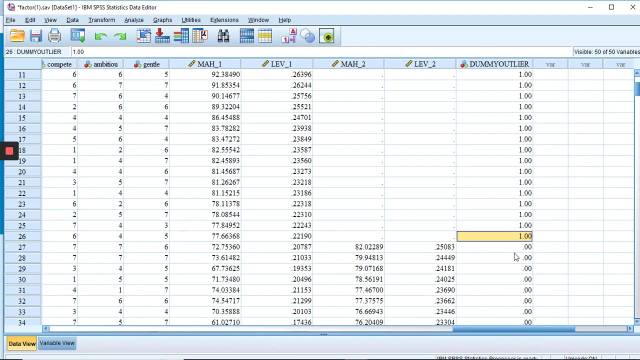 outlier and we want to replace the missing ones with a zero. add that in and continue. okay, you now going to our data set. yep, we've got zeros. for the rest of them, super. so now we're going to run a stepwise discriminant analysis. let's just save so. 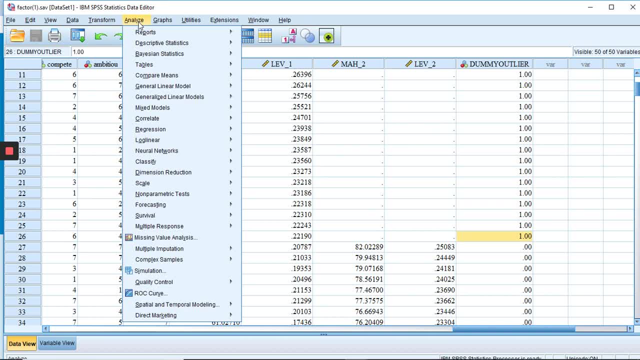 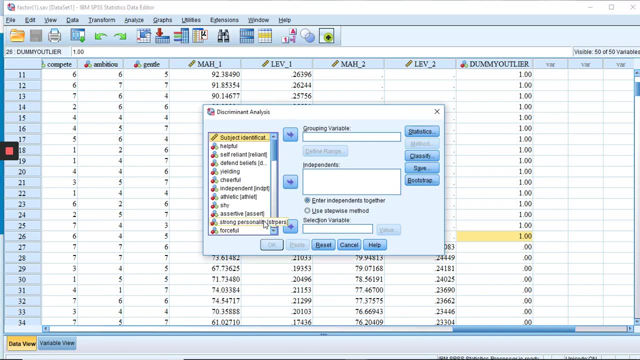 we have all this. so analyze, classify, discriminant, and the dummy outlier variable is the grouping variable and the range is obvious and we're going to run a stepwise discriminant analysis. let's just making sure that we're resetting everything from the planner, and can you? 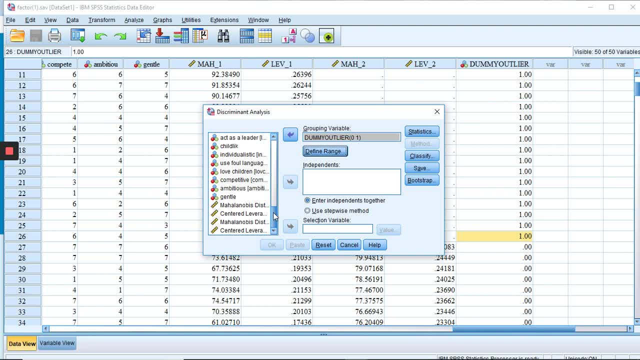 see, because the numerical families are pulled from way back up so it needs to be everywhere. so let's say, as my holding panel and I go through all the variables, you can see this one down there and now it says independent, there is not. and I're going to run this, so let's see if it works. okay, we got two. 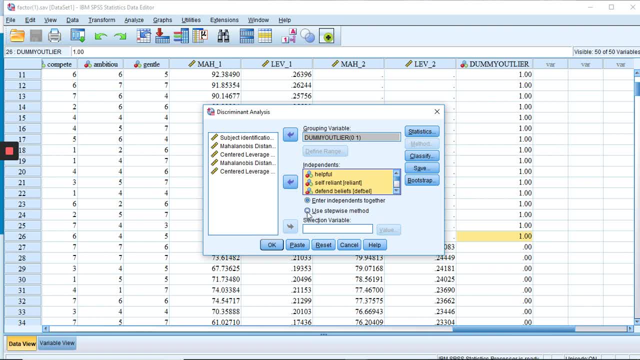 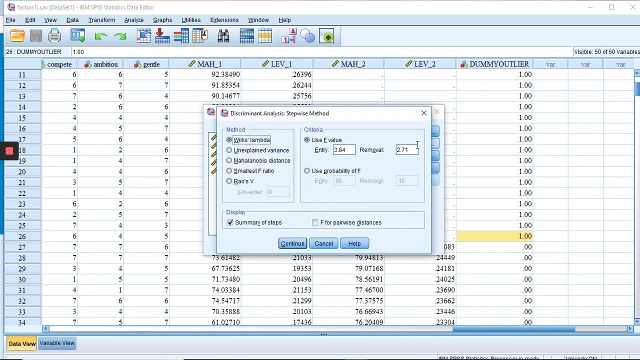 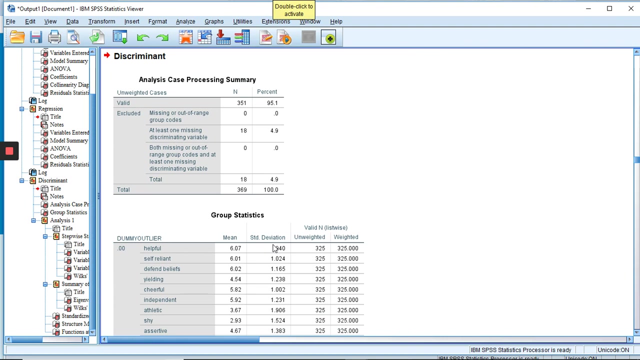 values that we have here, obviously zero or one. that's what we've got: two values and independence, our all the variables, except like all this inventory variables, to use a stepwise method and statistics. we want the means, and let me see method. okay, that should be everything we need, so click OK. and now what we're looking. 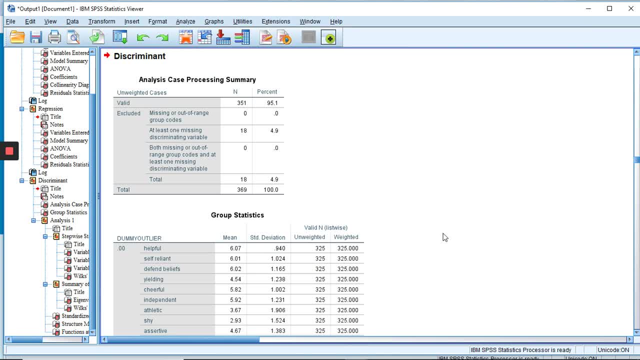 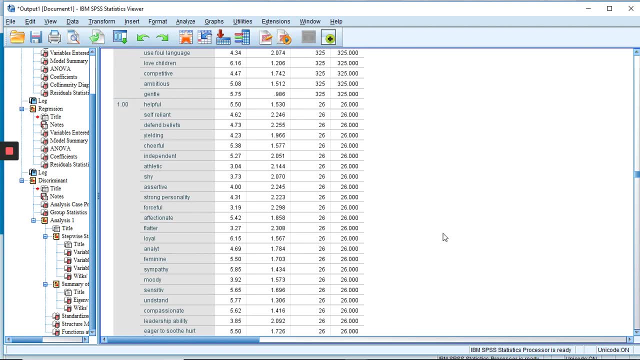 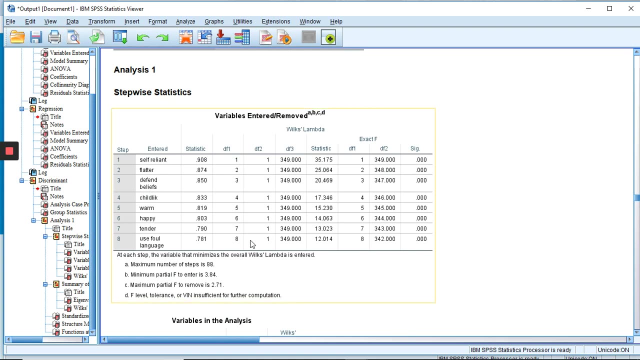 for is trying to see these. this gives us all of the means, so scroll down on your output and right here is what we want to look at. this variables entered, removed, and there's all these different steps, and so it shows the order of these. now they're all significant here, so I was a little 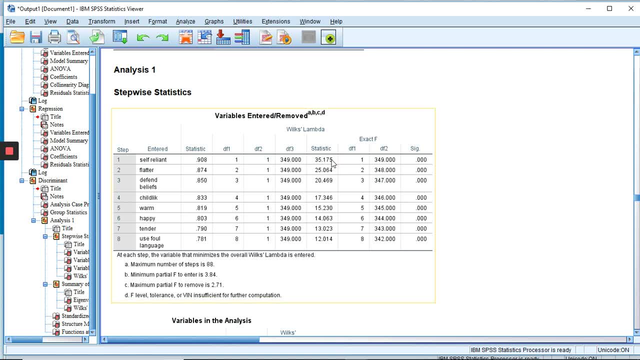 confused at this point, but you can see from this statistic here that 35 and 25 are fairly high values and they're, you know, they kind of stand out from the rest, and those were the two variables that the book referenced as well: self-reliant and 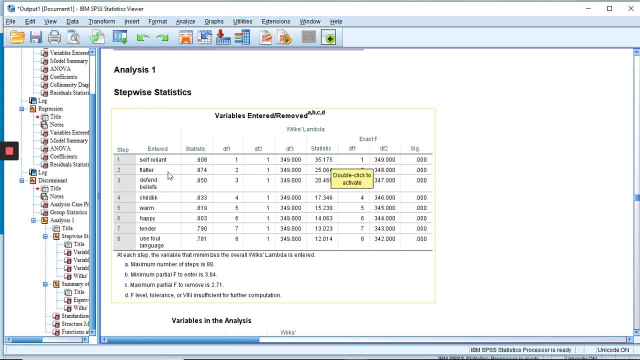 flattery or flatter, I don't know. flattery, I guess, and so basically what this shows is that there's a lot of things that we want to look at here and really need a comparison for each group appreciation. so our first step of today's lesson was to tweak these things a little bit for each group we mean. 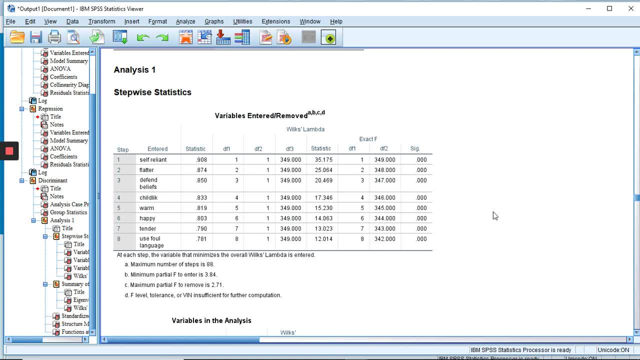 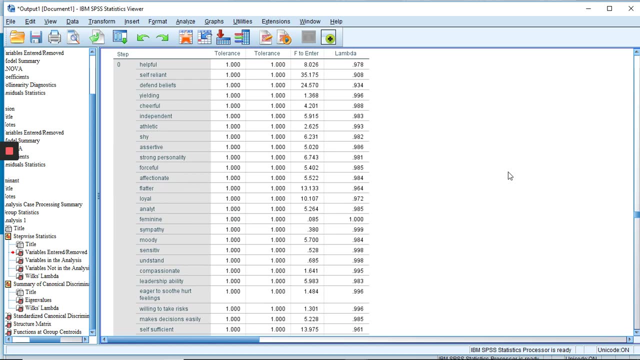 We're showing those based on these two groups and also some of the definitions of those other groups. if we were to think of it with this reason, we took the model as sort of a super-digital model of. we're emphasising here to make a moreester-friendly or sort of uni-detjamineer relationship which can solve anything we want, and so I'll show this problem and where to use this protein and how to use it. 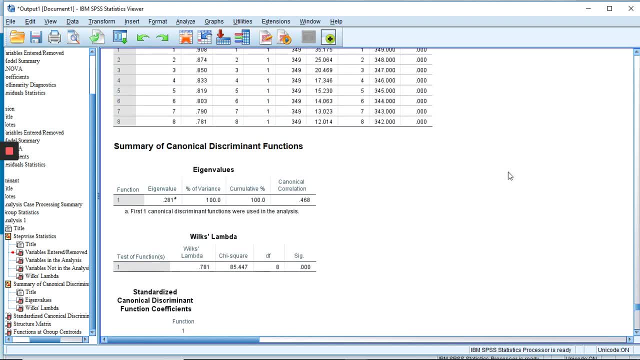 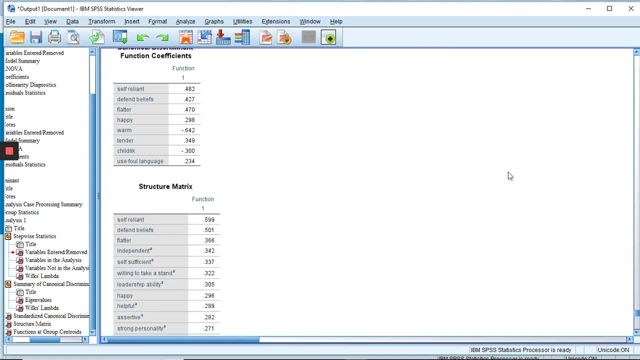 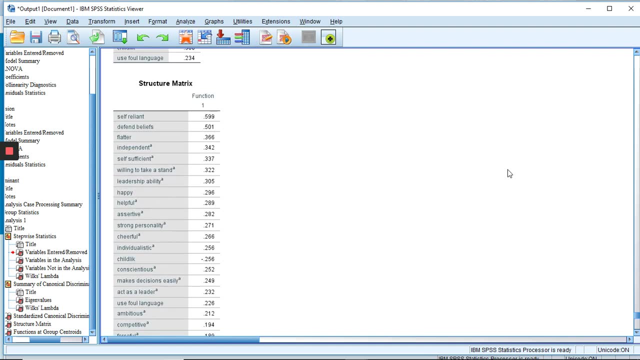 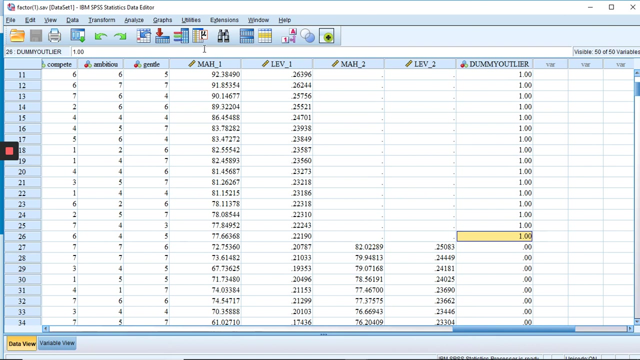 anything down in the rest of this output. Yeah, So I mean, it looks for the variables that are the most problematic between those two groups. So one thing that I did was I also was just thinking: okay, when you're comparing groups, what do you do? Well, maybe an ANOVA. it compares. 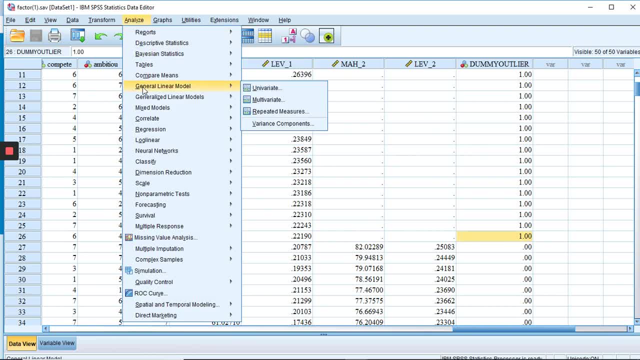 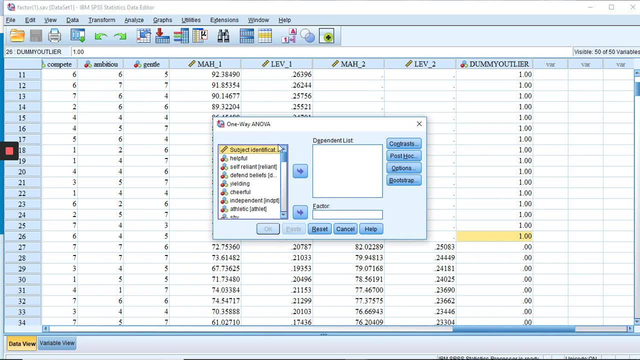 things. So I just went ahead and did a where is it? Compare means one way, ANOVA too, And I think I just selected all the variables that are on the inventory, And then I use the dummy outlier as the factor And let me see if I clicked anything. No, 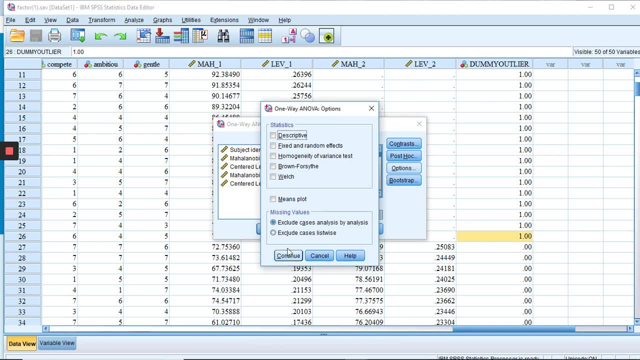 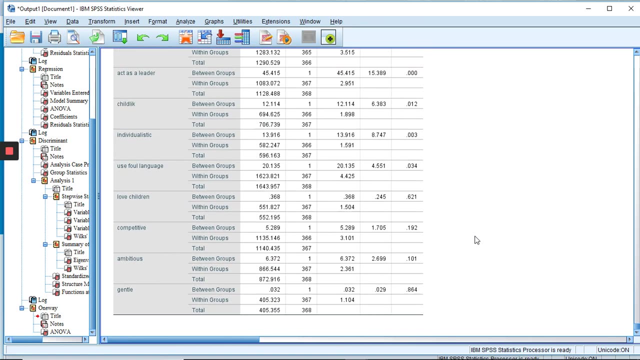 I don't think I did. I don't know if you could do a means plot, but that might give you like a thousand different. I'm not sure what it would give you. So just click, okay, And I think what I was looking for here. let me see. 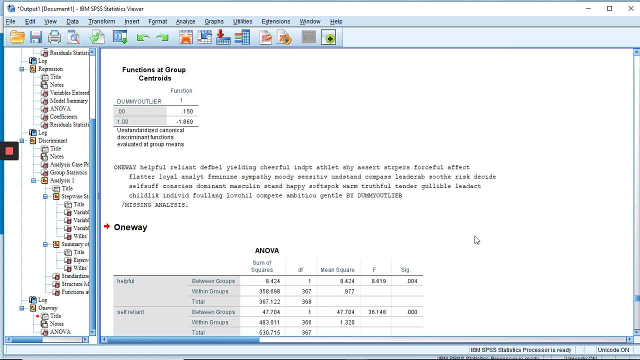 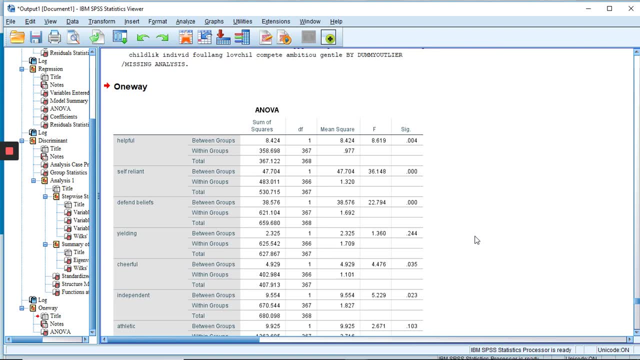 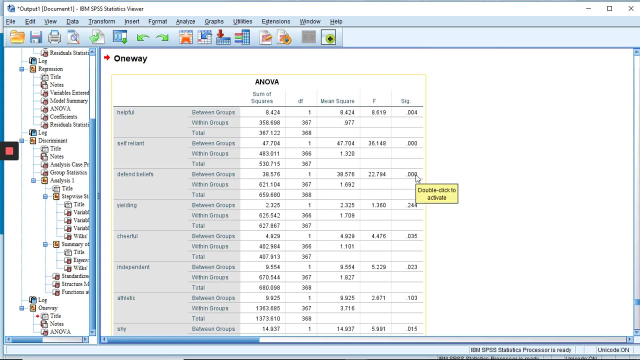 Hmm, Hm, Hmm, Hmm, Hmm, Hm off something else when I did it last time. but I mean, just look at how many of these are significant. right, It shows that there are significant differences between the groups. 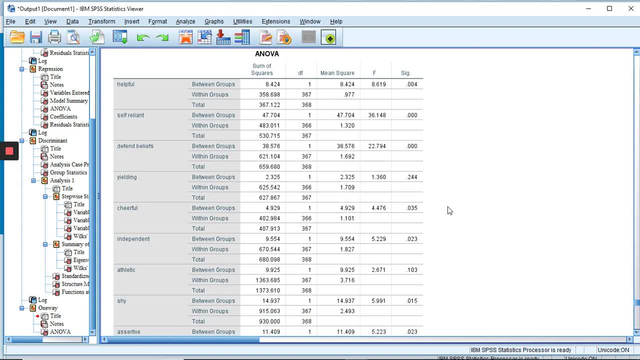 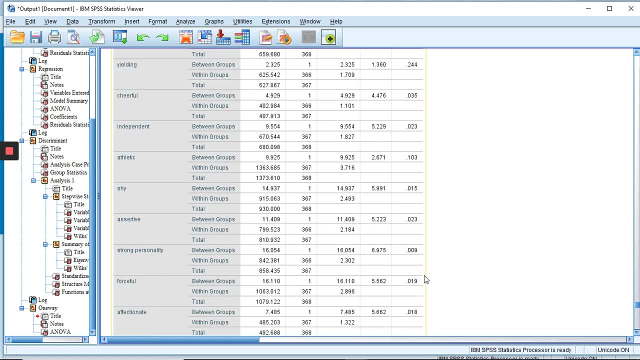 So we've got 44 variables here and we've got 1,, 2,, 3,, 4,, 5,, 6, 7,, 8,, 9,, 10,, 11,, 12,, 13,. 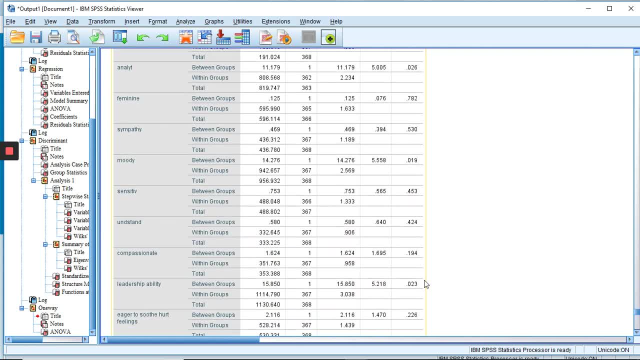 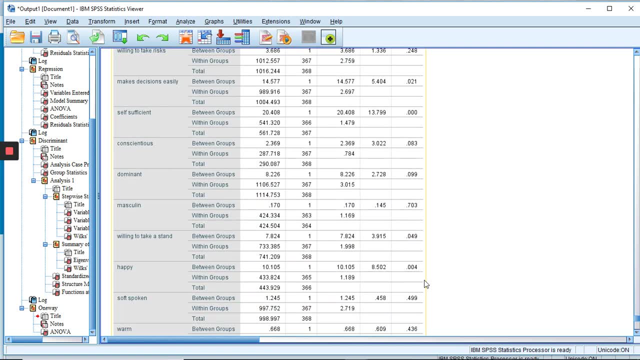 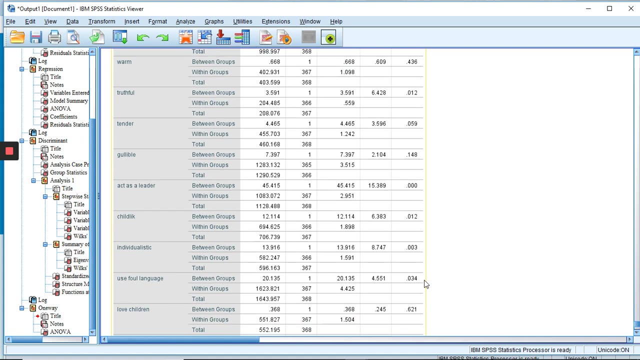 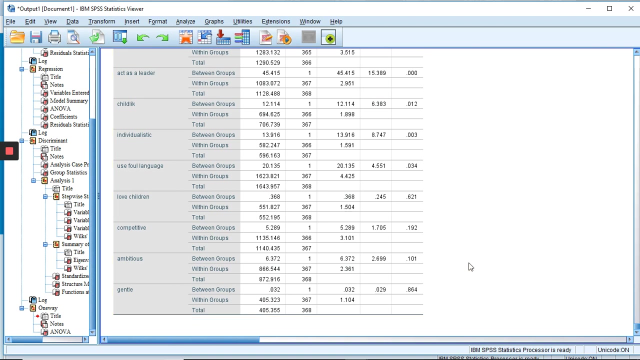 14,, 15,, 16,, 17,, 18,, 19,, 20,, 21,, 22,, 23, 24.. 24 variables for which the outliers as a group were different, significantly different At the 0.05 level, from the grouped non-outliers. So I don't know if that's a right way to do it. 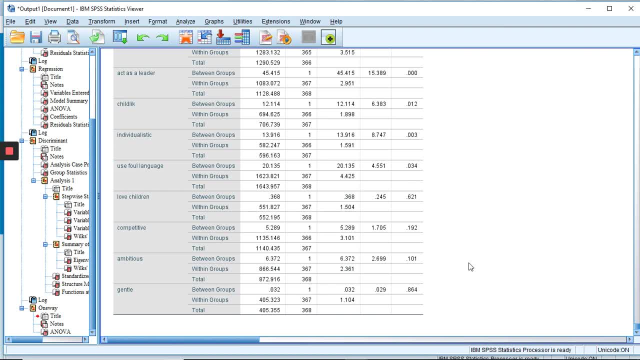 but it made sense in my head, and maybe it makes sense to you, or maybe it doesn't, And you can leave a comment and say: Kristen, you're totally off your rocker here. But as far as I was concerned, it was enough to establish that these two groups are different, and on enough variables that I feel. 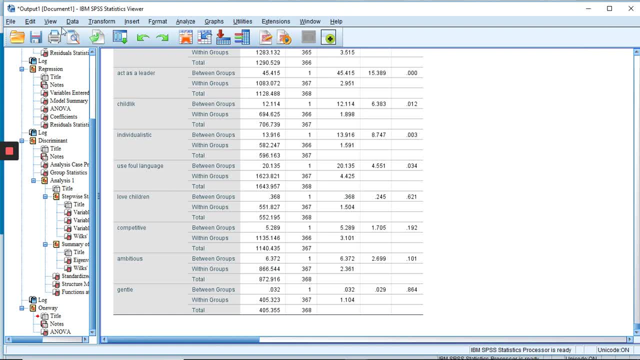 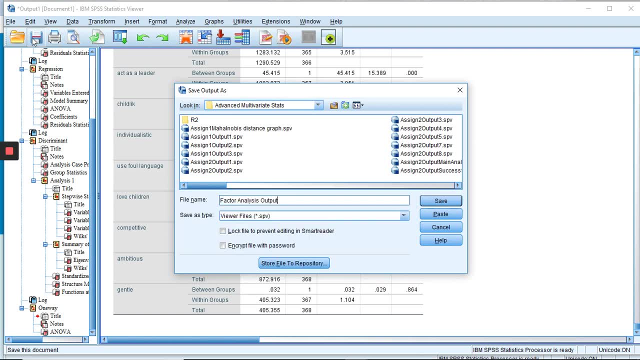 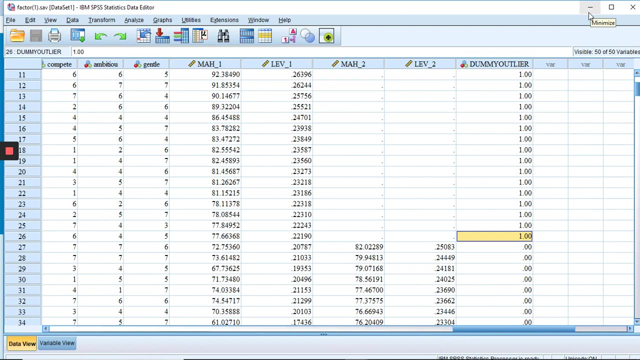 comfortable deleting 26. Outliers. So, by the way, let's save our output and we'll do factor analysis output. Okay, And let's minimize that. So now we're confident and we have them grouped here, So we can just go ahead and 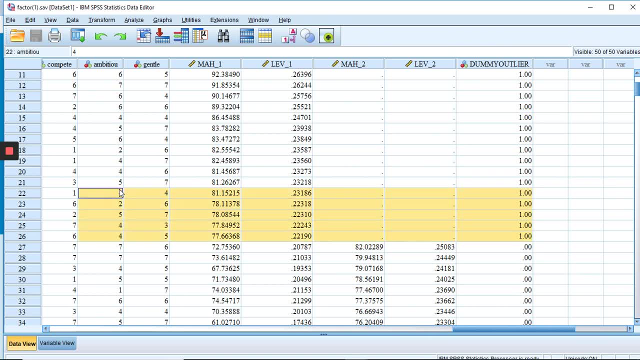 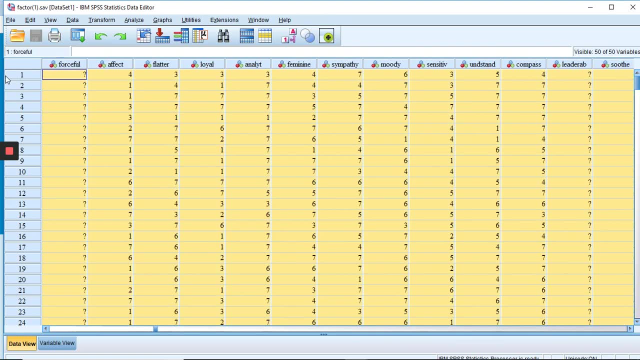 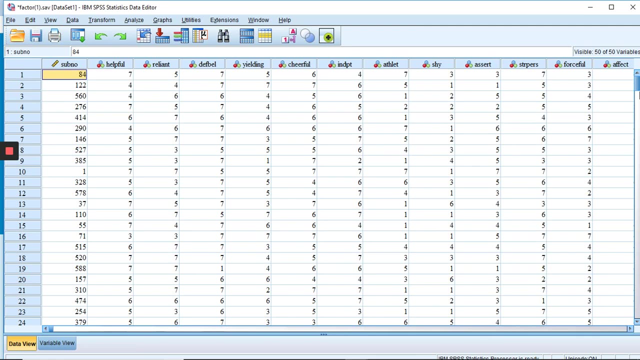 basically select the top 26 cases And we have the dummy outliers to help confirm that we're doing the right ones. Scroll all the way Over and just select the whole thing and then hit delete. Okay, Now, before you go on, make sure. 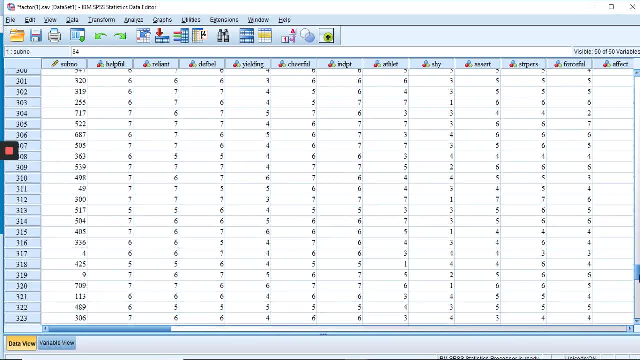 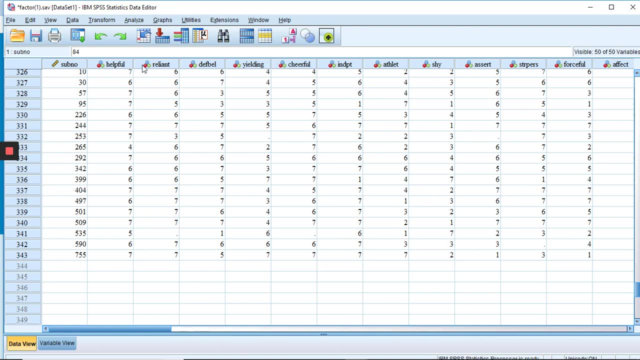 that you scroll down to the bottom here and you should have 343 cases. If you don't, then you accidentally deleted too many and quickly hit undo or you're going to have to start all over again, because it only undoes, I think, one action, So it doesn't give you a whole lot of room for messing. 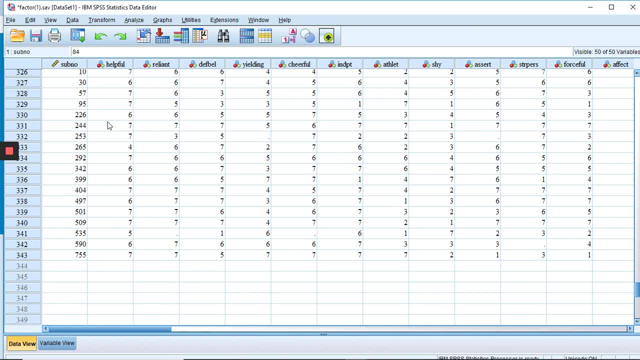 up, Okay. So now, um, we we have deleted that And um, you can explain all of those steps if you like. um, if you're writing this up as an assignment, Okay. So now the second limitation that we're assessing for. 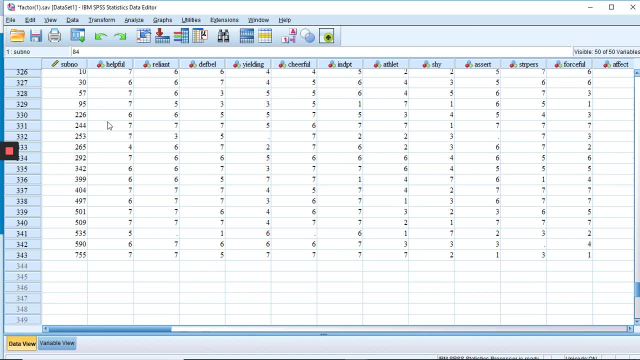 is the factor ability of R, And really what that means is we have to have at least several correlations above 0.3, because if you don't, how are you going to really group these, these characteristics right? You can see on the screen here, helpful, reliant, uh, defending beliefs. I think that one is yielding cheerful. So all of these, you know, if you have 44 completely different things and none of them are correlated with any of them, factor analysis is not your, uh, your choice, because what you really want is to group these things into, into categories. So you're looking for correlations And so, before we run the whole analysis, we can just do a quick little. 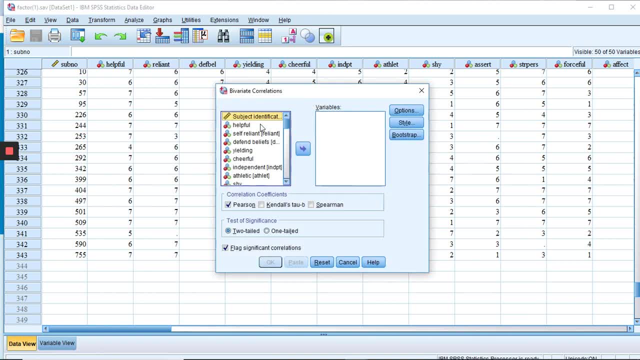 analysis, Analyze, correlate, bivariate. And Pearson is good, because these are, uh, continuous Click on helpful. scroll down to the bottom gentle there, hit shift and click, scoot them on over And um, I don't think we need any. we don't need the means and standard deviations and all that. What we're really just looking for is correlations, And this says flag, because significant. 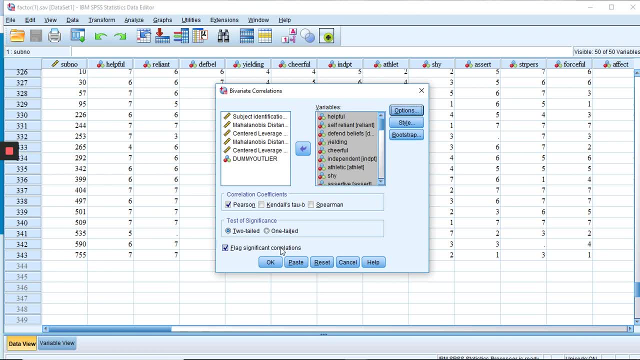 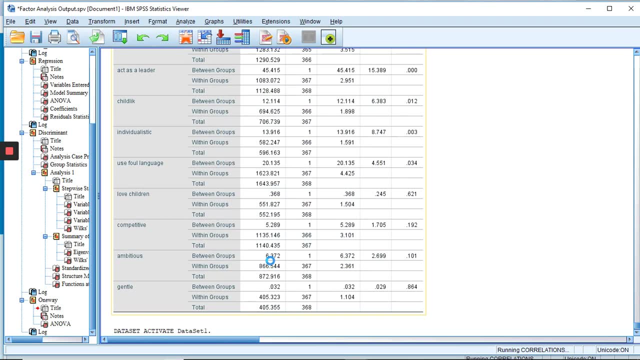 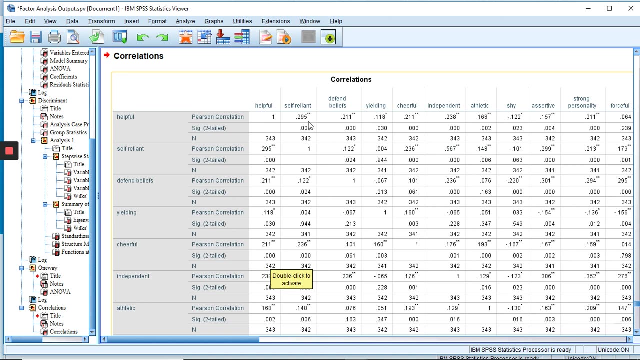 correlations. If we went into the syntax we could actually specify that we want them to be above 0.3, but I'm not going to bother with that right now because this is just a visual check. So go ahead and click Okay, And here we've got correlations and see how the two dots kind of signify some that are um are flagged, but that still we're looking for above 0.3. So our standard is a little higher: Um. now you can take some time and take a look at this chart and make sure you're looking at the line that says Pearson. 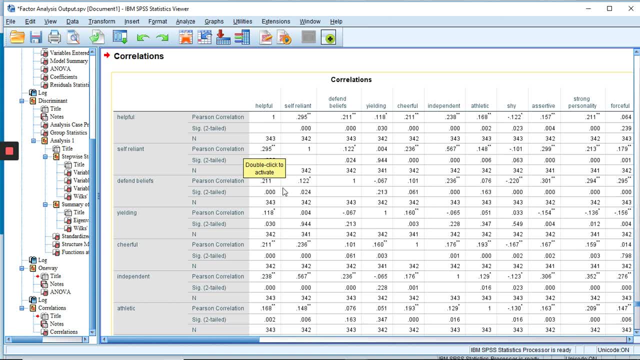 Correlation. You're not looking at the significance, Um, and you'll notice that N is different in certain places, And that's because, um, I skipped a step and we need to do missing data next. So hold on, Cause we'll do that in a second. We might as well look at this right now. So basically, um, that's funny that I missed that, Okay, Um, so yeah, basically, you can look at this, uh, to your heart's content. 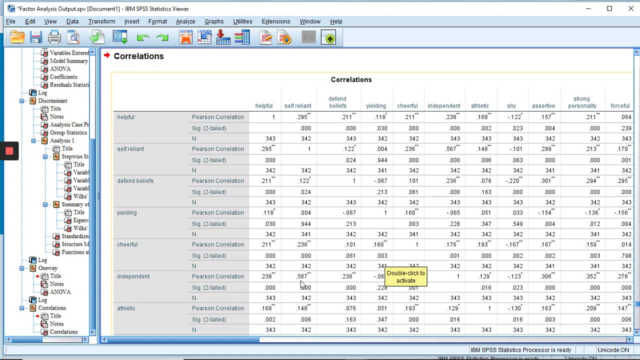 And. but here's a good example where independent and self-reliant are correlated above 0.3.. I counted like 20 before I gave up counting and just decided, yep, we have enough, So there's enough correlations in here that are above 0.3 that we are good to choose factor analysis. So yeah, I forgot, after we deleted the outlier cases, which is important to do first- that you then assess. 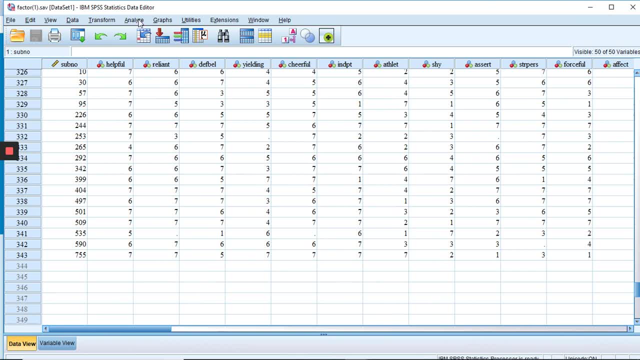 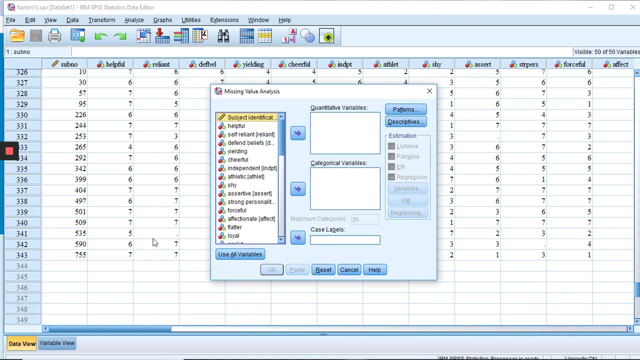 for missing data, And so a helpful way to do this is to go to analyze missing value analysis, And I really thought I wrote that down in my notes here, And so let me see if I can find that. Well, just to note that I skipped over the says: then replace missing data, Okay, So, um, okay, We want all of these variables here again, just the ones that I skipped over. 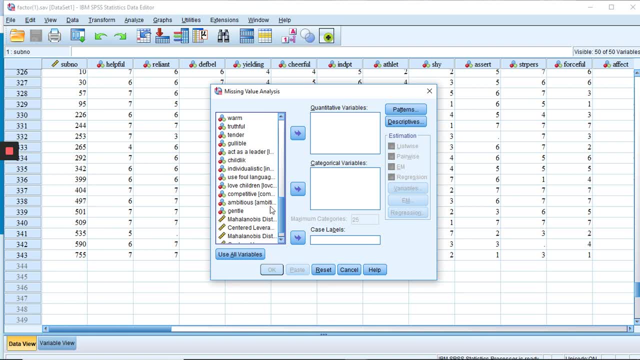 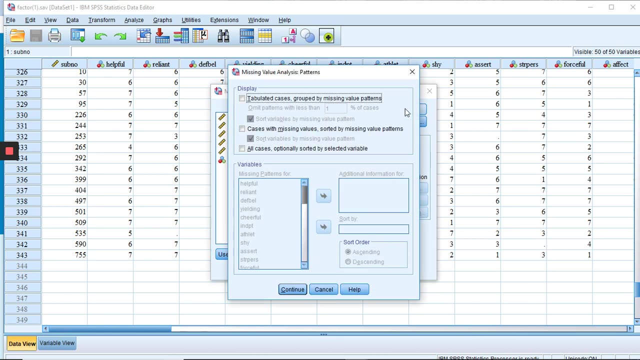 The ones, the 44, and we want this here shift over over and we want to um determine kind of if these are random or whatever. So we want, um, Hmm, Let me see what I checked off. I did not write myself, Good, 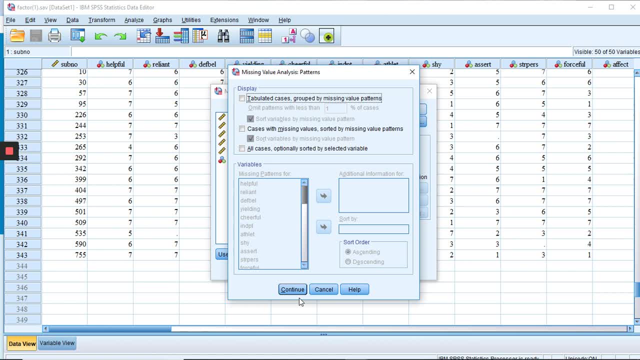 No, it's on this one, I think, because I looked back at the other one that I had done. So let me pull that up real quick. Sorry for the delay. Um, sometimes I think I have all this set and then I didn't write one thing down and then it throws me all off. So let me just check here at um the logistic regression that we did the missing Okay. 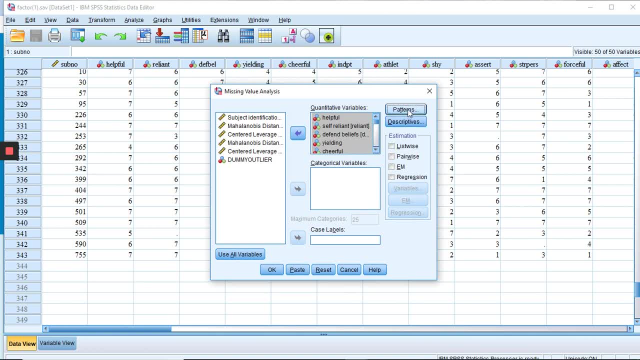 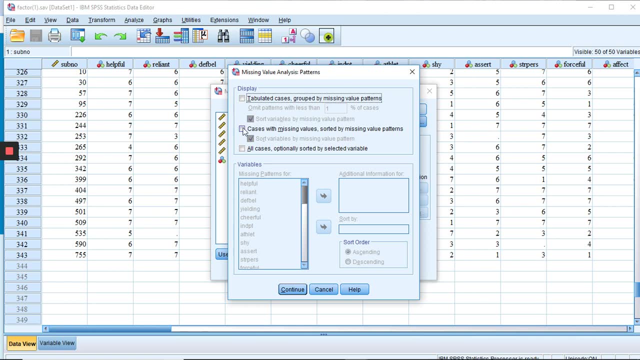 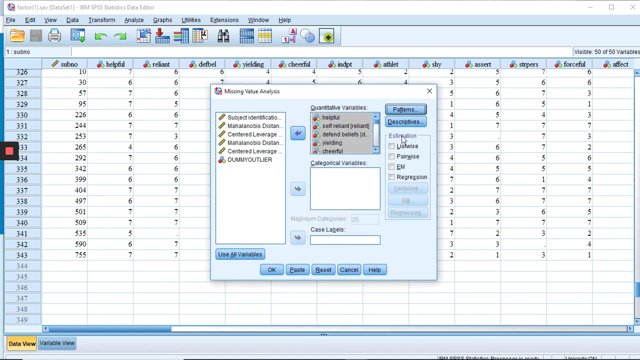 So let's look at um patterns and missing cases with missing values: Continue. Okay, And the descriptives? We want to uncheck univariate And we want we don't need cross tabulations because we don't have any categorical value variables, but we can do. 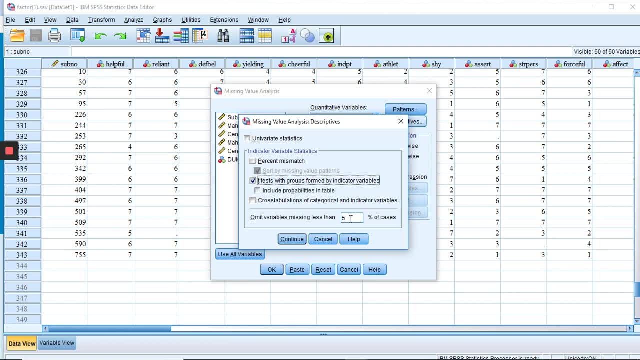 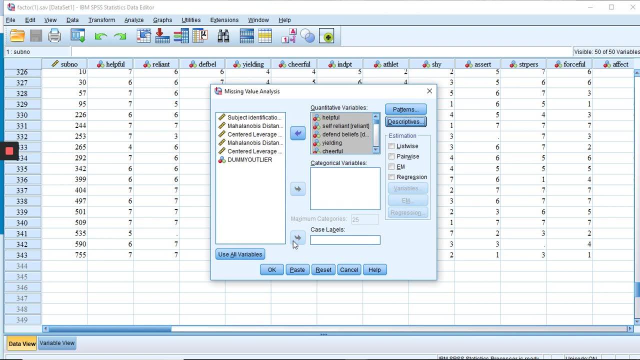 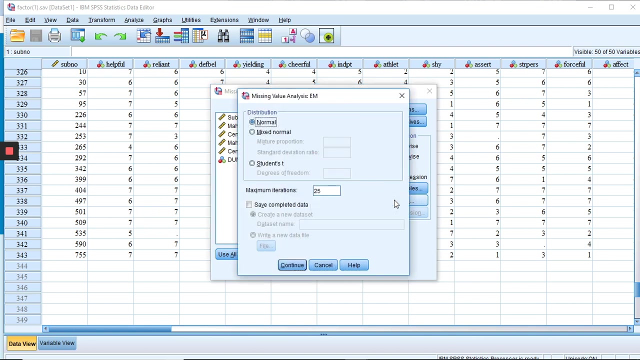 Um t-tests and we can change this to 1% of cases, just doing what I did when I did the logistic regression, And so um the EM estimation we want and then, if we click on the EM which is um, the estimated means um. 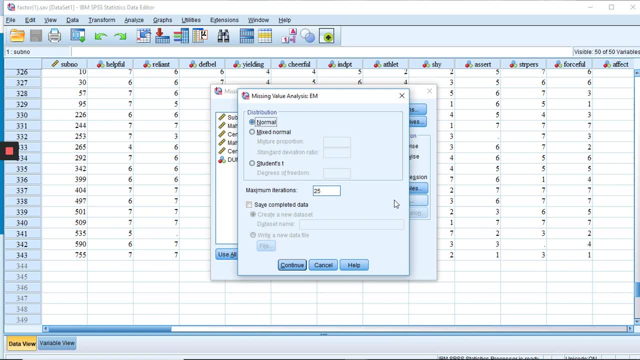 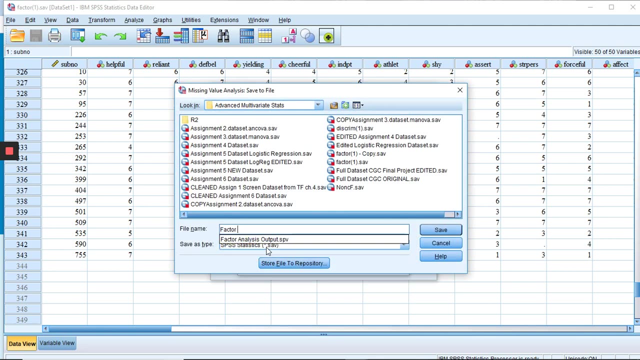 that should be normal. But then we want to save the completed data and this is going to write a new data file, And so the file here we'll call it um, factor analysis, with removed outliers and replaced it. You can call it whatever you want, but this is going to help me remember. 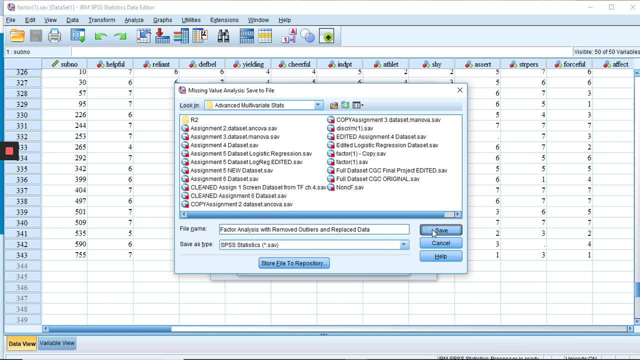 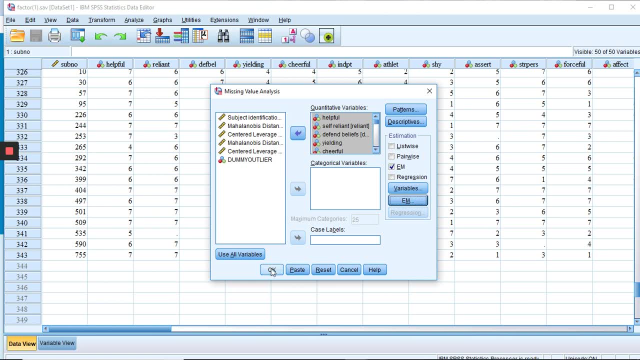 Um, and so I will click save Okay, And so we're going to continue and basically it's. the new data file is going to have Any missing um variables replaced with the estimated means, but it will show us where it is, So we can either use this one or the other one and make our decision either way. So click Okay. 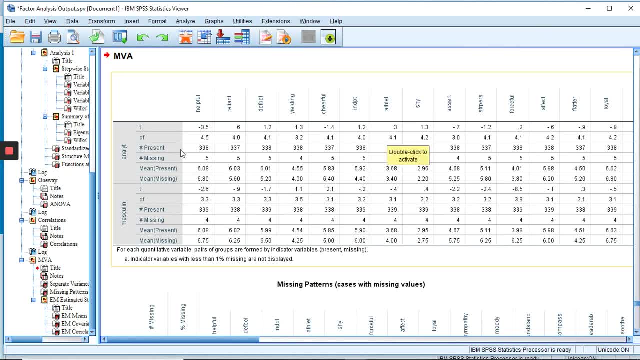 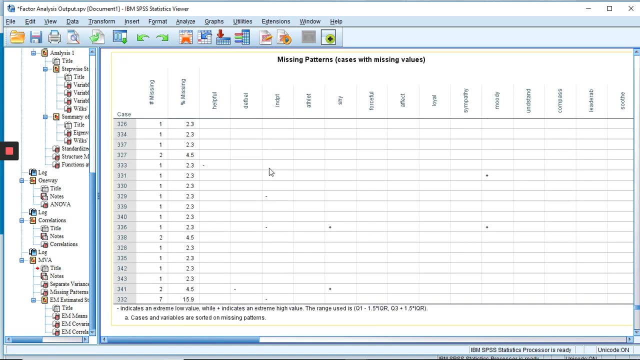 And, um, here we can see, uh, where the missing value is lie. it looks like there's two that are missing the most, and this is showing kind of where it falls. and so we can also see here kind of the the percentages. case three, three, two has seven items missing, and that's kind of. 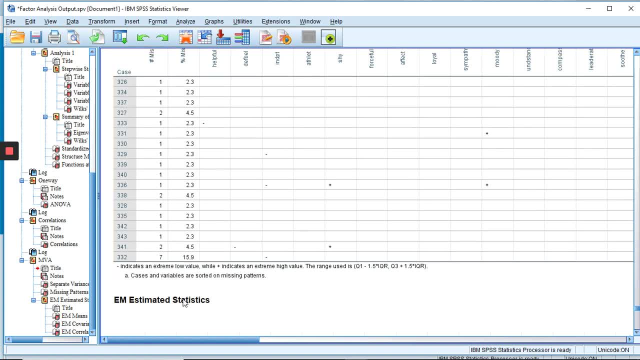 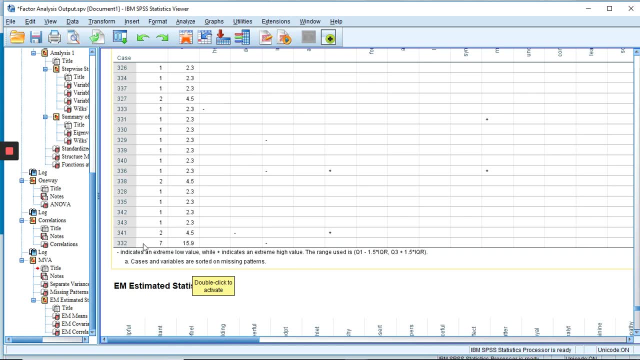 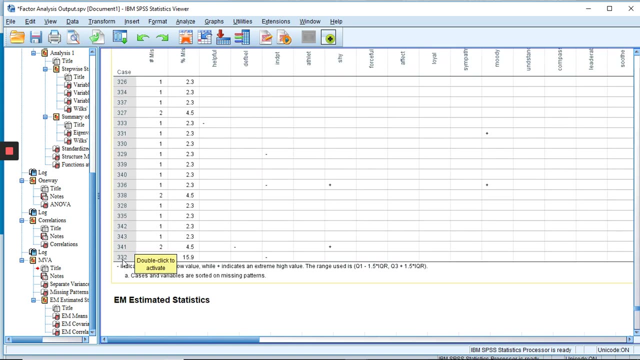 high. so actually, really I didn't. I didn't do this when I originally did it, but now that I'm looking at it again, that would be, I think, a fairly strong argument for deleting that case. and that would be the line number, not the subject number. so be careful not to reorganize your cases before you make that decision. 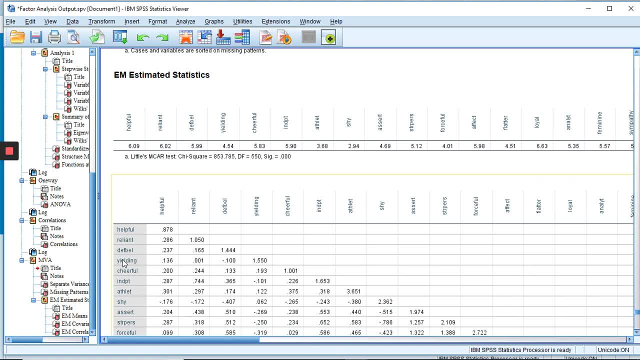 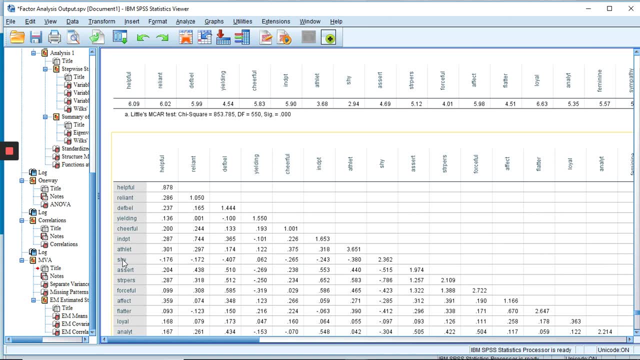 if you're going to delete that or not. so you could move forward with 342 cases. the book says that there's no missing data. I really can't understand that. so you could move forward with 342 cases. so you could move forward with 342 cases. 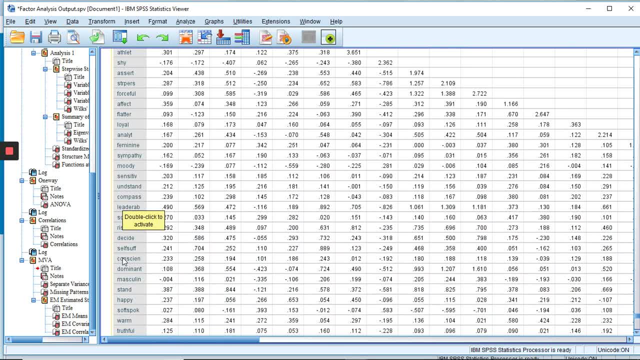 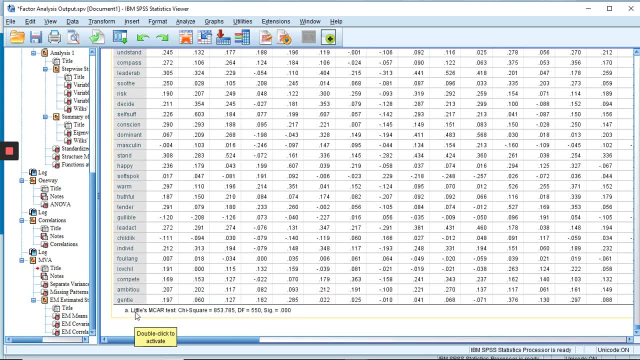 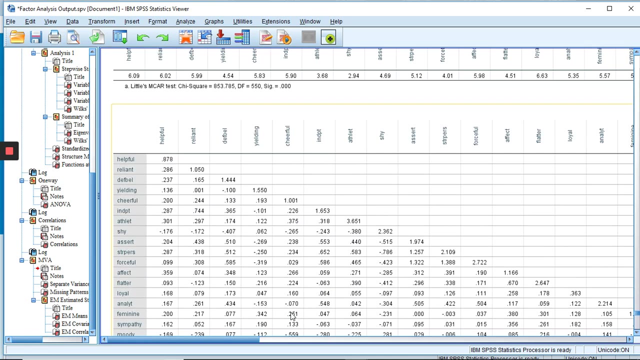 there clearly is missing data in this data set file, but anyway, if we scroll past all these charts and look at the very bottom, here Littles MCAR test is significant, which is a problem because that means that it's not necessarily randomly missing. however, I felt that because there was not a ton of variables. 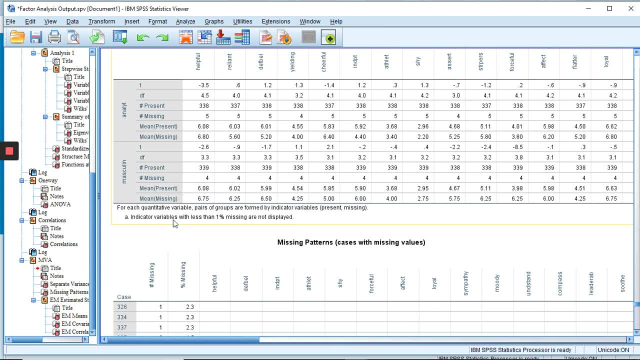 with a huge amount missing. it says indicator variables with less than one percent missing are not displayed. so it's just really these two, and it's not even that high. it's five cases and four cases. so I went ahead and just used the new file, so I'll save. 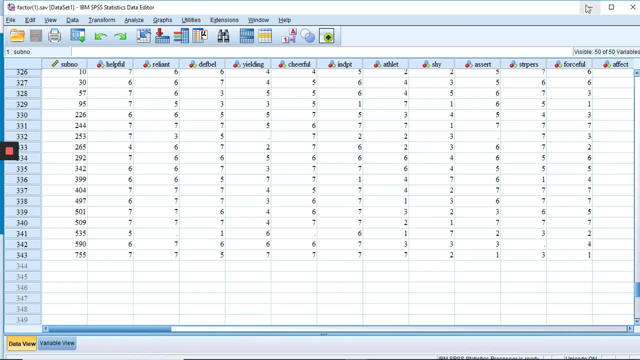 this output and then I will go down, and so this is the old data set and you can even see right here: this is the line that we would be talking about. I think three thirty two was the one that was missing the most. they had seven or so. so if you want to delete one more case, you could. your numbers will vary. 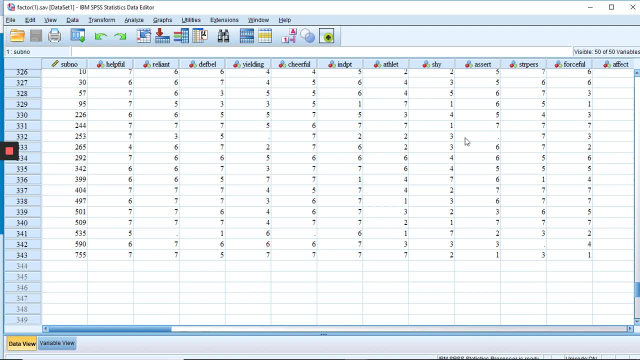 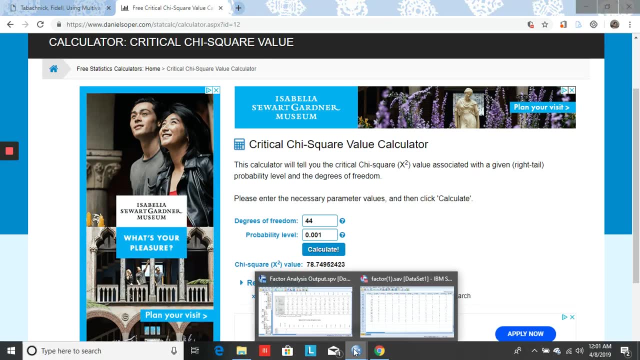 from mine, because I'm going to proceed just replacing the estimated. so let's just take a look at minimize this here and we should have a new data set to look at, do we? maybe we need to open it up. let's see if it saved it down here. 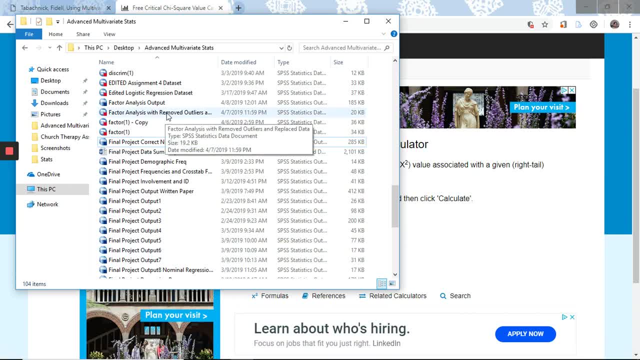 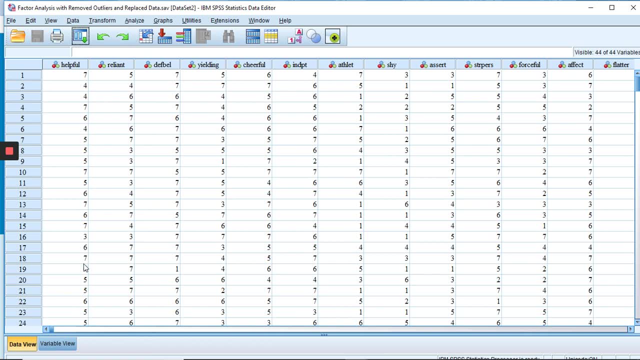 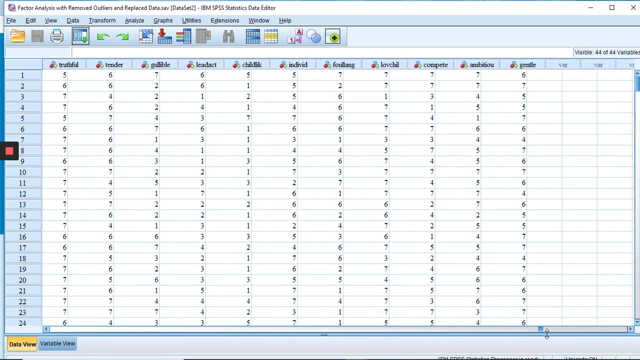 factor analysis with removed out. Yep, Okay. So wherever you, whatever you chose to call it, and wherever you decided to save it, go ahead and open that one up, And I don't think it's going to have the Mahalanobis distance um ones in here, I think it's just gonna yeah. So now it's. 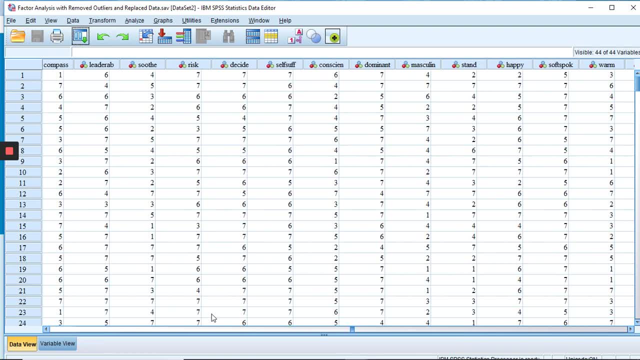 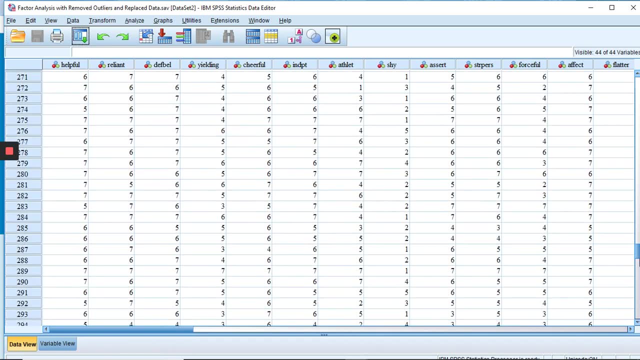 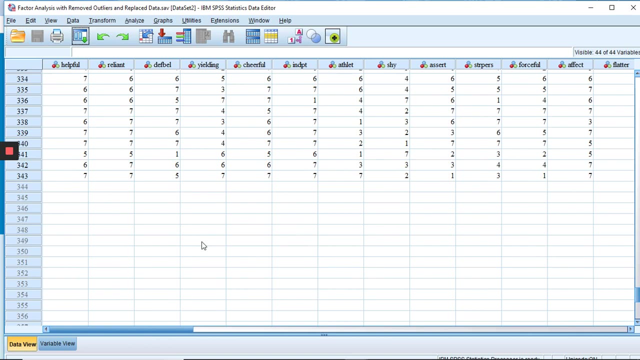 basically a new data set with now no missing values, and it's still going to have our outliers deleted, because obviously we deleted them, So you can't question that. So that's 343 cases. Again, if you had chosen to delete the one case that has seven missing points, then you could have 342.. 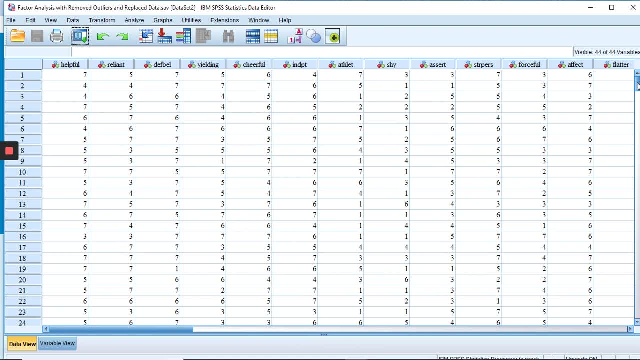 So we will proceed with the remainder of the analysis with this data set, this new data set. So if you need to go back and look at the Mahalanobis distance or the leverage values, that was all for determining the outliers And since the outliers are done, we don't need this anymore. but I may? I for my own assignment. 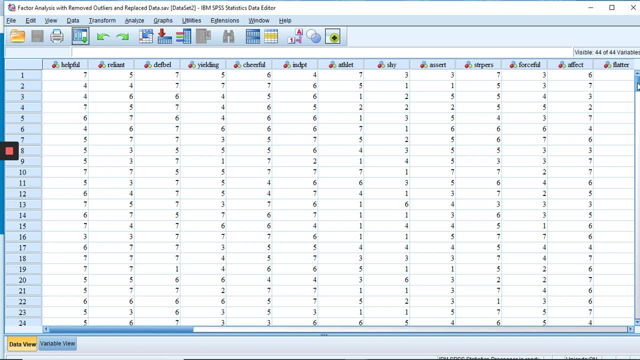 I might turn in both data sets to kind of show my process a little bit. So, um, that's just up to you. Okay, Now we are back on track. And so now, um, we talked about the factor ability of R. 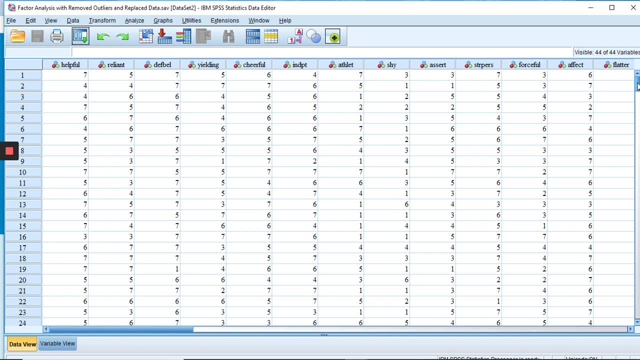 that's the correlations we were looking for above 0.3.. And so you can count those up and then we can move on to normality and linearity. So now that we have eliminated some outliers, we're going to check um for skewness, And that's really the only thing we're going to. 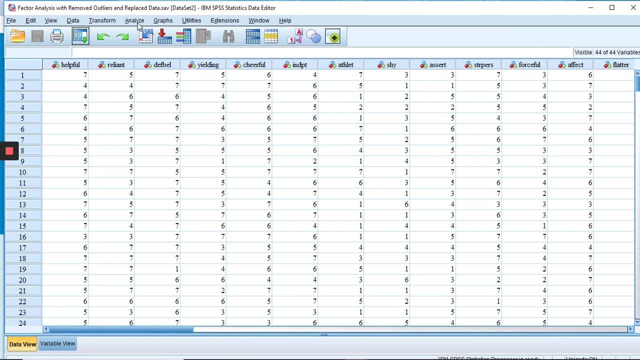 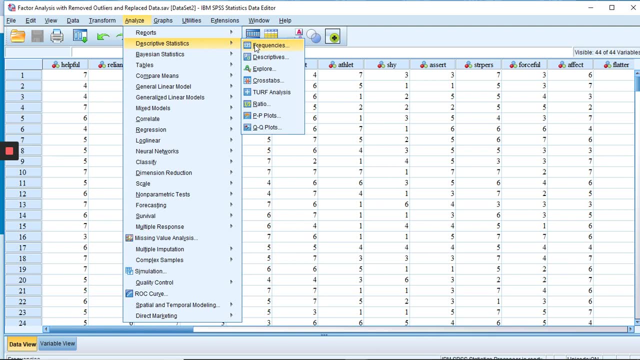 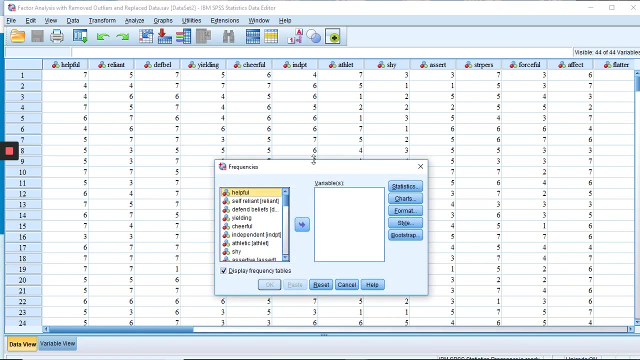 use to measure normality here. And so if we go to analyze descriptives and um frequencies, um, no hold on. Yeah, that should be right. And all we want is skewness, Okay, And then we just scoot all of the variables over. 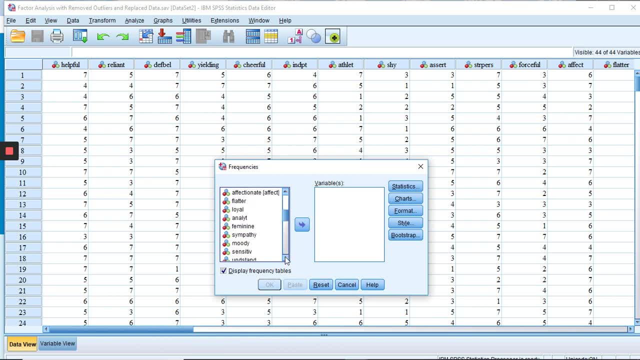 click on the top one, scroll all the way down, click on the bottom one, holding shift, And there we go And displaying frequency tables. Um, I, yeah, we're going to want that because we're going to want to have a lot of variables, So we're going to want to have a lot. 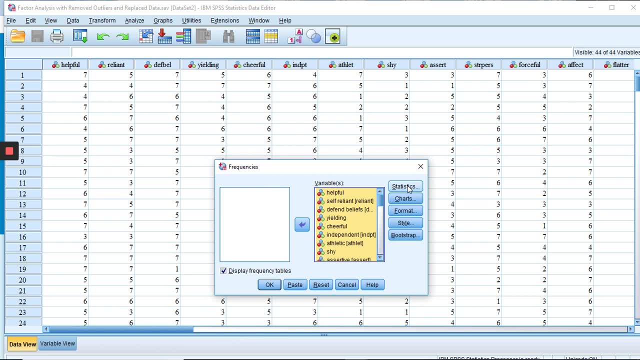 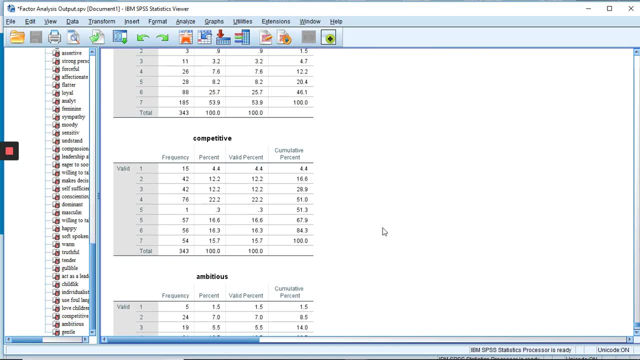 of variables because we're going to want- um, we're not really looking for plots here, We're looking for the skewness. So that should be good. Click, Okay, Uh, oh, okay, Yeah, Nope, We didn't. 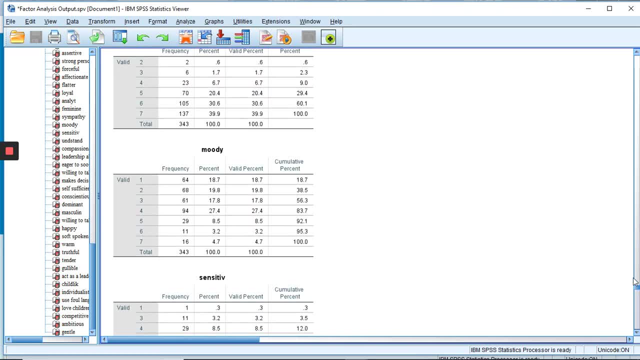 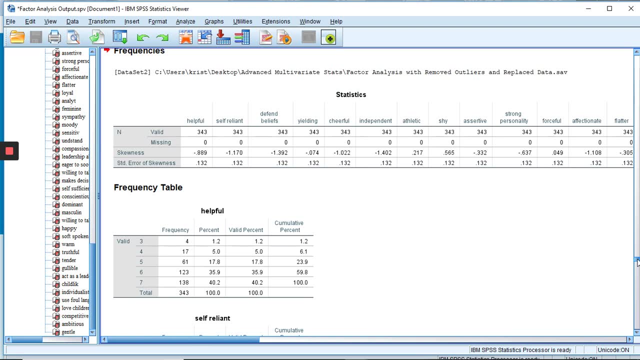 need the frequency tables. This is a nightmare. Um, let me see where it gives us the skewness. I don't. I must've unchecked this. Yeah, I unchecked that before. Okay, Rewind and uncheck that. Um, okay, And here, by the way, you can see all of our beautiful zeros and the missing data. So, 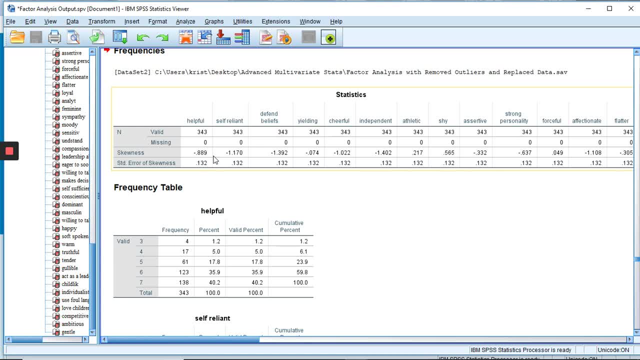 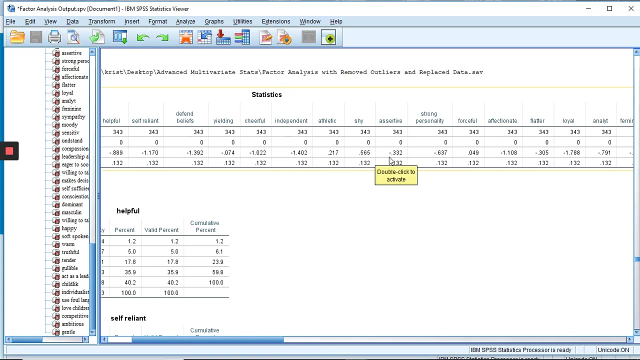 everything is is clear now. Here's your skewness, And so what you want to look for is ones that are above one or below negative one, And so you can note them. We've got self-reliant here, defending beliefs independent, So you want to jot down the ones that are. 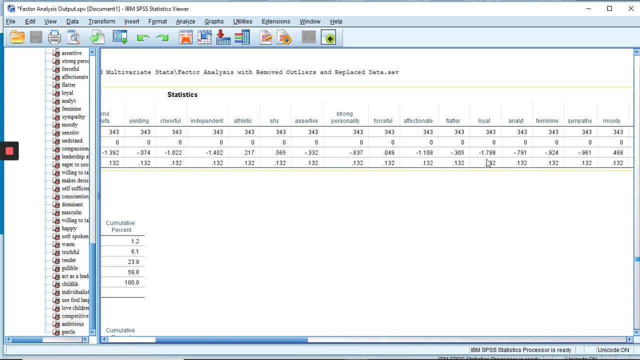 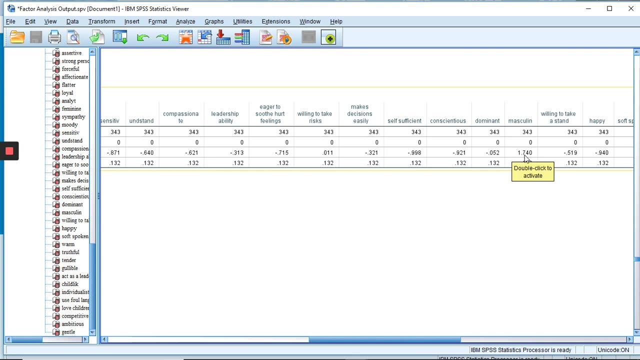 are kind of stronger, So loyal here. we've got some skewness over here. Um, and keep scrolling all the way over. here is masculine, which is up in the positive side, So some are skewed to the left, some are skewed to the right, Um, and so what we're going to do? 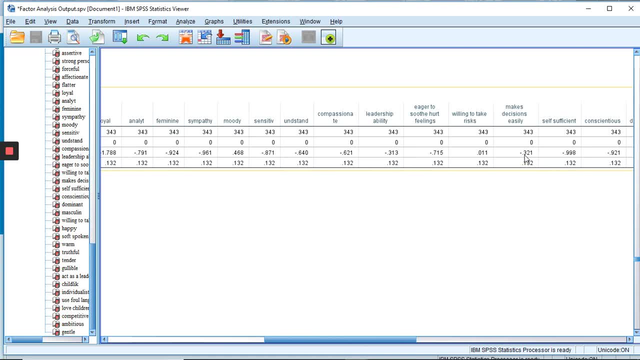 is really assess the ones that are the most different. So I will tell you that, um, I used three of the of the lowest. So, um, loyal is the lowest, it's negative: 1.7, 8, 8.. Um, and that should be. 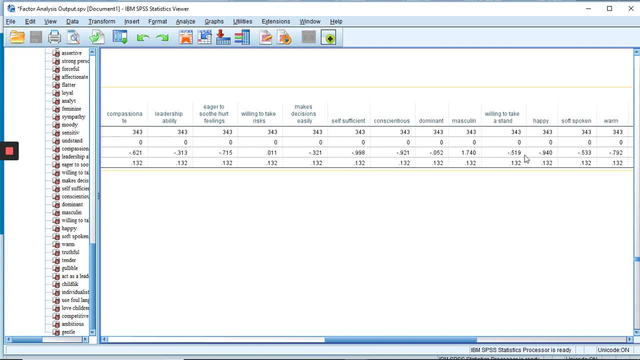 what was loyal. again, Let me check that number because, um, I don't remember how, but something was different when I was doing it. Oh, okay, That is right. Okay, Yeah, So um, negative 1.7, 8, 8 is the lowest, And then 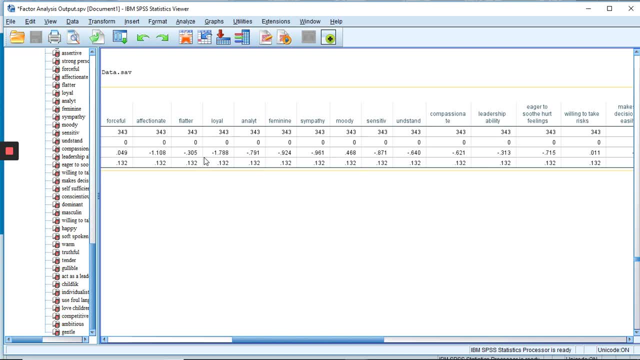 love for children is um negative 1.651.. So you can look for that somewhere over here. There's so many variables. It's a little bit cumbersome to dig through all of this output. It really took me a while to just get my bearings. to be honest with you, wherever love for children is, here we. 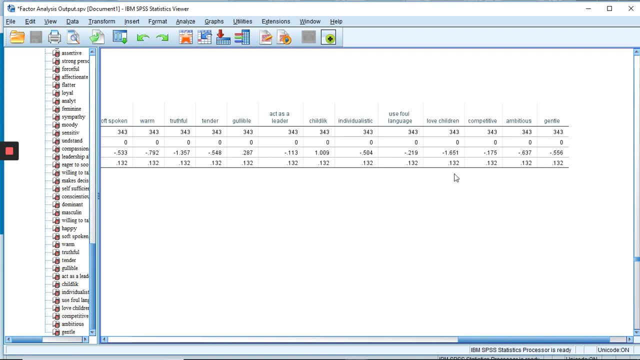 go Love children. So you can see that one there is negative 1.651.. And then independent is negative 1.402.. Then on the positive side, masculine was positive 1.743. And childlike um, right here, is 1.009.. So if you um want, what we need to do is to test for linearity. 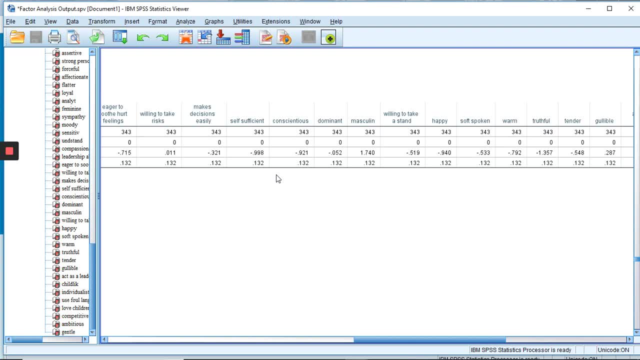 Um, so, basically, you count how many variables have skewness, either above one or below negative one, which I will tell you: there are 11.. So, um, essentially, um, it's not great, but we also have a situation where we cannot change the variables or transform. 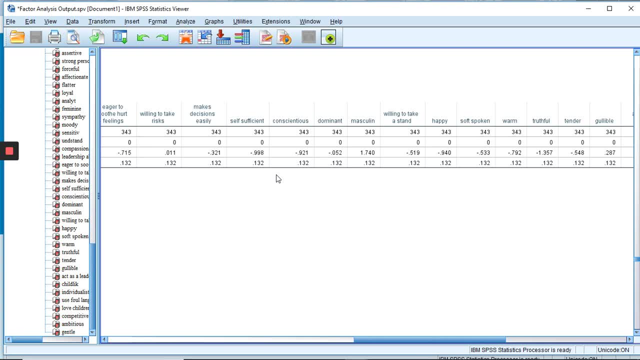 the data in any way, because this is already a published inventory And so if you were making your own assessment tool or something, then you might want to uh, transform some of the data, um, do a log or something like that, But because we can't do that, 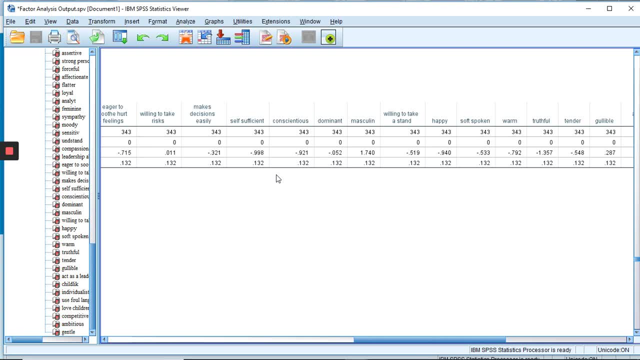 we have to just kind of accept it. Um, although the good news is there's not any that are like so egregiously high that we couldn't continue. Um, I don't know what value that would be, but certainly, you know, um beyond two, or you know really high, would be a problem. 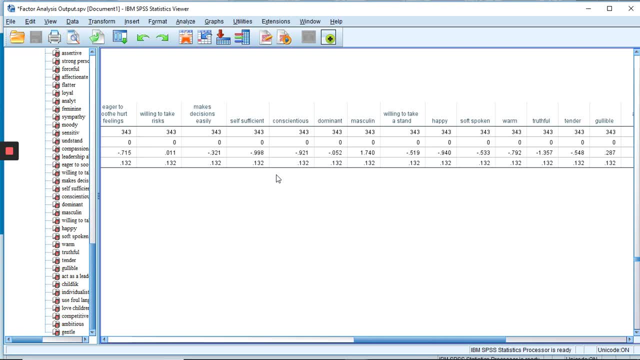 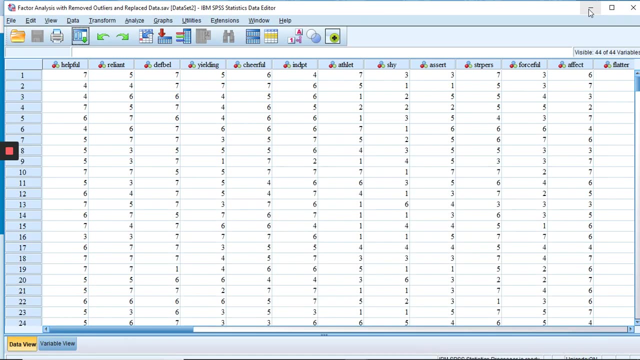 So, um, we're going to proceed. That's where we're looking for linearity. So it would be a lot of combinations to look for every single one you saw with the correlation matrix. I mean, imagine if you did that many scatter plots, that would be crazy. So we're not going to do that. We'll minimize our output here. 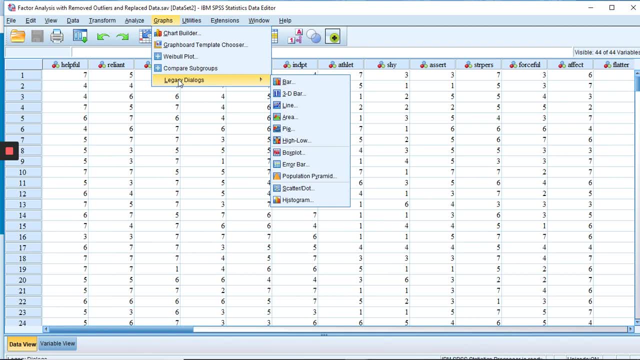 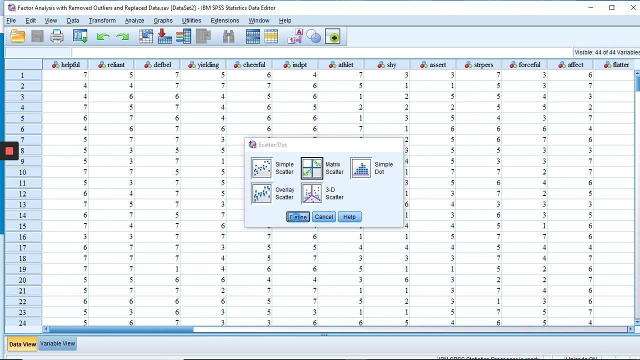 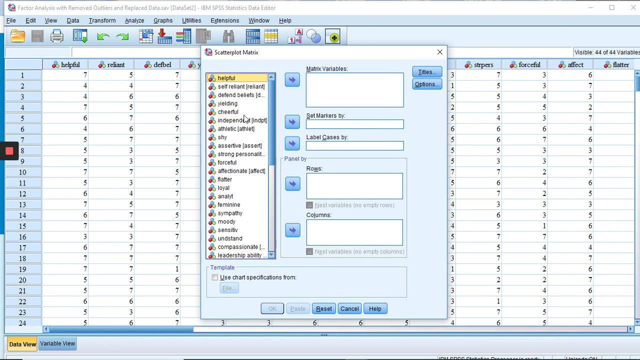 again and go to graphs, legacy dialogues and scatter dot, And what we want is a matrix scatter of the ones that are the most negative or the highest positive. So that is um. we're putting in those matrix variables, So we're looking for loyal um, independent masculine. Let's see where's masculine. 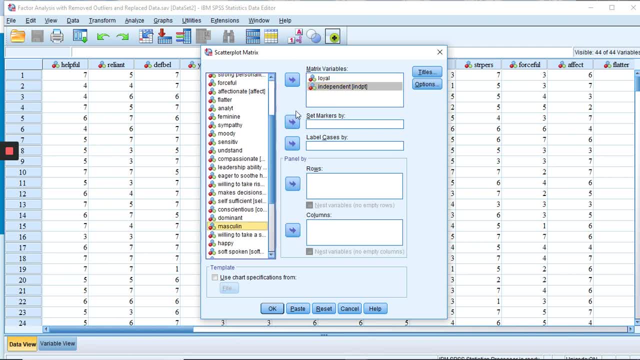 masculine here: Um, childlike that's down towards the bottom, Um, and then um love for children. Oops, sorry, Okay, So that's it. We just want those five because ultimately we're not even really looking at all five of the combinations, What we're really 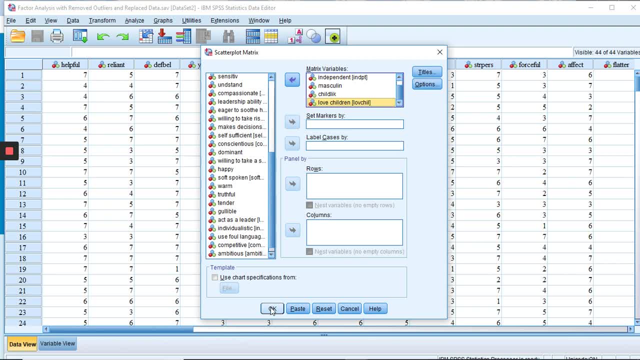 looking for is, um, the, the positive versus the negative. So we're going to kind of compare masculine and childlike with the others and kind of see what we're looking for here is. a great thing would be an oval shape, But if there's a very clear U shape then we have a problem with linearity. So go ahead. 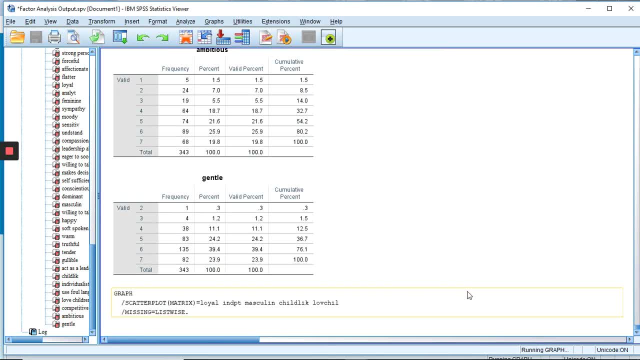 and click, Okay, And it's going to take a second. Sometimes with the pictures it takes a minute. Okay, Hmm, Taking some time here. Sorry guys, just this is a moment to you know. sip some tea. 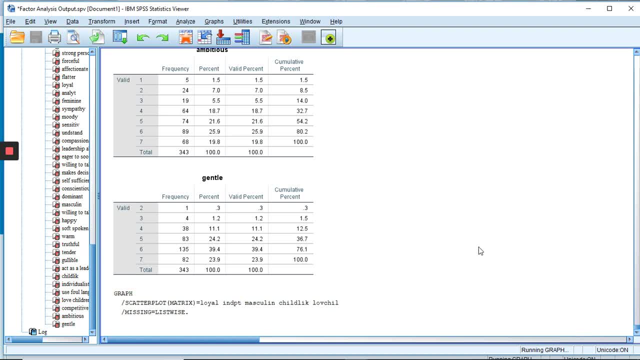 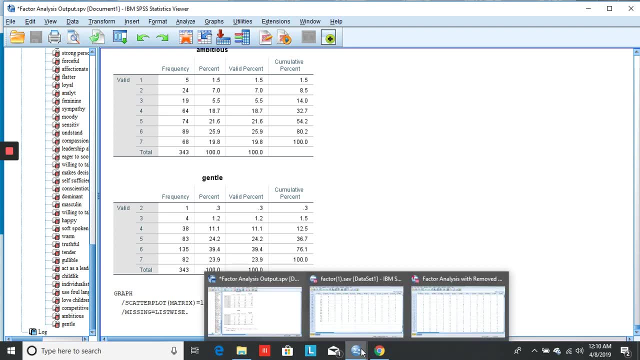 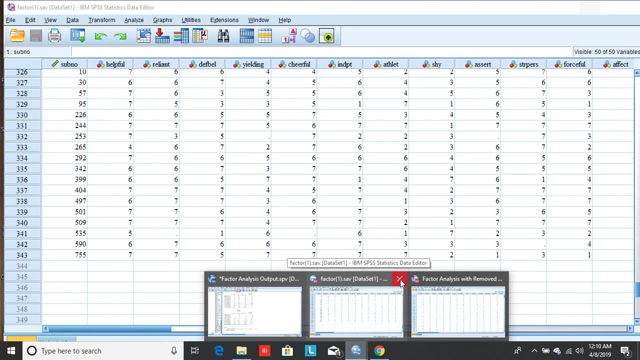 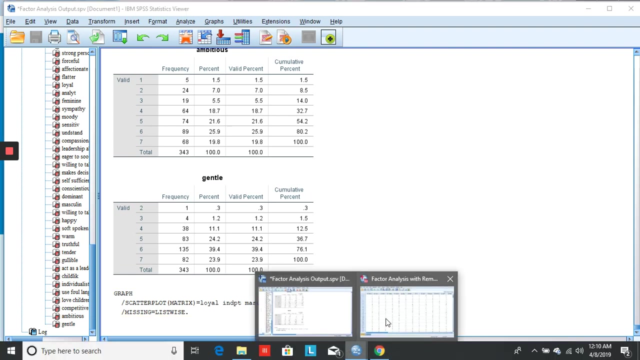 relax, It's okay. Wonder what has happened to our beautiful graph. Maybe we should close one of our data sets. That was our original one, So let's close it. We're not using it anymore. Maybe that will help us. Oh graph, Where are you? 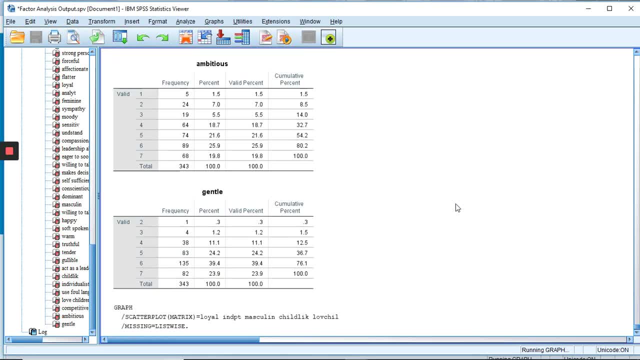 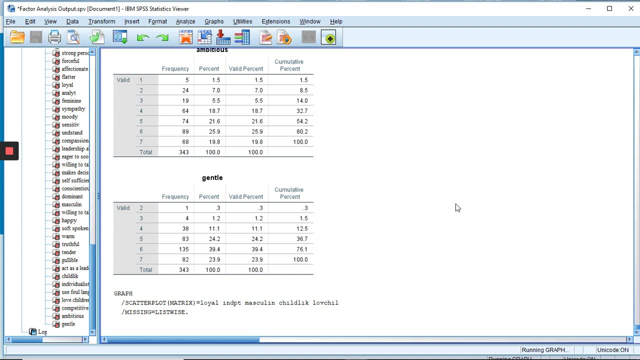 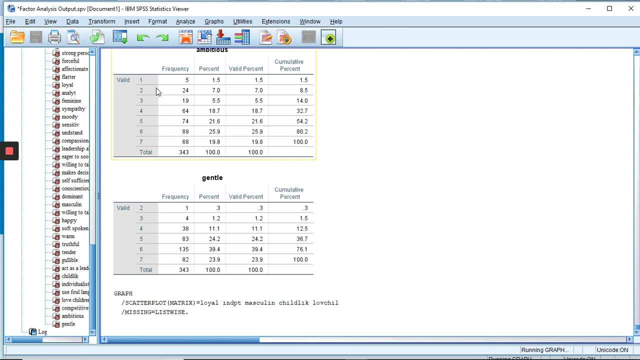 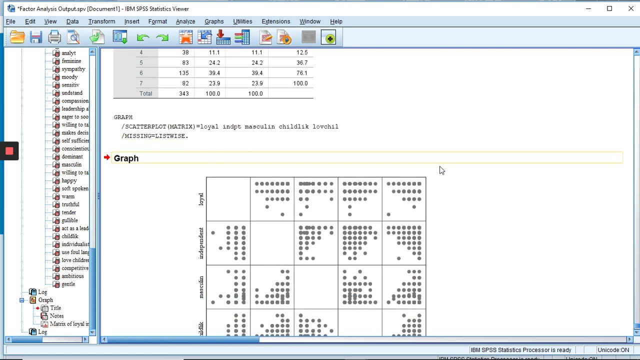 know, Let's take a minute and wait for the computer. Let's just take a moment and appreciate that It's not just you. Okay, guys, I literally had to pause the video that took so long. I don't know if yours took that long. 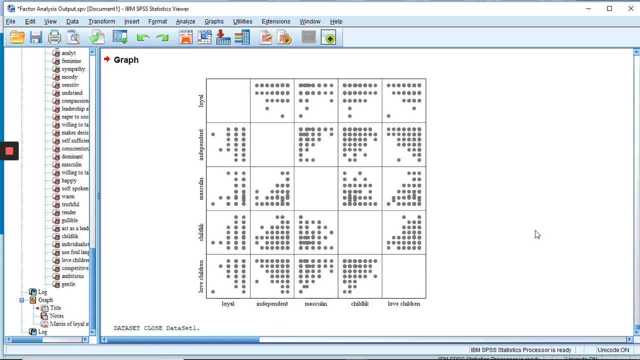 but wow, that was crazy. Okay. So here we have our scattered dots And, as you can see, because we chose basically the worst possible combinations, so once again we're in the data set scene And so we have to use these for each, for each of our data sets, right, And the math this: way. But when we click you see how it's Woods And okay in the office here. but notice this number thing. you can also use regular klip and start here to use it. right? I'm going to actually click to open the Huawei calculator. We're going to click the. 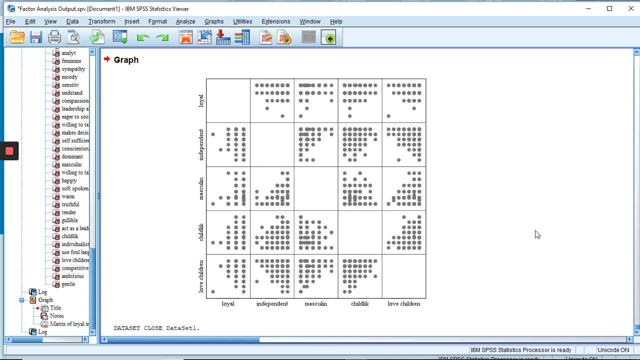 possible combinations of variables. They're not that beautiful, but we don't have any that are in like a really obvious U shape. However, the worst would be masculine versus loyal. So here's masculine, here's loyal. Oh, that looks a lot like a U, but you know what The book says. it's okay. 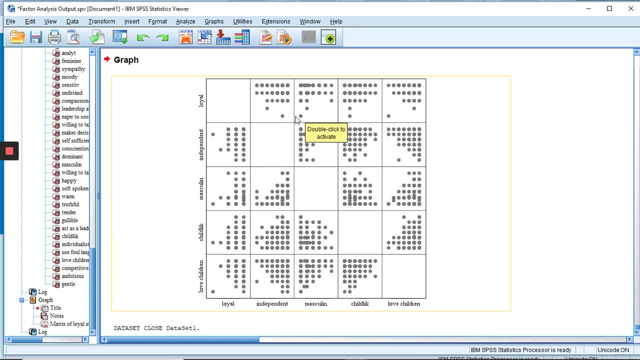 And so it's not a perfect U. I mean they use words like it's not true, non-linearity or whatever. So it all depends on how you want to interpret it. If it were me, I would say: ah, maybe we should rethink this. But again, we're not in a position to rethink. 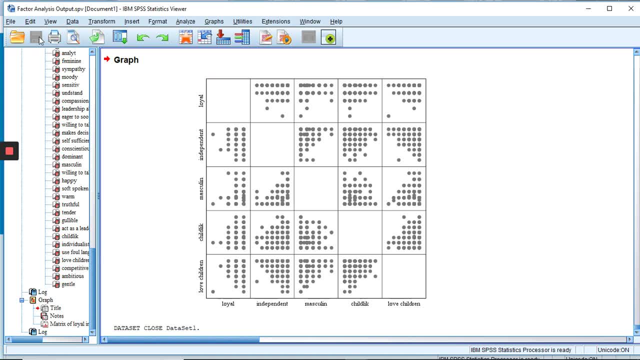 these variables, And so we have to live with them. So, basically, you can explain all of that. show this graph and explain that it's not as bad as maybe it could be. Okay, So that is our linearity explanation, as unsatisfying as that is, And um, now we're going to look at. 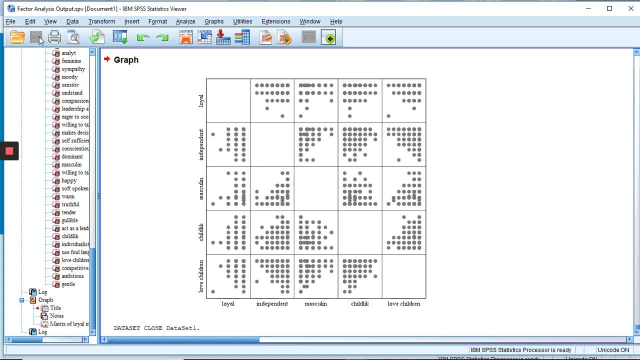 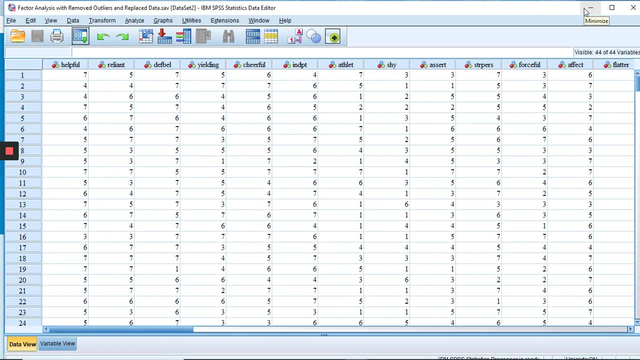 multicollinearity and singularity. So I know you guys are so just excited, thrilled to be here, And, um, so am I really. I mean, what a privilege right To figure stuff out. Okay, Just keep it in. 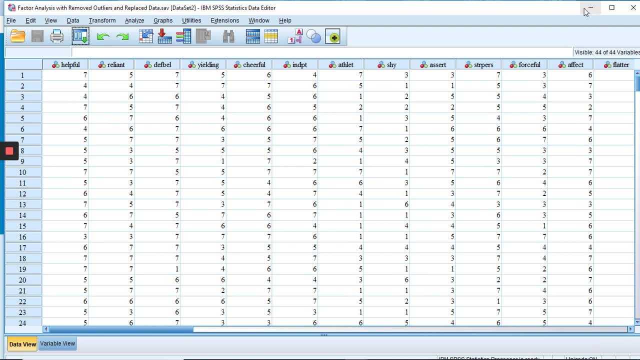 perspective. People were figuring stuff out and it's actually going to be kind of cool at the end. So spoiler alert: stay tuned, It's going to be great. Okay, Multicollinearity: We're going to actually look at when- after we do the factor analysis part, because we need to make sure that. 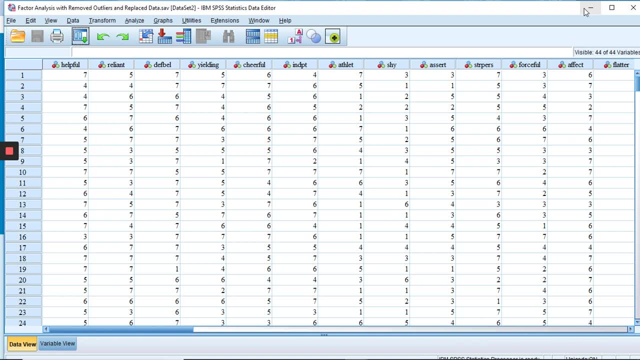 they're. all of the eigenvalues are above um zero And so, um, we're going to make sure of that. We can also look at our collinearity diagnostics from earlier. Um, so why don't you go back to your output actually? 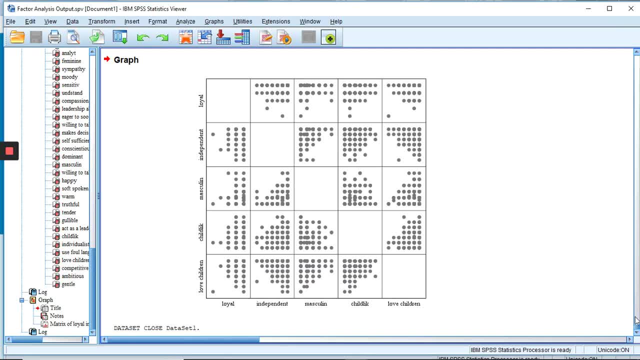 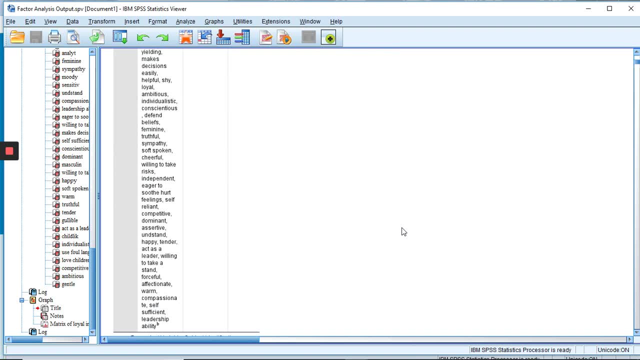 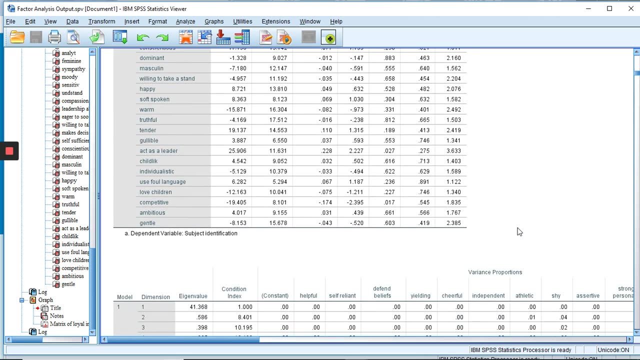 And kind of take a look at that. Um, if we go all the way to the top with our now see, this is where I was questioning myself in terms of now we have removed the variables, Uh, I mean sorry, remove some cases, And so here, Oh, and that's just that's interesting, that that has eigenvalue. 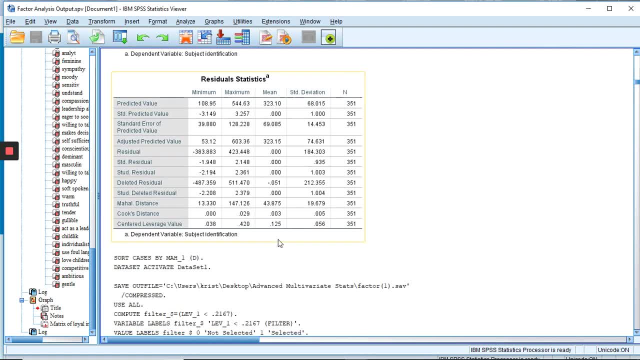 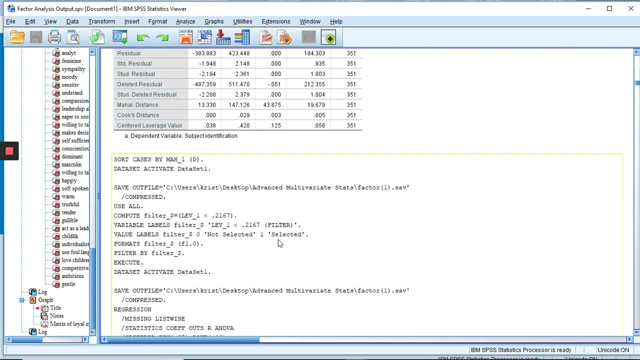 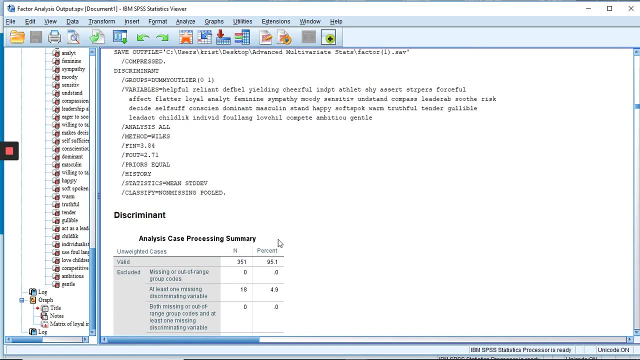 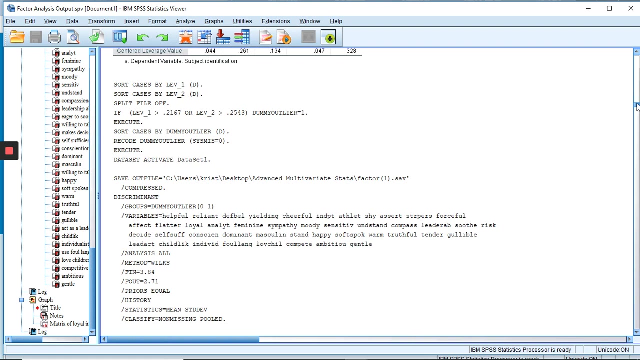 but that's different, that that comes out different, So don't pay attention to those. Um, what I am looking for here is the collinearity diagnostics. Where was that? This was our second one. Did we not check off collinearity? I know we talked about it, Where did it go? 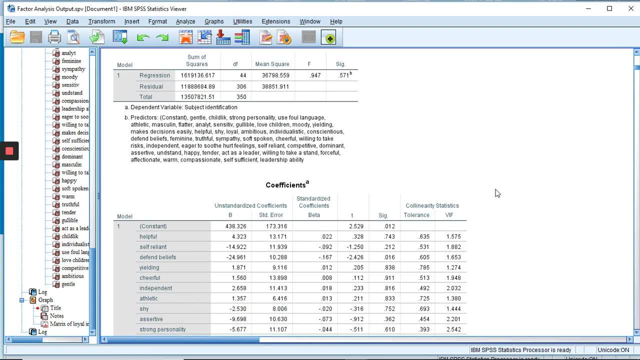 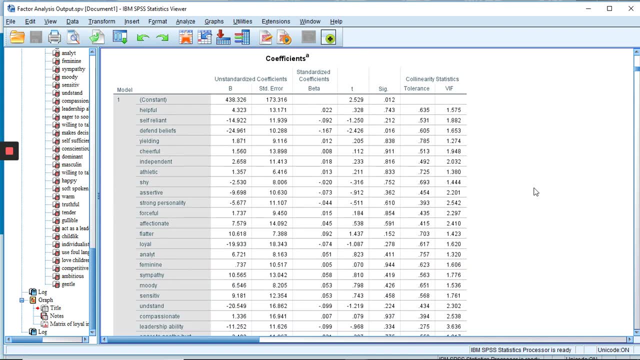 I don't know what. that is Okay, Um, Oh yeah, Hello, Here, it is Okay. You guys are probably shouting at your computer like hello Kristen, but I can't hear you. So isn't that sad. We can't really collaborate, Um all. 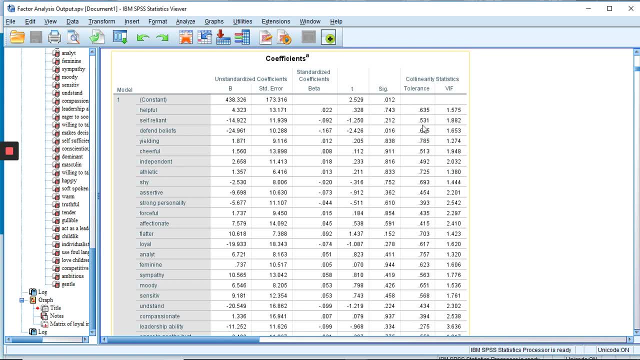 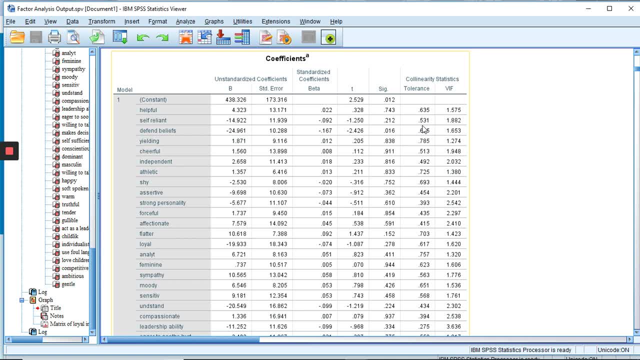 not given to us by SPSS, Unfortunately, it's one of the worst things about this chapter. So, but one minus the tolerance is equals the SMC or the squared multiple correlation. So basically, if, if the if it's one minus the. 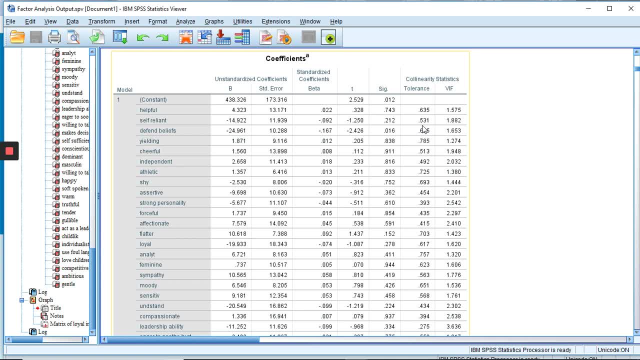 tolerance and we don't want it to be too close to one, then we basically want big enough tolerance values. that gets farther away from one. So if the tolerance is super, super small, then one minus that super, super small thing is still close to one. So that's another way we can look at this, as well as we will. 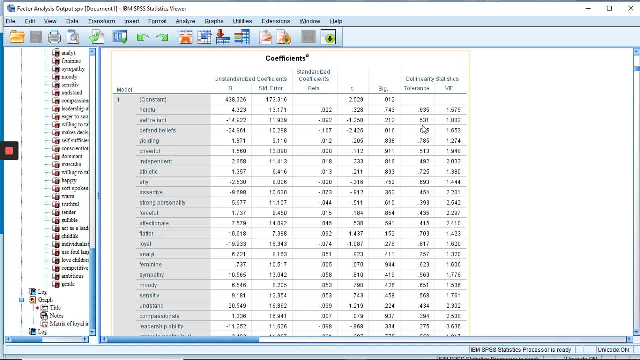 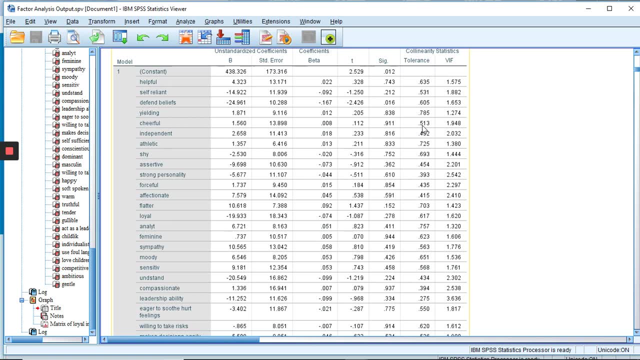 make sure that our eigenvalues are well above zero later. So let's just take a look at these while we're here, And this is also going to be important for when we're looking for outliers among variables. So again, any any. 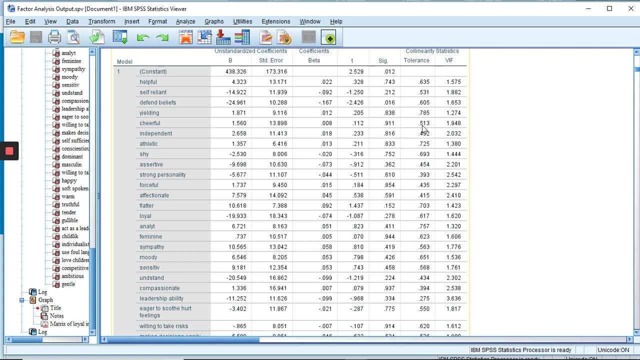 any variables that have a high squared multiple correlation are going to be a problem and we might want to delete them. So let's just kind of consider all of these areas at once while we're looking at this little chart here And essentially just remember that a low SMC squared multiple correlation, which is what we, what we do. 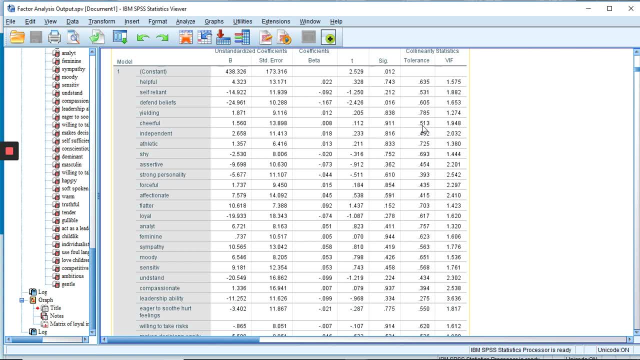 not want or we do want, hold on, We want. I wrote down: low SMC equals high tolerance equals bad. So but that's for the outliers among variables. So I'm not sure actually if that is what we are thinking about for multicollinearity, But anyway, please comment. 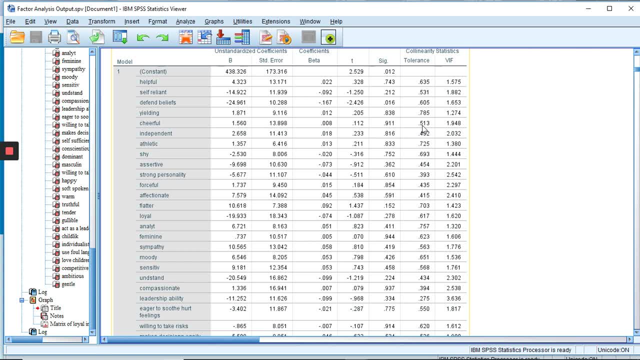 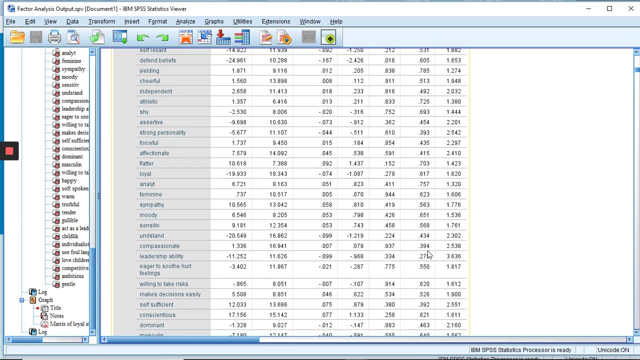 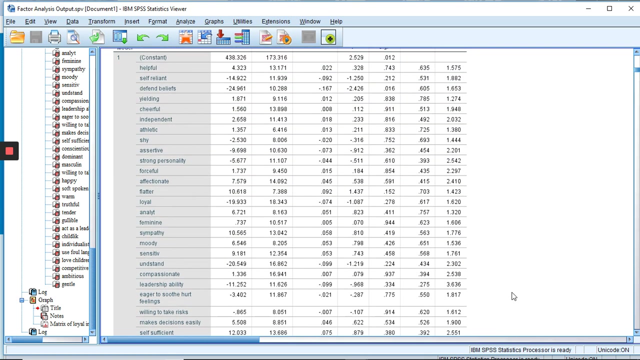 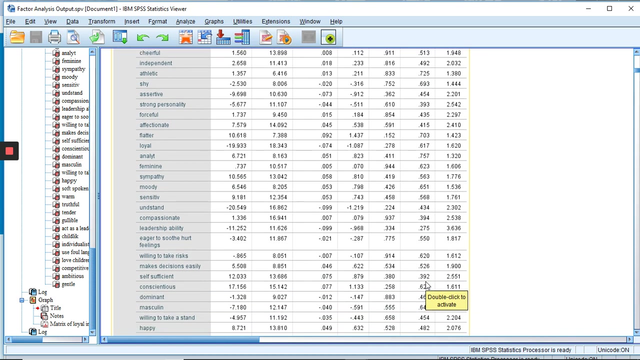 below if you understand this better than me, because then we can all learn together. Okay, So um, for now, let's go back to our discussion about multicollinearity and singularity, And I'm sorry that if I'm confusing you with too many things here. basically, let's look at this for any low values of tolerance. right now That's what we're looking for, And it looks like they're all pretty good. Now, if we look for a high tolerance, which will be the outliers piece, 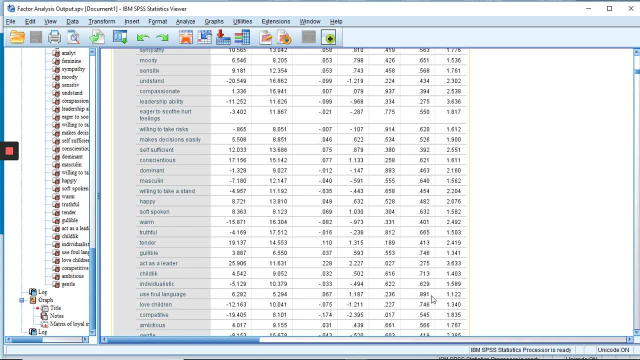 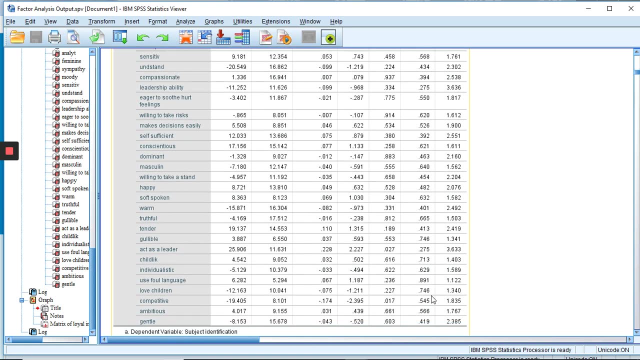 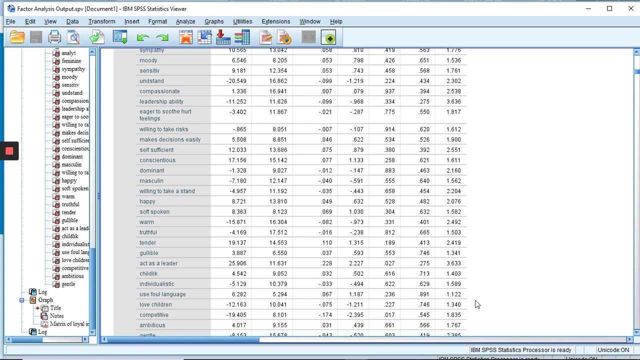 that. what I found was that this one right here use of foul language- is .891, which creates a very low SMC because it's one minus .891. So that one was the most extreme case. where you do look at the outliers among variables, It just shows they kind of don't fit anywhere. You can also, after we do the main analysis. 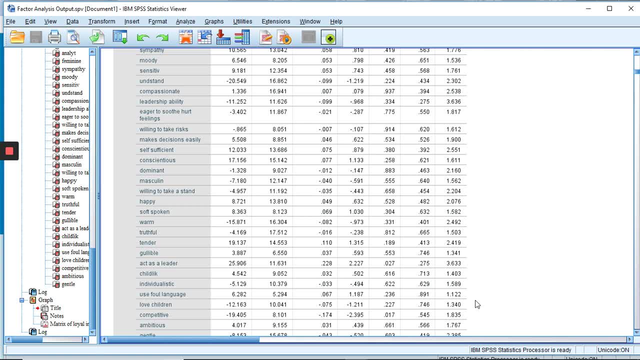 see how that one, you know if it fits with any factors. but spoiler alert, it doesn't. So that one has that particular variable has quite a few problems as we'll go along here, And so we could argue for that one being an outlier among variables. but essentially, 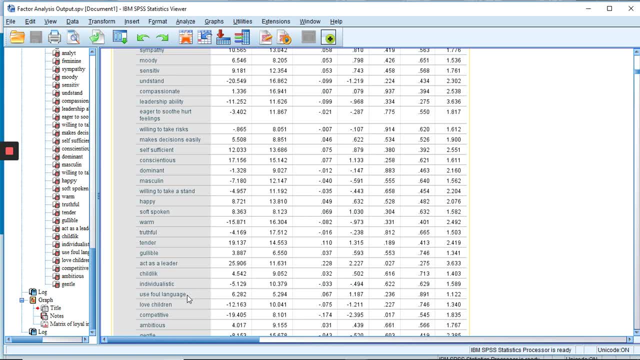 we don't really delete. I mean, I don't know you could, but the concept of deleting a variable is really you have to think of it on a broader level, not just like, oh, hit, delete in the data set, but thinking about your research and thinking about if you're developing a survey. 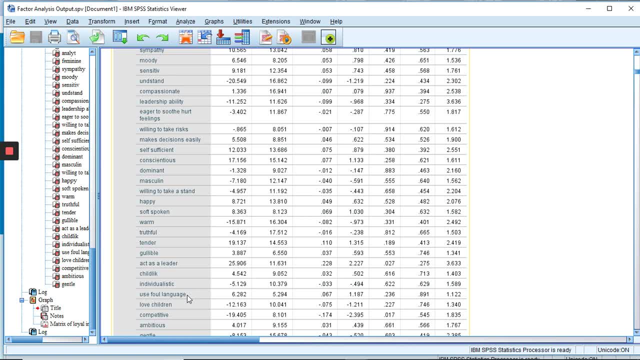 or inventory of some kind. what you're really doing is deleting that item from your survey and then doing the survey again and seeing if that helps. The other thing that you could do if you had some that were kind of on the line, that you wanted to just construct a little bit better. 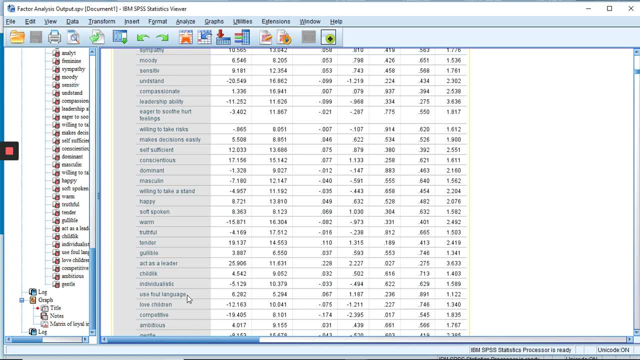 you could add some items to your survey or inventory. that would help kind of boost what you mean there. So you want to be thinking about this in terms of the actual broader aspect of what this is for. I think sometimes I get it's easy to get kind of lost in the weeds on the numbers and trying to figure out what the 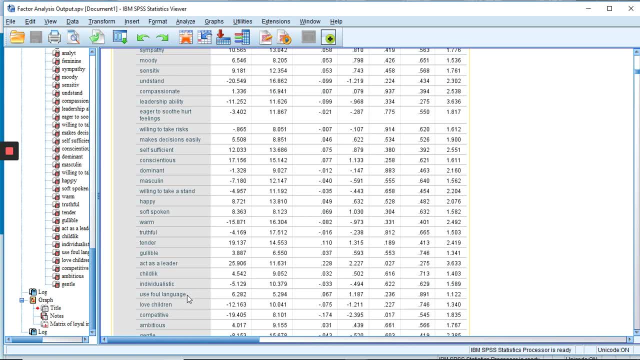 heck like SMC is and where it is on the output, And you forget. you know, imagine yourself as a researcher and you have a tool that you're really trying to develop. then this would be a lot easier than you know just following along in a textbook on some antiquated thing, that's. 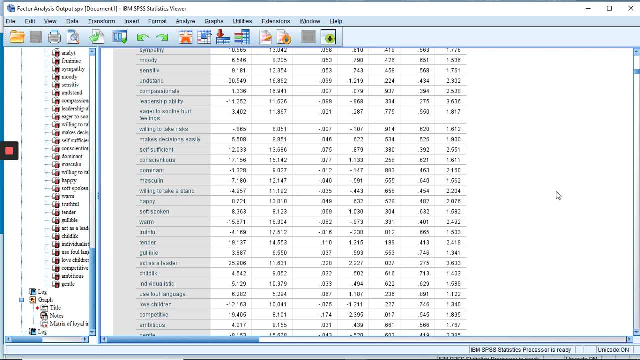 measuring masculinity or whatever- whatever the heck that means nowadays, Right? So you've got some of that you got to think about. Now, the thing about singularity- going back to that- is that the large number of correlations that we have in our correlation- 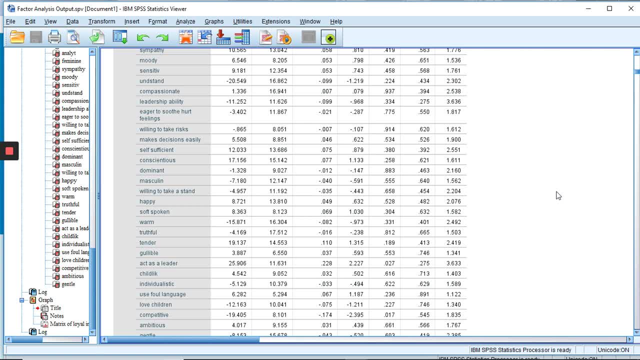 matrix from before. that's a good sign for singularity. When we do our factor analysis, we're going to look for Kaiser's measure of sampling adequacy. We want that to be greater than 0.6, which spoiler alert it will be. 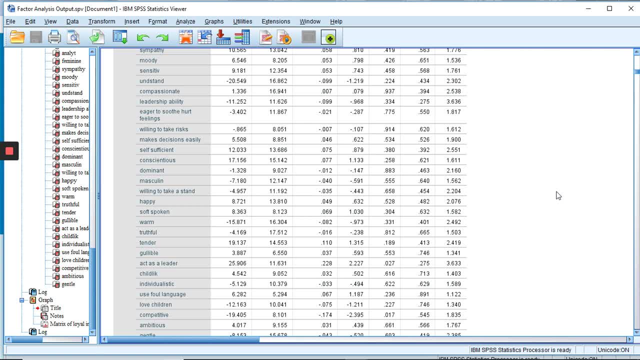 It's going to be 0.849.. So that's good, And we're also going to look for small values in the negative anti-image correlation matrix when we do the factor analysis. So let's get to that And we will first begin with a. we'll go to analyze and it's found here on this dimension. 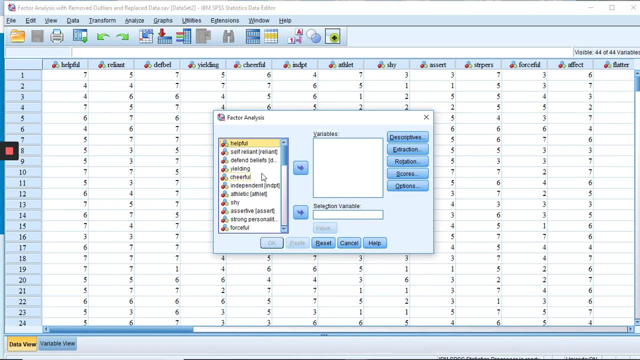 reduction factor. And the first thing we're going to do. well, we want to scoot all of these variables over. Oops, I forgot to hold down shift. That didn't do any good. Well, I selected that one. So hold down shift down. click that one, scoot that over. Now descriptives. 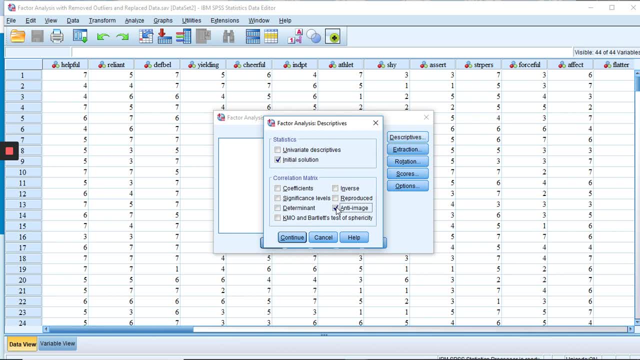 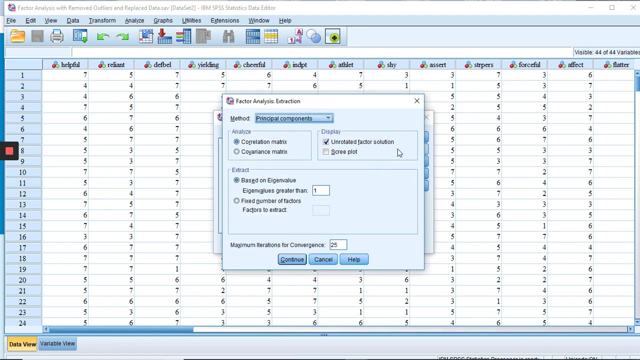 we do want this anti-image one, because that's what we're going to look for. that singularity, as well as the KMO, is the Kaiser's one that we're looking for. So we want that, And that's probably all we need there. And then we want extraction. The first one we're doing is: 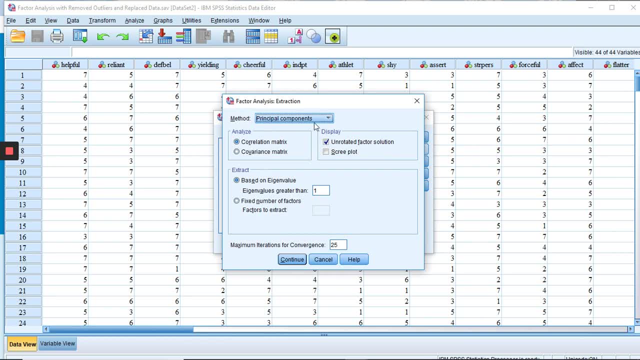 this principal components. That's kind of like a test. We're going to look for that multicollinearity with the eigenvalues And we're going to check for small values in the anti-image correlation matrix. We're going to look at Kaiser's measure And that's what we're going to do. We also want: 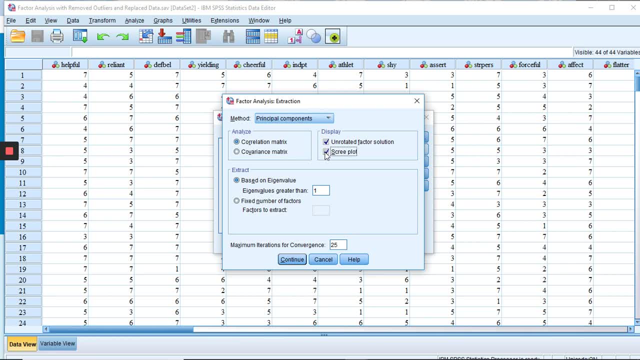 the scree plot. So we're going to look at the KMO And we're going to look at the KMO And we're going to look at the KMO, And that's going to be really helpful for us And we want it right now. 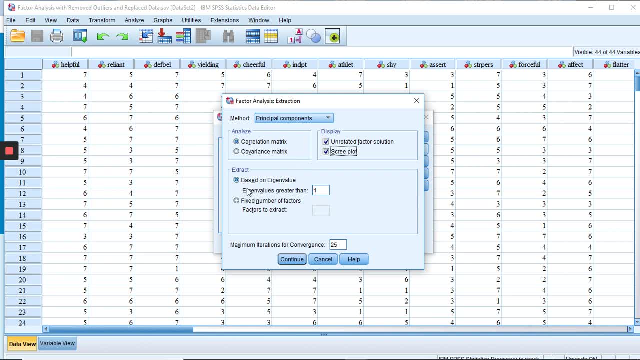 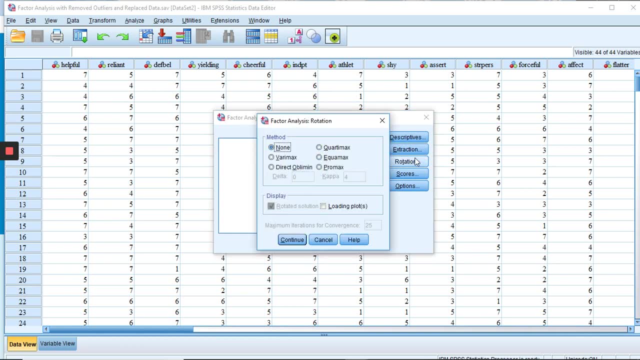 based on eigenvalue, So we're going to keep that there. So click, continue The rotation. right now we are starting off with just a Verimax rotation which is orthogonal, And we can click on loading, continue Scores. Oh, do we need these scores first? Oh, did I save the scores? Let me see. 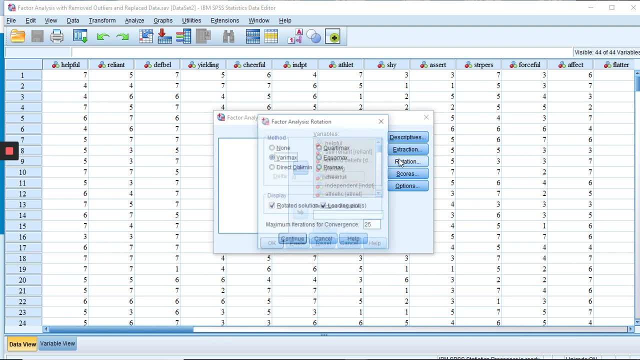 Oh, you know what? Hold on, Now that I'm looking at my notes, the rotation is actually going to be the ProMax for this first one, with a two in that box. Hold on, No, My notes, guys. I need to take better notes. Okay, Rotation Verimax: Yes, We want that first. 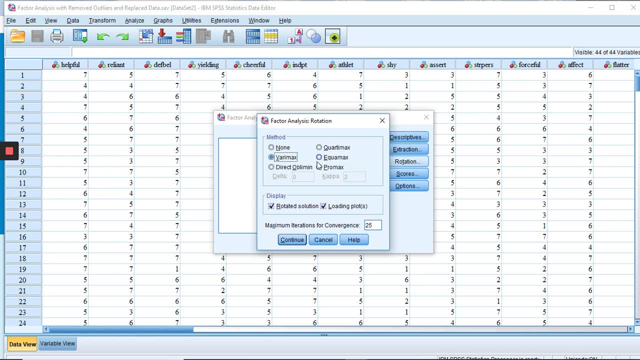 We're going to play around with this. We're going to run this so many times that you're going to be confused too, But then you'll be unconfused at the end. It'll all work out, Trust me. All right, We do want to save the scores, So let's go to scores. save as variables. 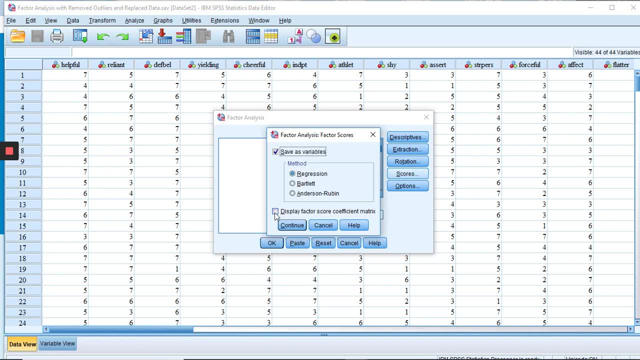 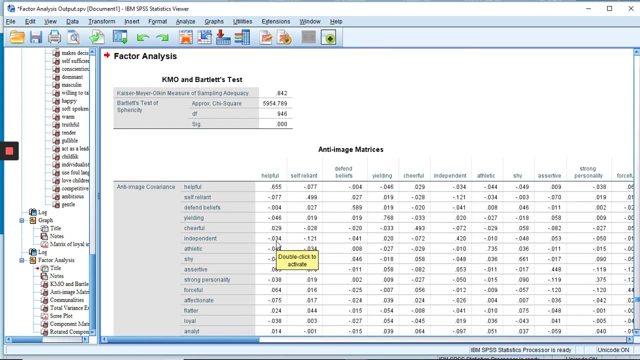 and keep it on the regression. one Display factor: score: coefficient matrix: Sure, Okay, I think that's it. I'm looking carefully at my notes here. Let's go ahead and click okay and wave our magic wands. All right, So here you go, The Kaiser. 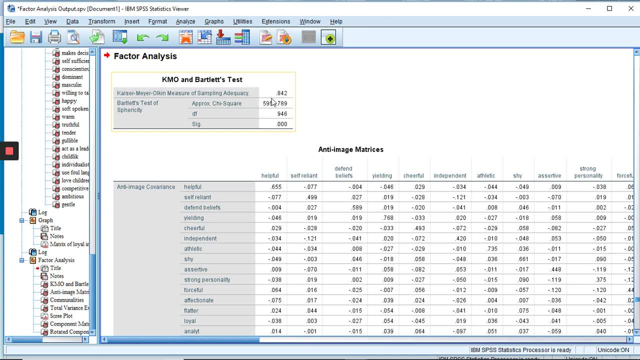 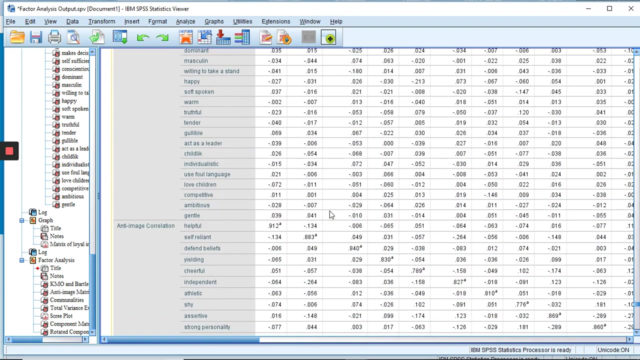 number here that is above 0.6.. So that is really good for singularity. So that's what that will do. It'll help you show. And then here's our anti-image matrix, And the anti-image correlation is what you're looking at for singularity as well, which you want: small values in the 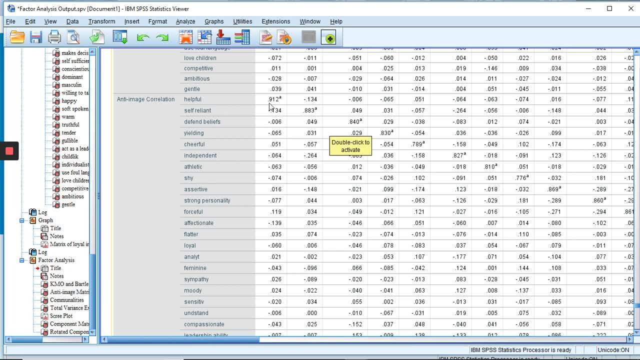 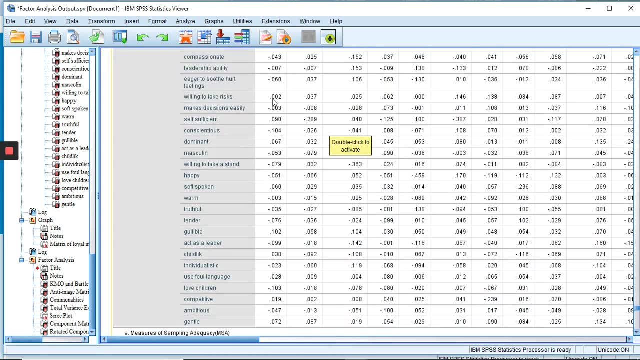 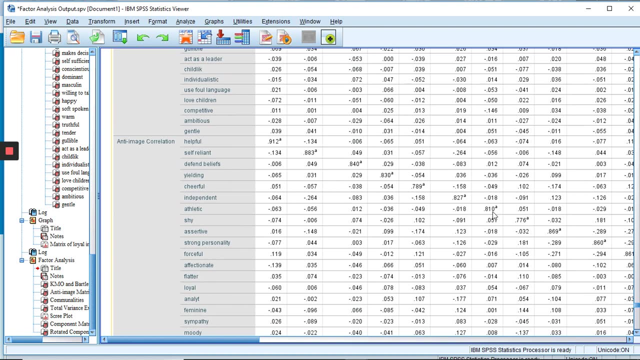 anti-image correlation. It looks like one of them here. this A- let's scoot down here and see what it says for A measures of sampling adequacy. Okay, So that's a really big number, but otherwise it looks like here they kind of flag big ones. 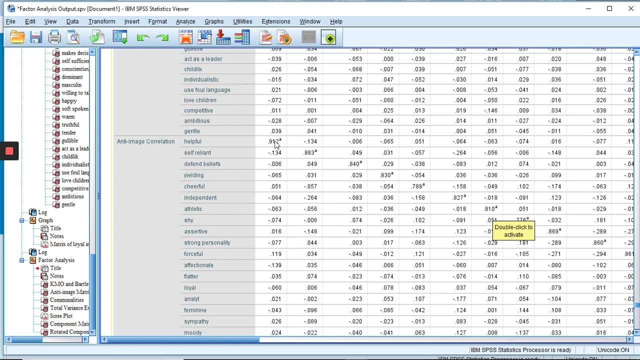 Oh, I see why this is the diagonal, So we can ignore that. So, don't worry, That's helpful with helpful and self-reliant with self-reliant. So yeah, basically all the other ones we're looking at, they look pretty small. They're all 0.0 or 0.1 something, So that's a good sign for. 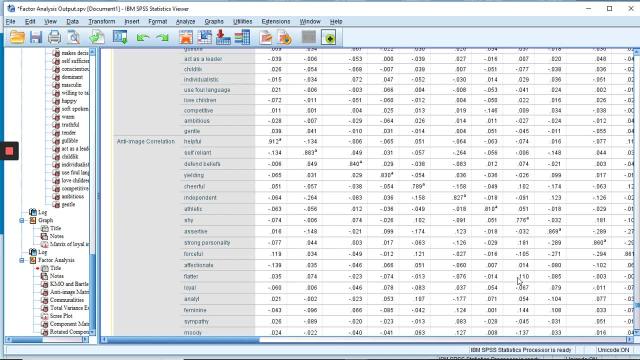 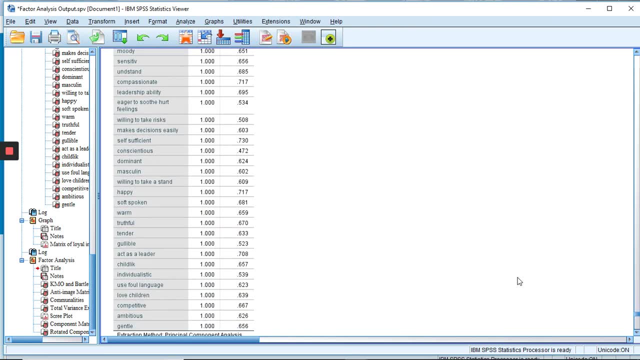 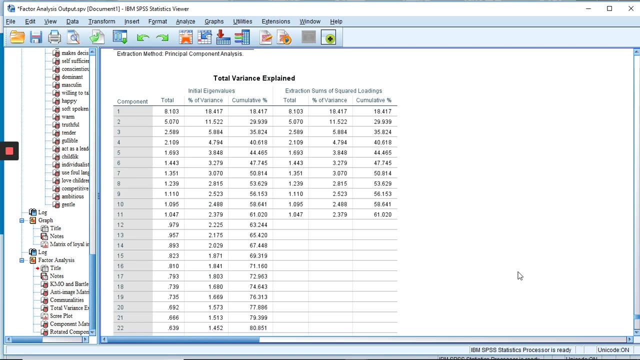 singularity also. Okay. So then here's what we want to look at now for this output. This is going to skip everything, except for this chart here where it says total variance explained. Now, this is in the main analysis section, If you're following along with that checklist, that is number one, the 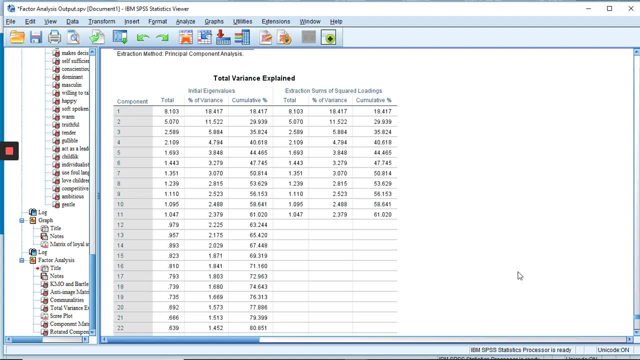 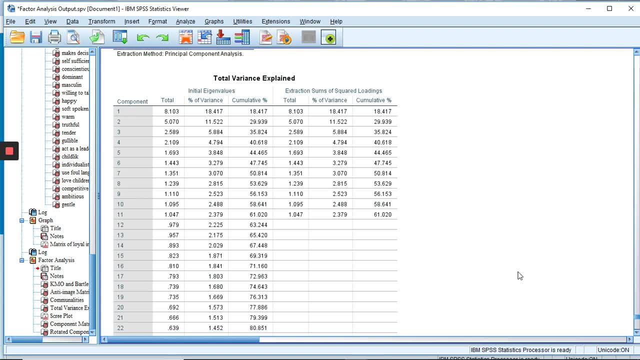 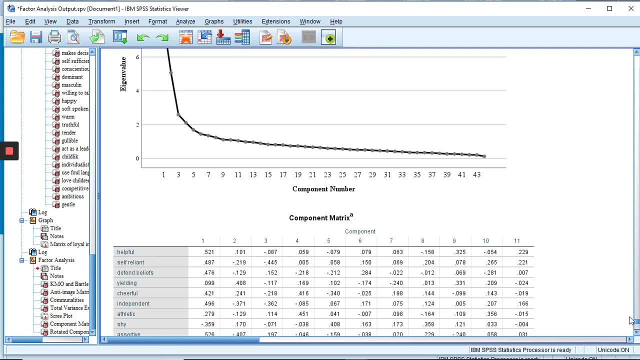 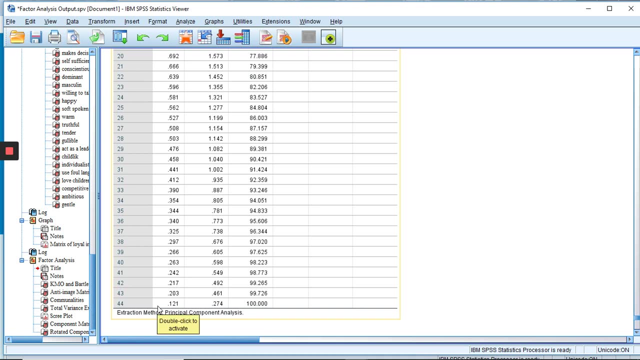 Oh, one more thing we wanted to check on for multicollinearity before we get into the number of factors is the eigenvalues. They all need to be above zero. So, oh dear, Oh my gosh, Sorry guys, My screen Okay, Right down here. This is the lowest eigenvalue: Eigenvalue. 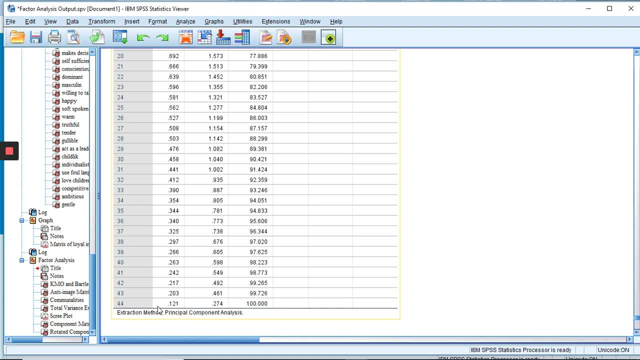 Eigen, I don't know, Somebody needs to tell me the pronunciation in the comments. But it's small, but it's enough above zero, Right, Yeah, So that's also good for multicollinearity, So you can document that. 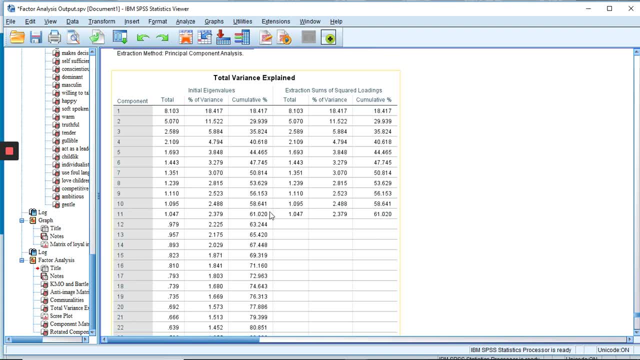 All right. So now we are looking at 11 factors where the eigenvalue is above one, And that's what we would need for it to be considered a factor. But if you imagine that you are conducting a survey and you have 11 different things that your inventory will show you, 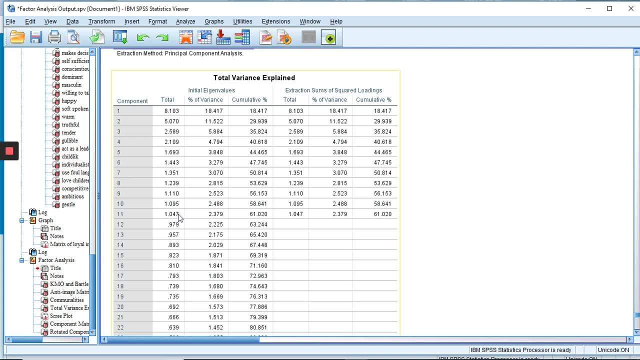 especially on something with only 44 variables. that's kind of a lot. So we're obviously not going to go with 11.. And so you can see here- okay, let's look up at the top- that 8 is really high, 5 is really high. 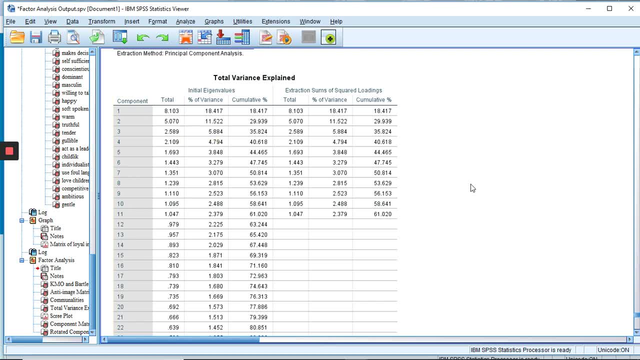 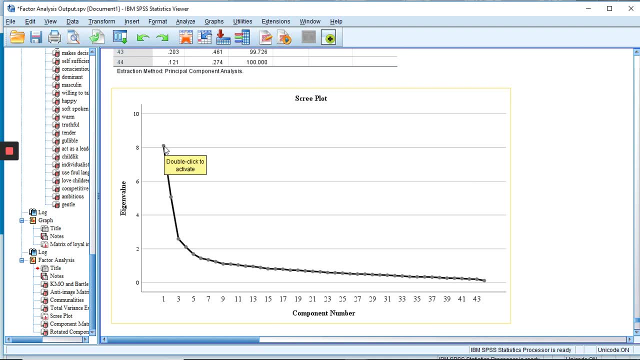 these 2s are really high and then we start kind of dropping off, which is what is displayed here in this lovely scree plot. You see, these are the factors, So it's the eigenvalue here, Factor 1,, factor 2,, factor 3.. 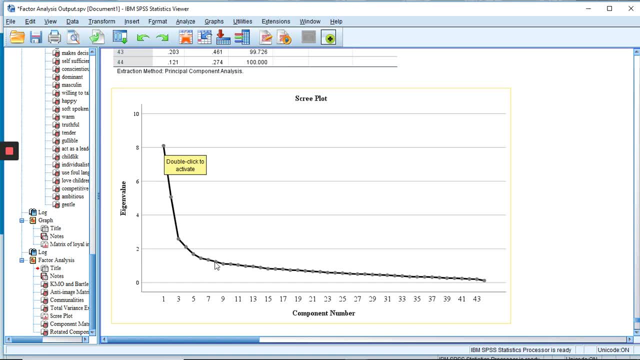 Factor 4,, factor 5, factor 6.. And then it starts kind of flatlining. So, as the book will describe, looks like between 4 and 6 is about right. Somewhere between 4 and 6 factors will be our most accurate. 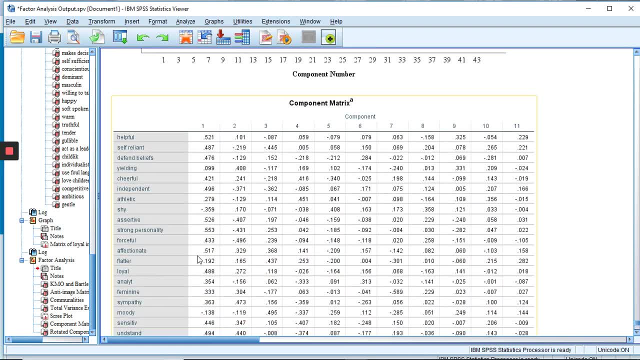 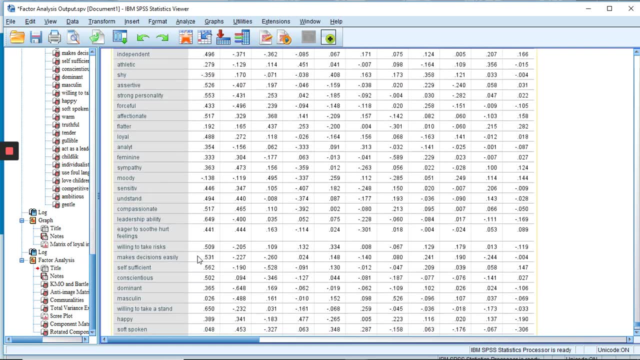 And so that's what we're going to play around with now. We can kind of ignore everything else, because obviously we're not going to choose 11 factors. That was just to kind of give us, you know, a preliminary look at the data. 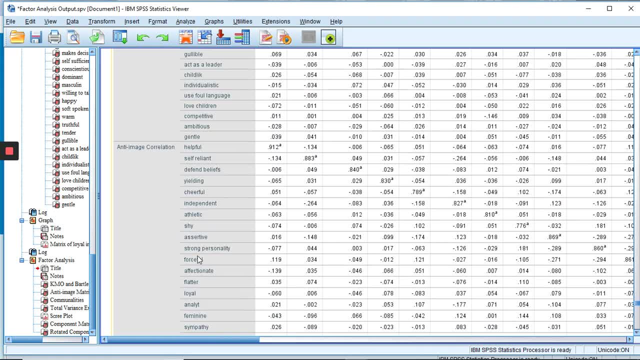 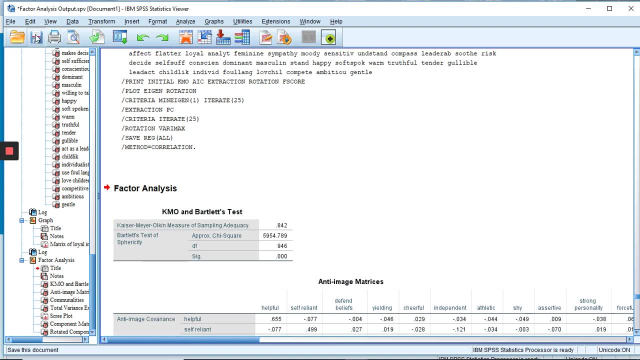 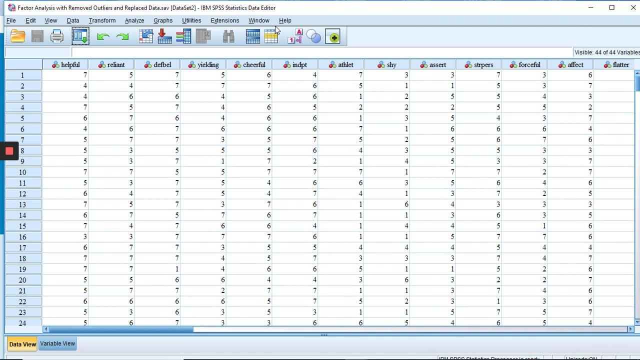 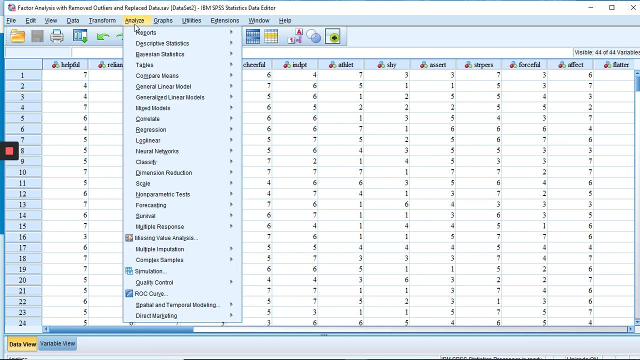 So these, this part of the output is not what you're going to be mentioning in your interpretation. Go ahead and save that and then we will go back here. And now we're going to play, So think of this as fun. And now what we're going to do is go to analyze and dimension reduction factor again, but this time 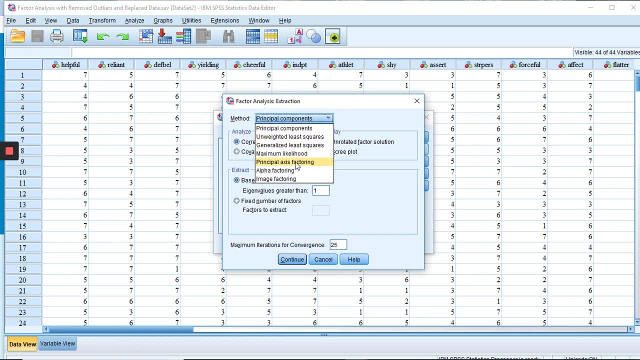 the extraction. what we're going to do is this one called principal axis factoring, which again the book calls principal factoring, And I was a little confused because I wanted to make sure it was the same thing. And so it is, and we already have seen the scree plot now. 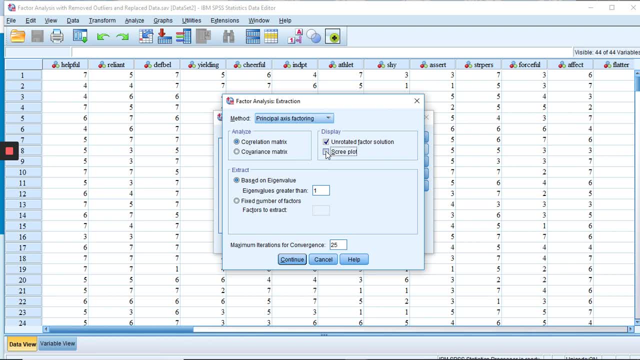 So we probably don't really need that anymore. We know what that's going to look like, And what we want is a fixed number of factors. Let's start with 6.. We'll just go down 6,, 5,, 4, and we're also going to be asking ourselves about the rotation. 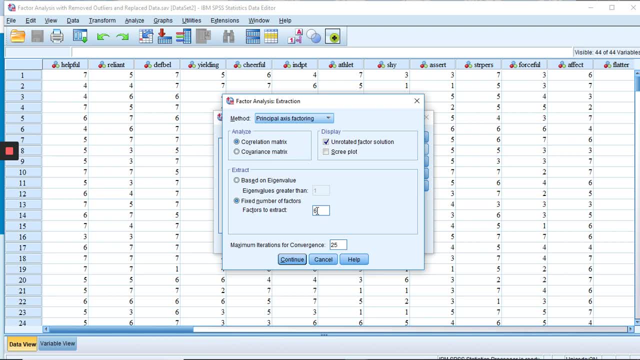 So there's a couple options for rotation and what that basically means The rotation is. best I understand it- is that you're first taking the correlations of all of the variables to see what most highly correlates- and kind of multiple correlations- And then, after you've done that, you try it again. 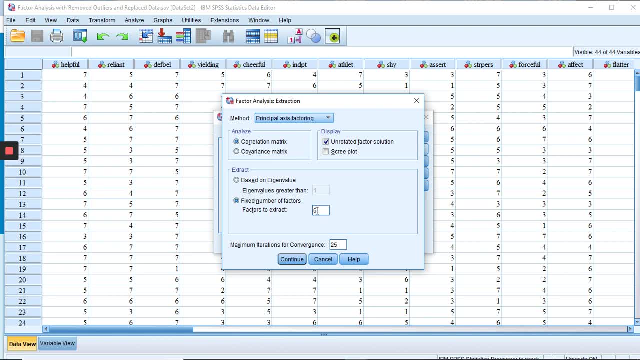 Okay, And then removing that, those correlations, you kind of get the second best correlations and then the third best correlations and the fourth best correlations. So each time you try it again it rotates kind of the axis, And so there's some pictures that kind of show that. 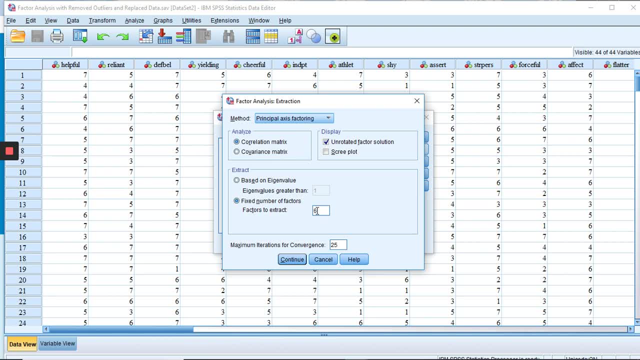 And you have to, I think, understand it three dimensionally, which is hard, even though in the output it does. I just want to give you a little three-dimensional plot. if you check that off, It is a little bit hard to understand, I think. 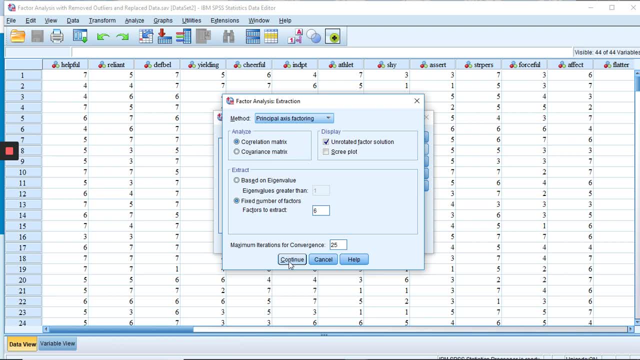 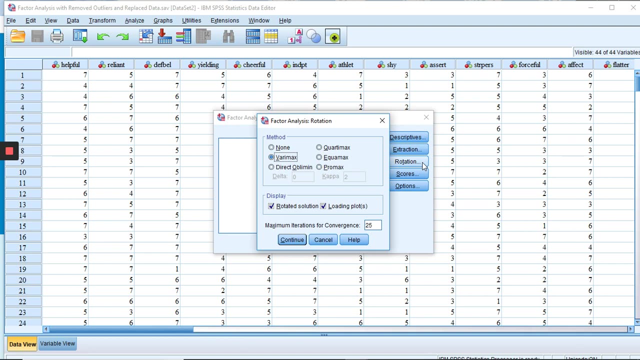 I only barely get it, But it helped me to think about it as, like you know, the first best correlations and then the second best and third best, So click, continue after you've clicked that 6.. And then our rotation. right now we're going to keep doing Veramax while we figure out how many correlations we want to do. 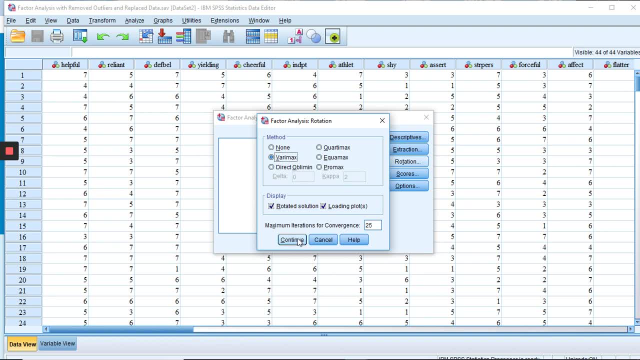 many factors we want. And then, once we decide on the factors, then we can play around with the rotation. So, I know, don't be too disappointed, I'm making you wait on rotation. Um, we all need options now. Okay, Descriptives: Yeah, we don't need any of that. Okay, We don't need the anti. 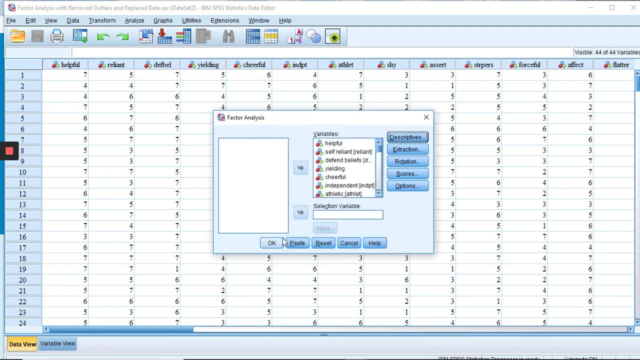 image anymore, so we can get rid of that, just to give give us one less thing to look at. Okay, So here we go. We are trying now with six factors. We're going to see what that says: Click Okay And um. 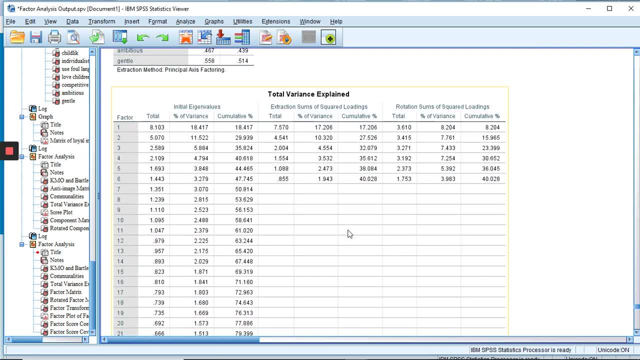 here we are And here are the eigenvalues which these do not change. And I was confused because the book kept saying: look, your eigenvalues are different. And I was like mine aren't. So I don't really understand if I'm doing something wrong or if it's just again a difference in um. 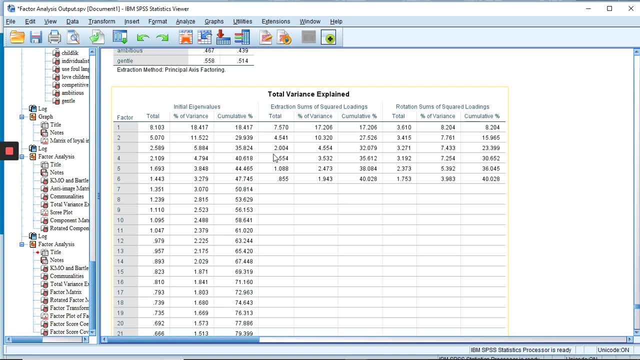 in the um, SPSS versus SAS. But what does kind of change is, yeah, these, these change um the squared of sums, loadings and the rotation sums of squared loading. So that's what we're going to actually pay attention to. The eigenvalues for SPSS should look the same for every single. 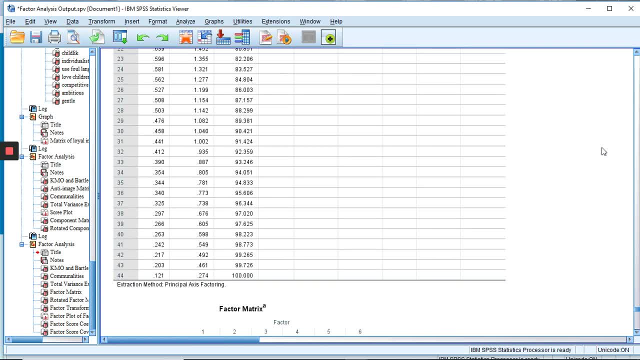 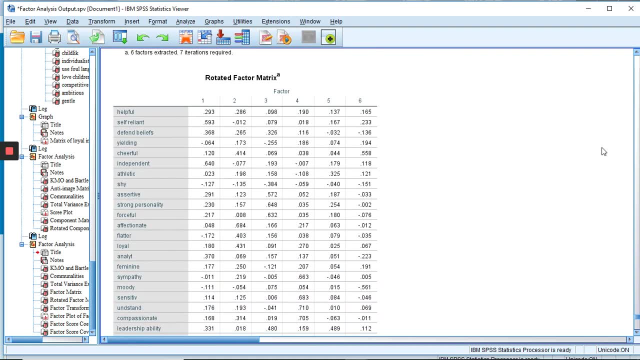 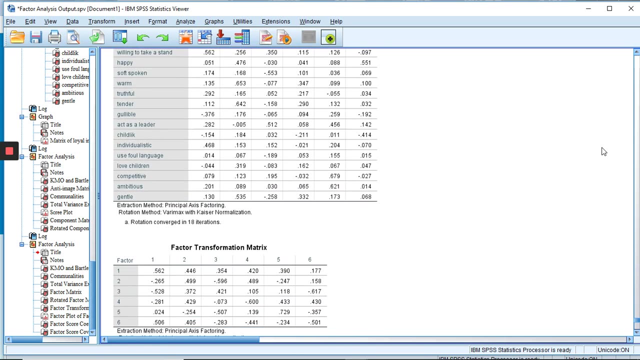 trial, that we do, But really what we're going to look for here is the um rotated factor matrix. Let me see Yep Factor. Okay, Hold on. I just want to make sure. see, this is a three-dimensional thing. 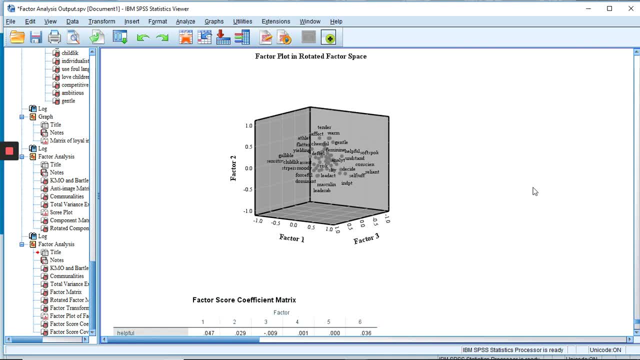 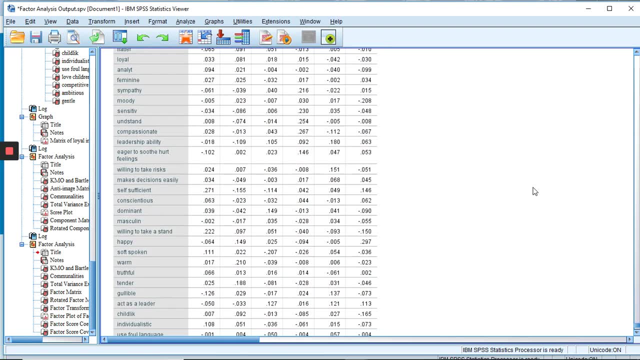 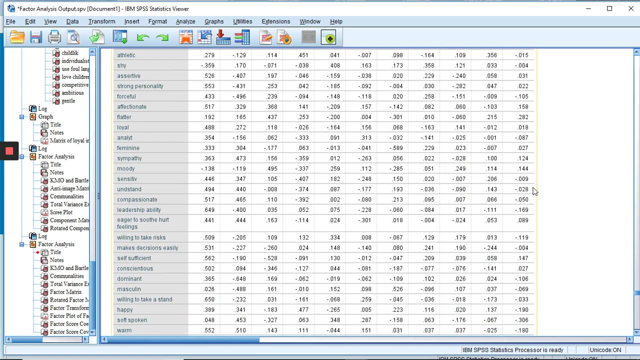 That's kind of cool, but it looks two-dimensional right on a computer screen, So we don't get the full effect of what it looks like, So we have to enter the matrix to understand it. Okay, So let me see here What we do want. Oh, that went all the way up. 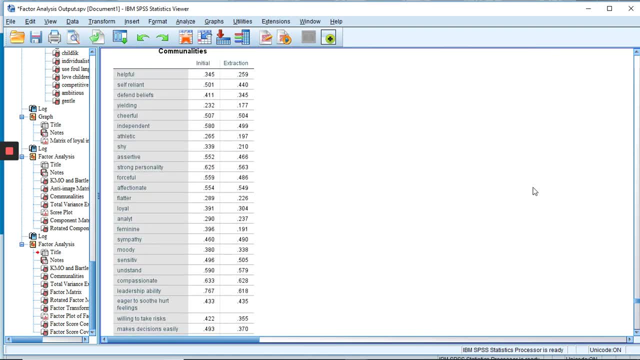 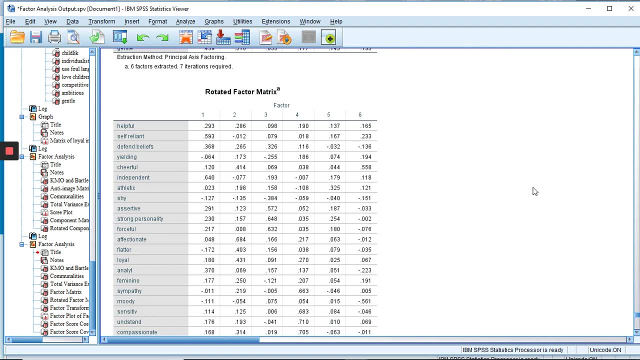 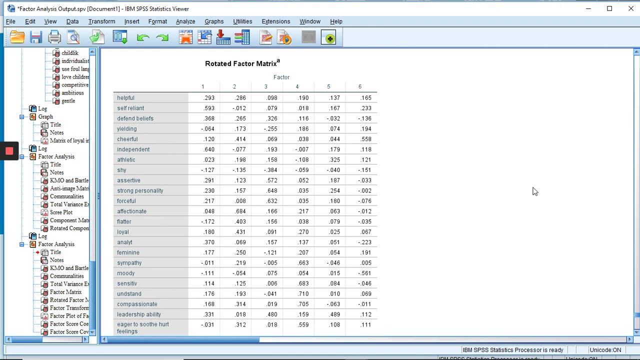 Hmm, We want. no, those are no. okay, We do want this factor matrix, I think the rotated factor matrix. Yes, These are what they refer to as the factor loadings, And the book uses a value of 0.45, which is considered good for um a factor loading, which means how significant that. 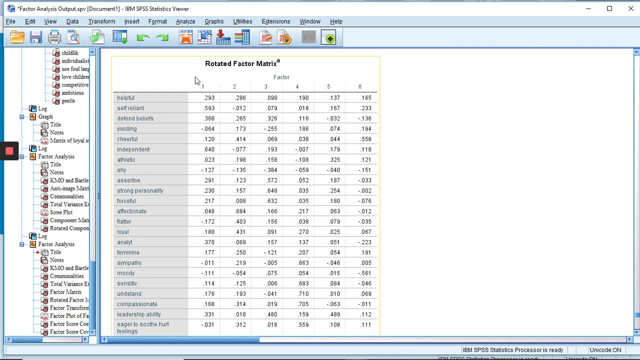 particular variable is. So let's say, for factor one, we're going to use a value of 0.45. And we're going to use a value of 0.45. And we're going to use a value of 0.45. And we're going to use a value of 0.45.. 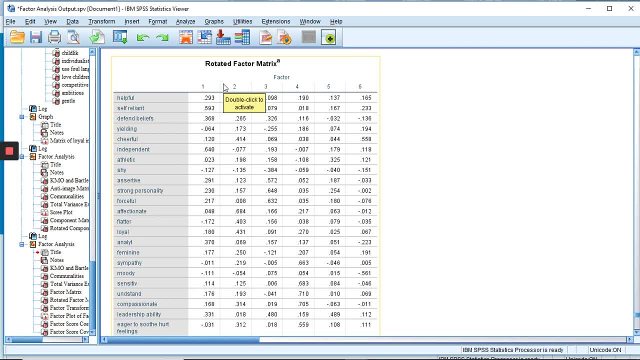 Which we haven't defined yet. We will talk about what the factors are shortly. First we have to figure out how many we're going to count. So here we've got um 0.593.. So for factor one, self-reliant is um one of the higher ones. We go down here um independent 0.64.. 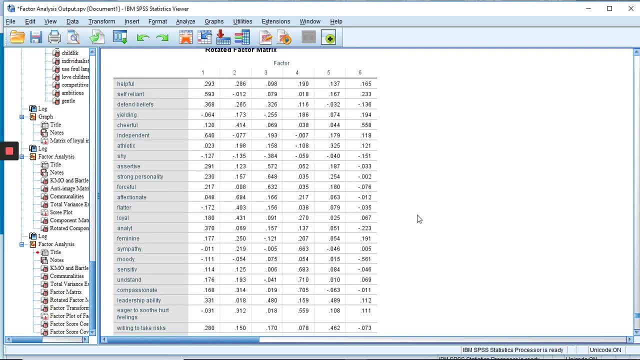 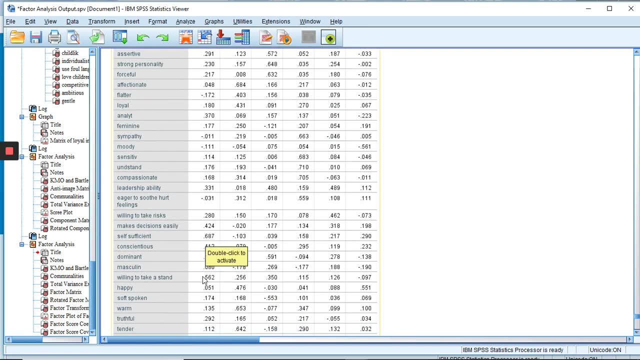 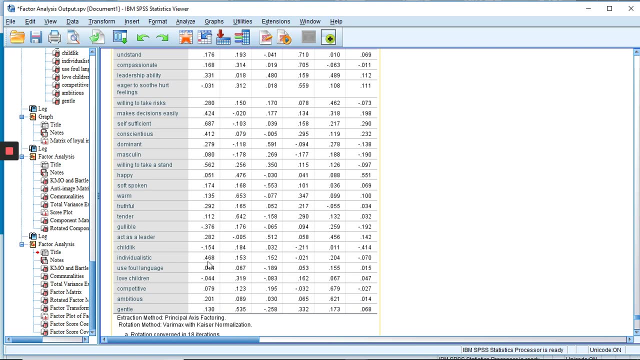 And let's see. So we've got self-reliant, independent. Um, here's another one here, Self-sufficient, willing to take a stand. So you could count them up, but basically any ones that are individualistic here, Okay, So any above 0.45, you could make a little list of them, But right. 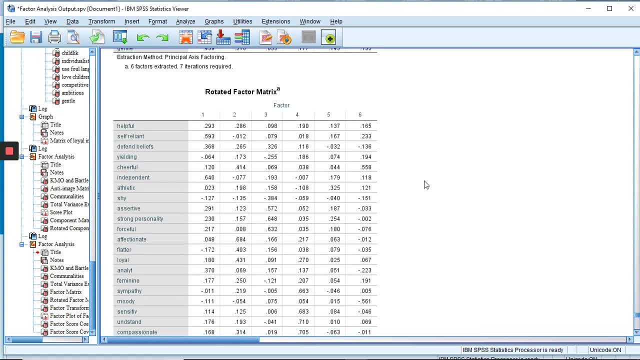 now what we want to look at is we would expect factor one to have a handful at least of values above 0.45.. Otherwise we don't have enough correlations to make this work. But when we get out here to factor five and six, this is where we're going to have a little list of them. So 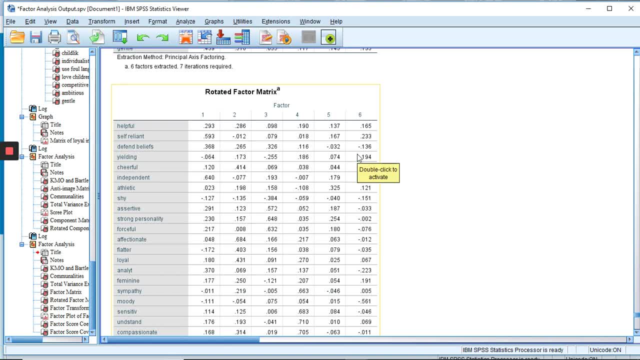 where we want to look for if there's only like a one or two that are above 0.45, then it's not a great factor, because if it's just telling us one variable, it's not really grouping them Right. So we have, let's count on factor six. We have one above 0.45, and I'm just going to scroll down. 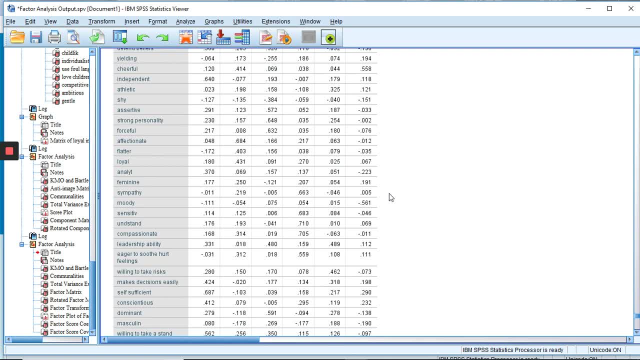 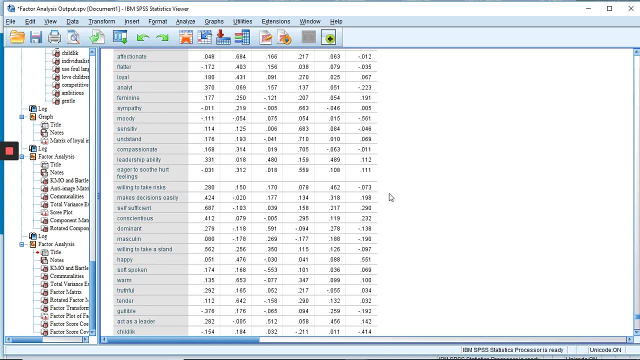 and kind of be looking And negatives, by the way, are low, lower, you know. so those are the ones that we're going to be looking at. So we're going to look at. you know we're going to look at. you know we're going to look at. you know we're going to look at. 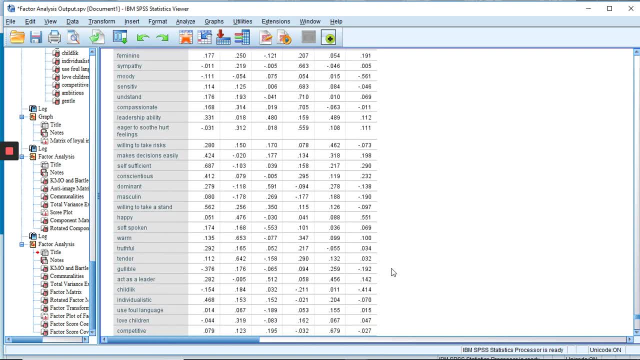 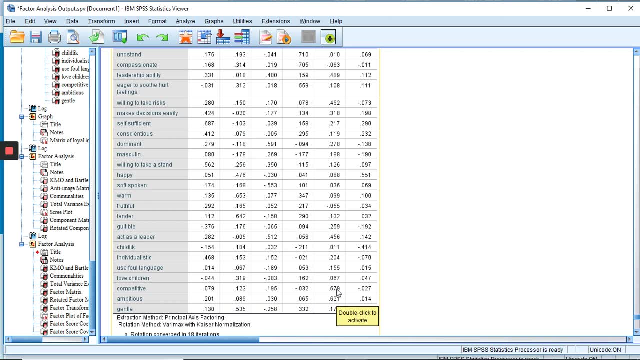 those wouldn't count. So that's two. Happy is another one, So we have two on that. We have two here on factor five, three, four, five, Okay, So that so, but we have one with only two on it. And 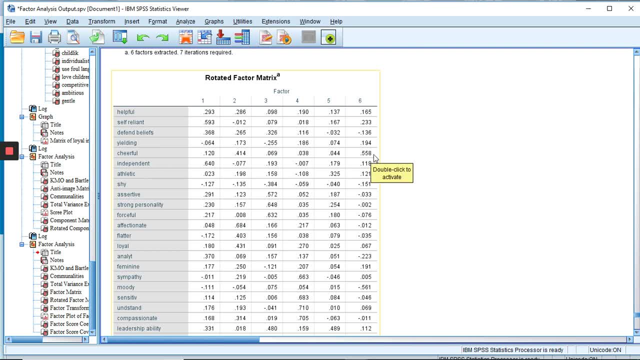 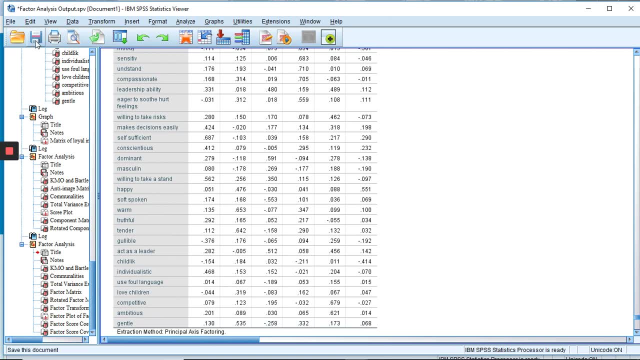 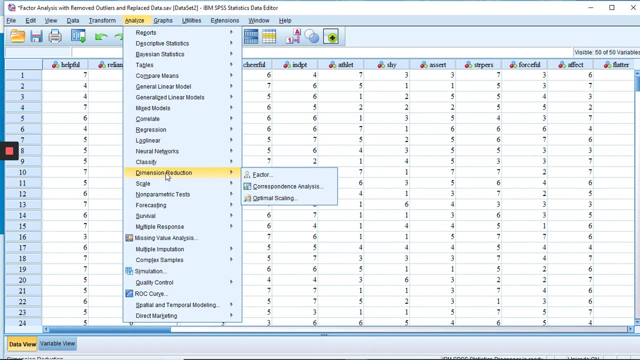 so that, oh, actually, maybe it has three. Yes, I, I might've counted wrong. So that's our first attempt. Now let's try it with only five factors and see if that improves anything. Analyze, dimension, reduction factor. Everything is the same except in the extraction. We're changing that number to five. 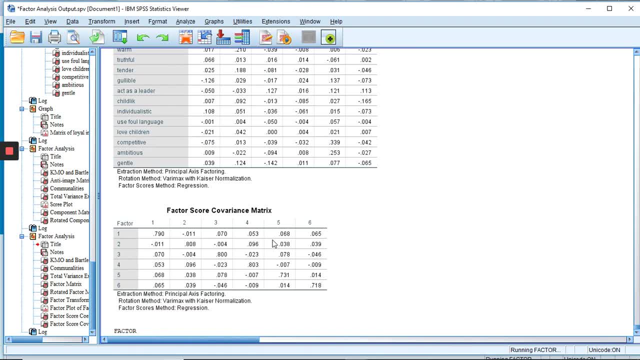 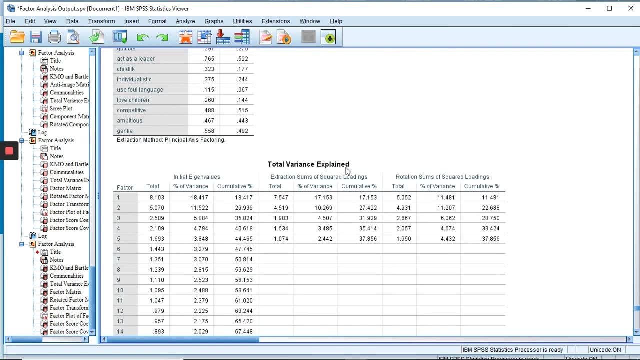 and continue. Here we go again. So let's go down here. See this, Bartlett. I mean, the Kaiser number is not changing. So that is is what it is, All right. So here we see that there is a difference. 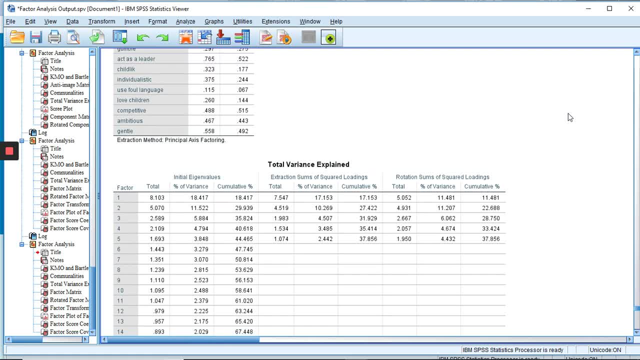 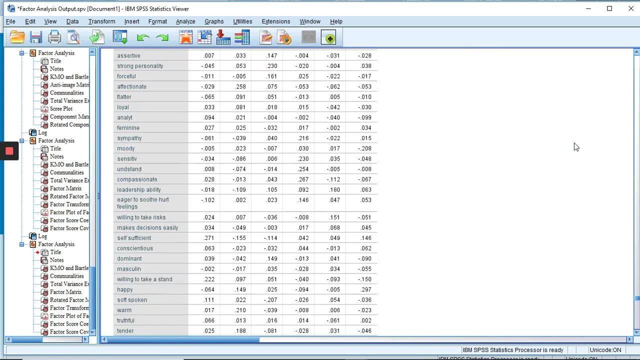 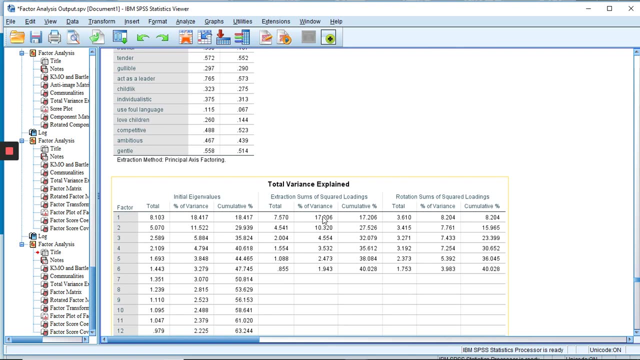 in the percent of variance. Let's compare that with what we had before. Let's see 17 on factor one. it's 17% of variance, And up on our other six factor one. no, that is the same. Ah, trying to think of. I don't understand why they kept saying that. 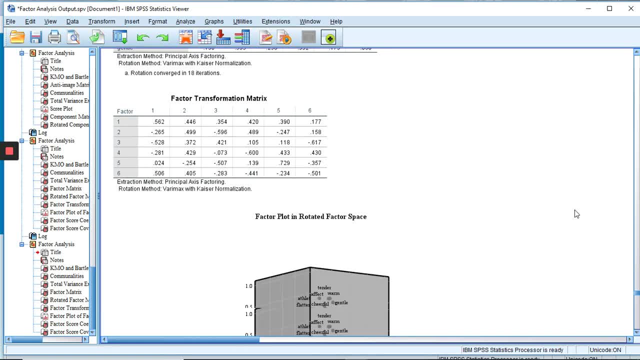 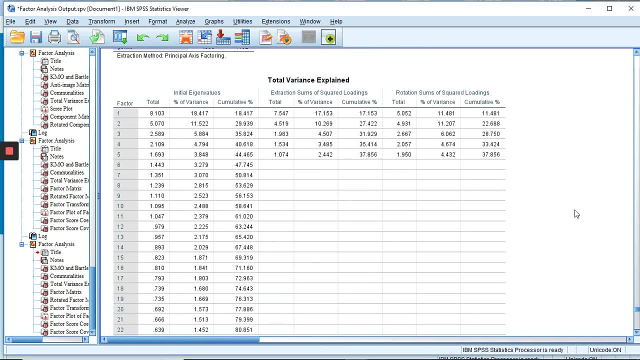 the eigenvalues were different. So I thought maybe that was my clue. but no, it isn't. So it does look like some of these differences. some of these are different. I really disliked this assignment for the output and how complicated they are to kind of like go through because you've 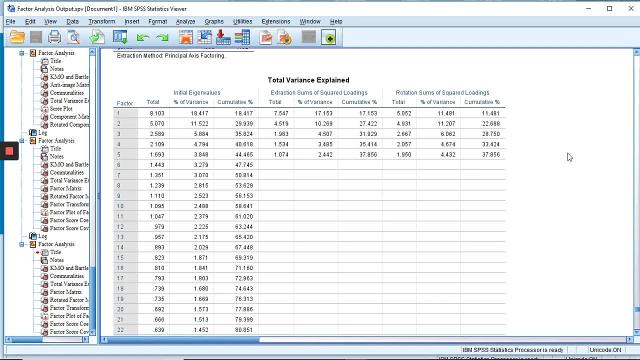 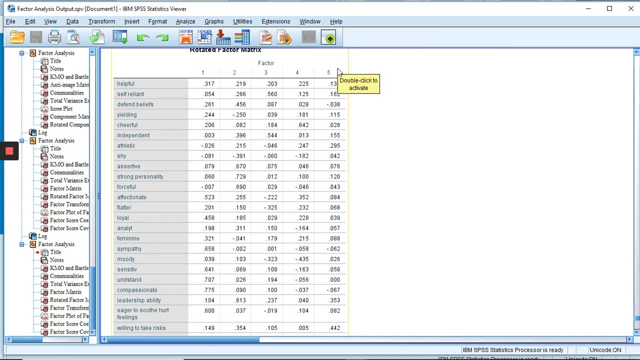 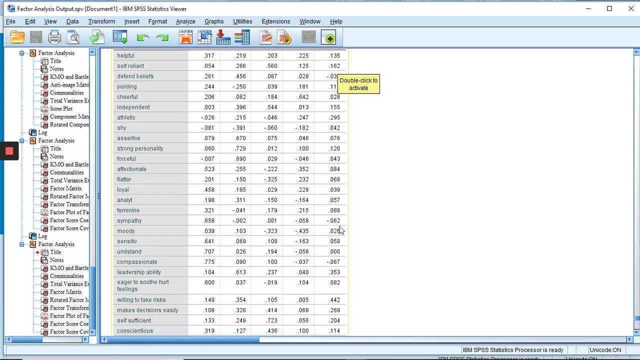 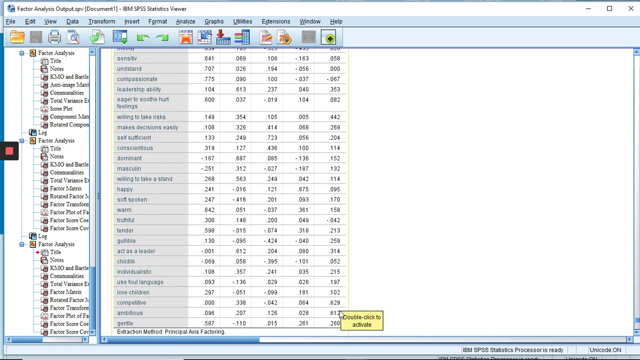 got 44 of everything in every chart. Um, so let's go down and look at just the, the rotated factor matrix, and see, all right, just on factor five here let's see how many variables there are, How many variables are above 0.4, sorry, 0.45, looking for looks like just two here, So again. 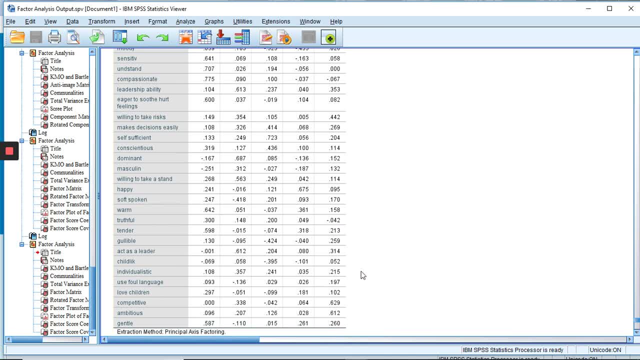 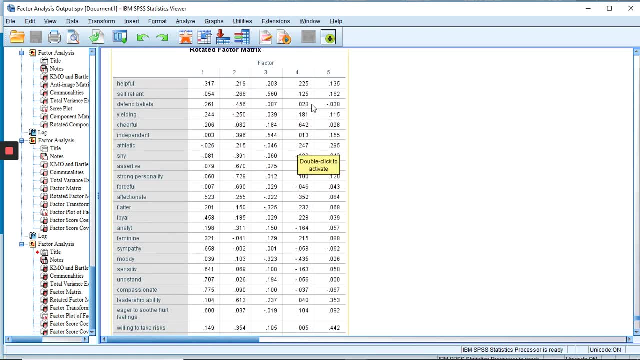 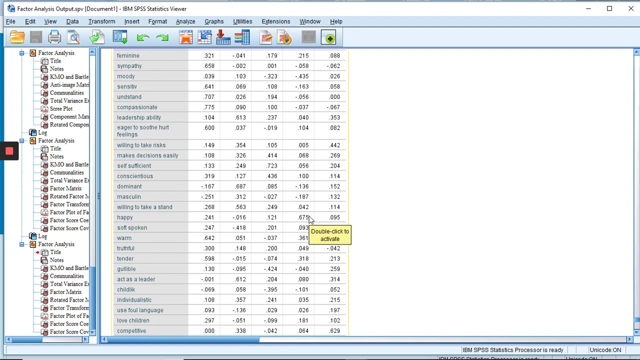 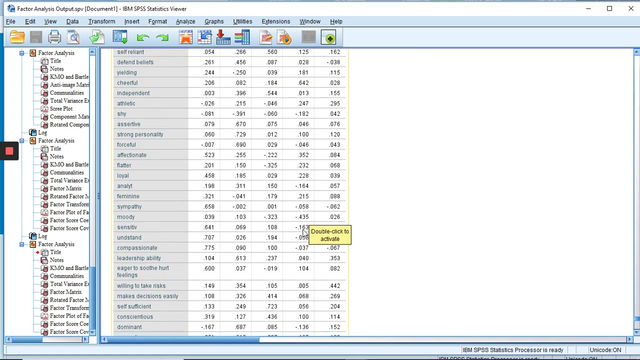 we've got a variable, a factor, with just two on it, unless I missed one. It's not great. And again, you could look at um factor four here. Um, there's one, I think, that only has one above 0.45.. So that's oh. maybe it's two, right there. 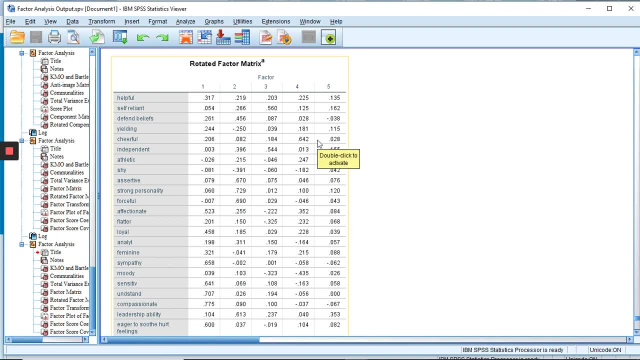 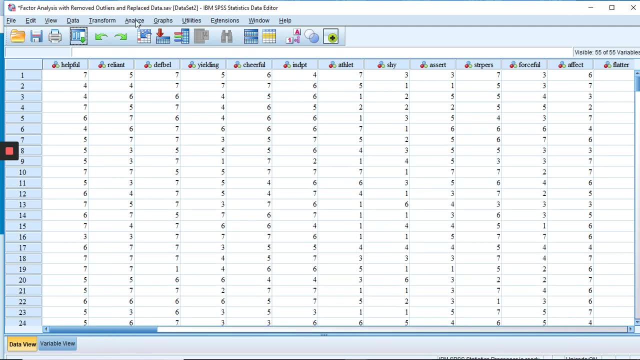 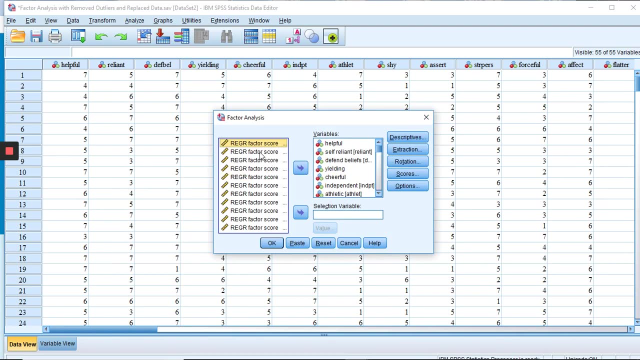 but still that's a couple with only two on it, And we really want to avoid any that have like just one or two. So let's try it with um four and see if that improves things a little bit. So one more time and we are going. it's saving the factor score. 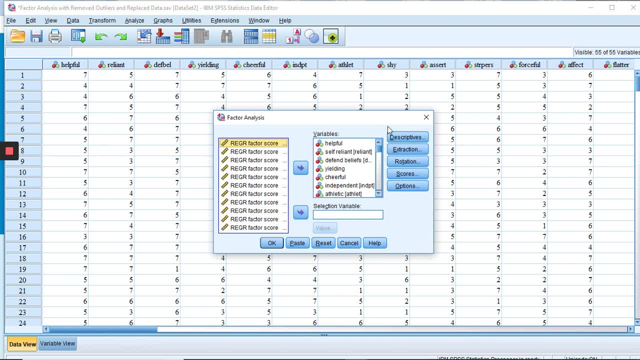 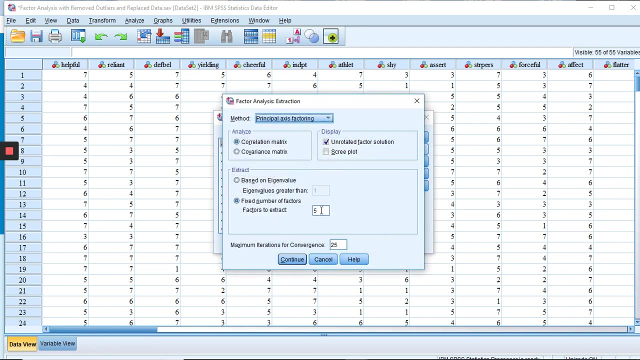 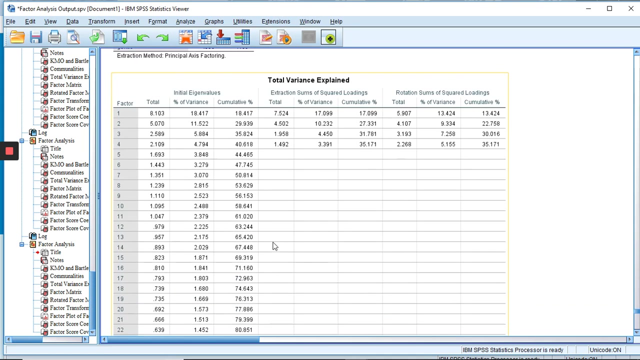 It's every time, by the way. So, um, we don't have to do that, Let's, let's undo that. Okay, All right. Um, so now we are doing extraction four and let's see here. All right, Let's scoot all the way down to this change, No see. 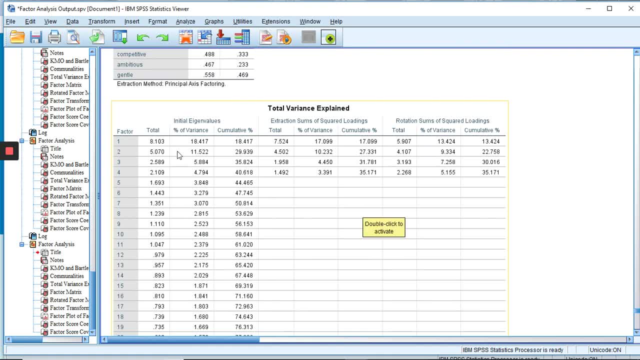 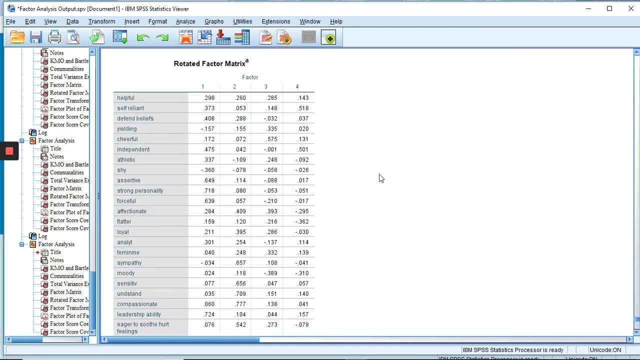 so this is still the same? I don't get that. And your eigenvalues are still the same, So I don't understand what the book's talking about there. All right, Rotated factor matrix. Look at these factor loadings and here we go. All right, 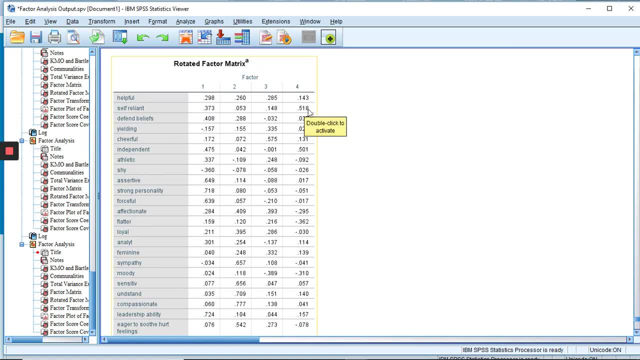 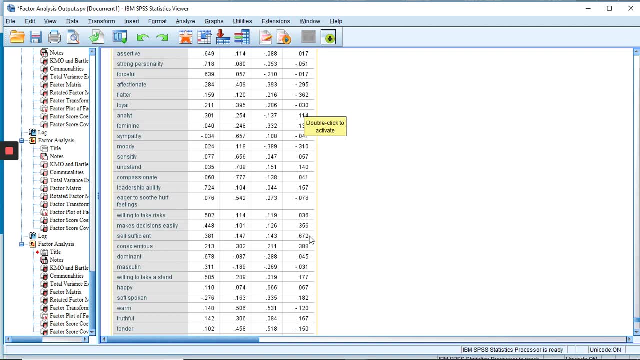 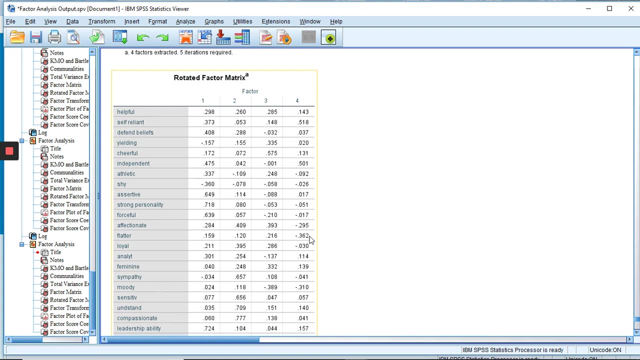 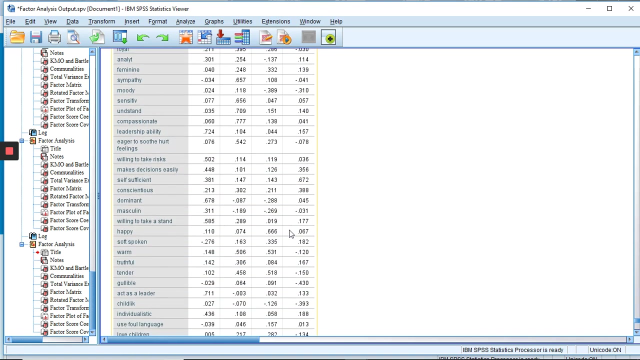 So factor four would theoretically be the worst. We've got one, two, three, three variables on that factor, which isn't great, but it's better because we had the other ones. it only had two And this one. factor three: we've got one, um, two, three. oops, two, three. 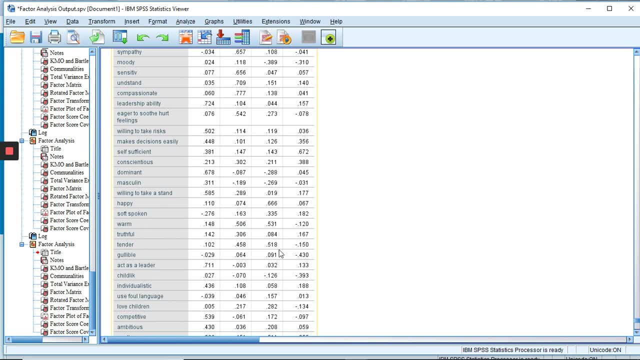 There's more than that. It's hard to scroll and look at the same time, but I will. I'll spoiler alert here: um, when we look at the nature of the factors. I wrote it down. So there are actually five that are above 0.45, um on this, and it should be gentle. 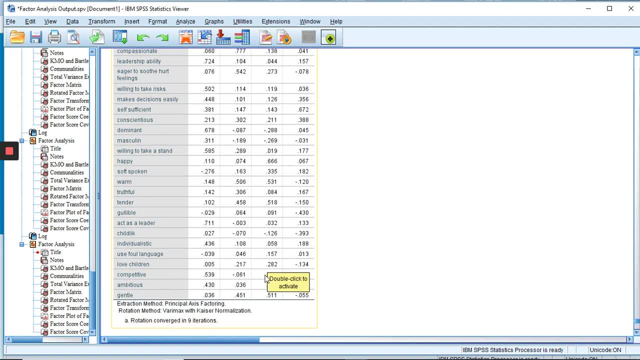 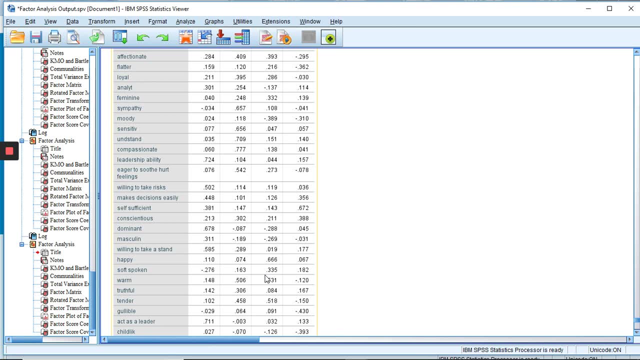 tender. let me see where it was: gentle, gentle, tender, happy, warm and cheerful, And so that's pretty good. We've got five on that one, three on the next one, And uh, I'll just tell you also that, uh, we've got five on that one, three on the next one, And uh, I'll just 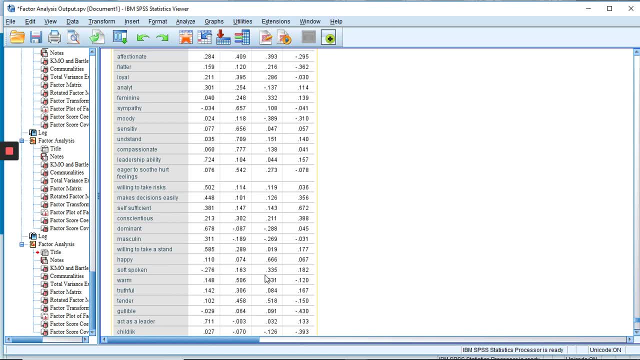 tell you also that there's six on factor two and there's 12 on factor one. So this is where we would kind of just show this and describe that if you were writing this up um explaining what you did, you would just kind of say: you know um with six factors, there was um at least one or 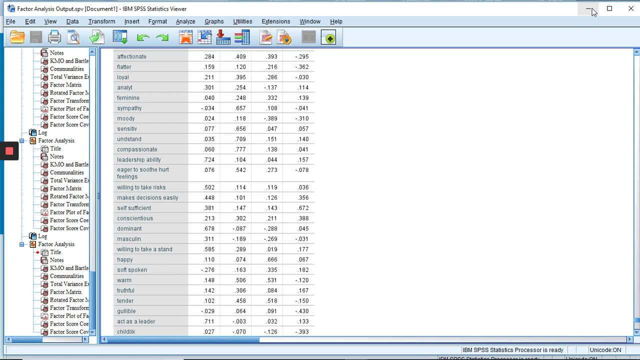 two factors that only had one or two variables And also same with extracting five, four. now our number is um three variables for that factor. So that is kind of our answer, that we want four factors And really if we go back and look at the eigenvalues we will see that four factors here is. 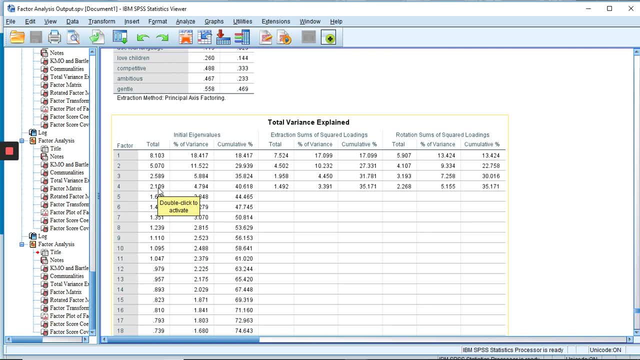 eigenvalues above two And that's, you know, a good cutoff, because there's a kind of big jump here between four and five. So that's kind of our decision to to figure that that's the best fit for the data. So now we have to figure out, okay, what um is, what are the factors? Because what we're 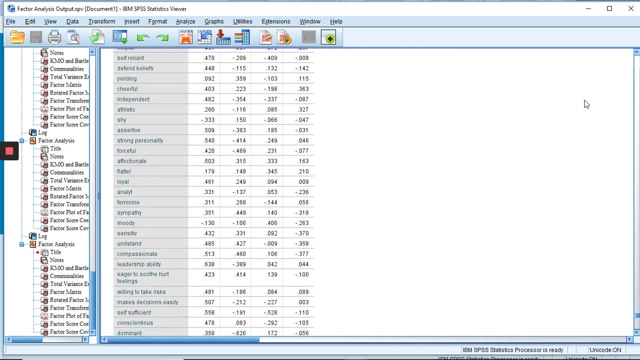 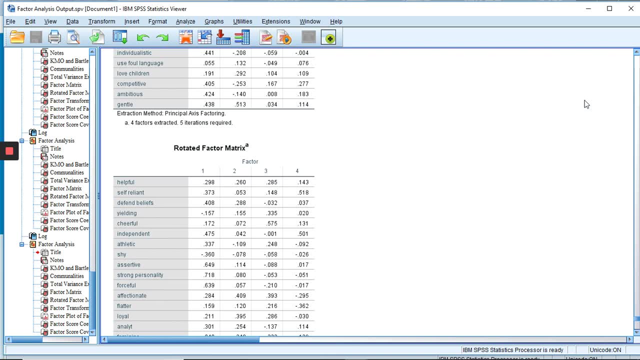 trying to do is group the variables into some kind of category. It's really like creating a construct And, theoretically, if you had designed a survey to measure a certain thing, you'd kind of hope that the factors reflect the thing that you're trying to create, right? So, um, you'll. 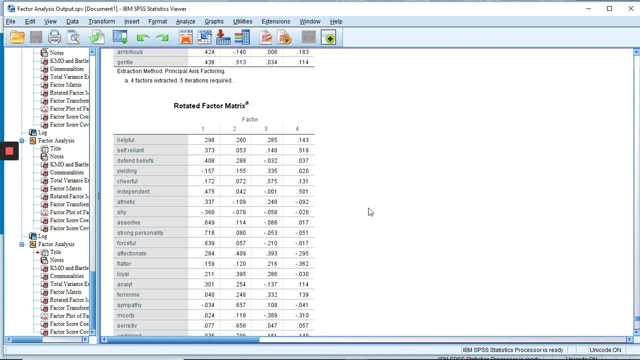 have to look through the rotated factor matrix for all the factor loadings, but I have it written down here And so basically, factor one, the um. the variables are independent, assertive, strong personality, forceful leadership ability, willing to take risks, make decisions easily dominant, willing to take a stand, act as a 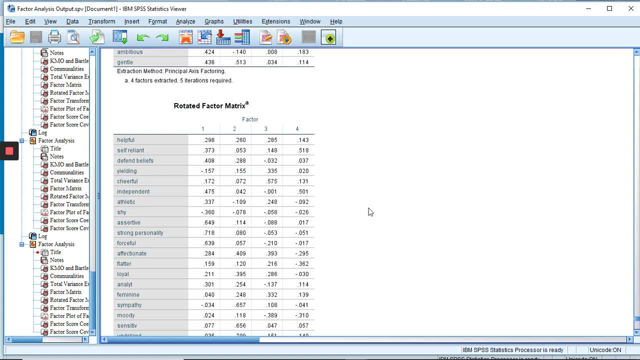 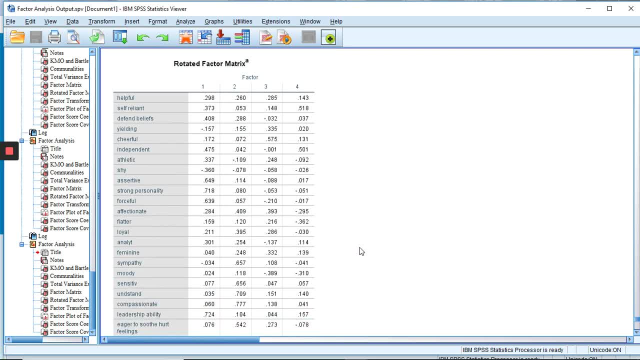 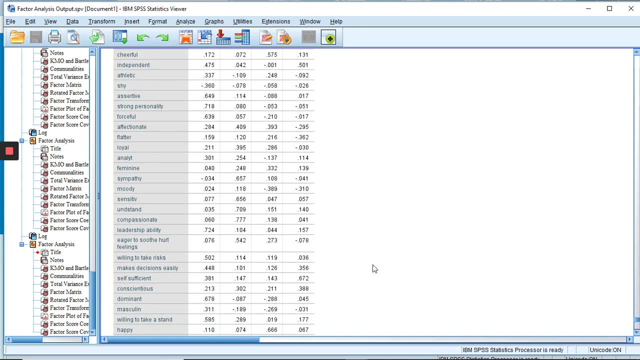 you want to look at um. when you're looking at the nature of the factors, you want to look for any values that are small or negative And that would indicate kind of the opposite of this um factor description. So okay, If you're thinking dominance, assertive leadership, something along- 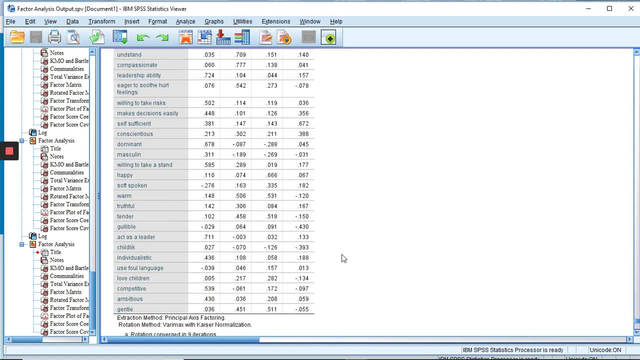 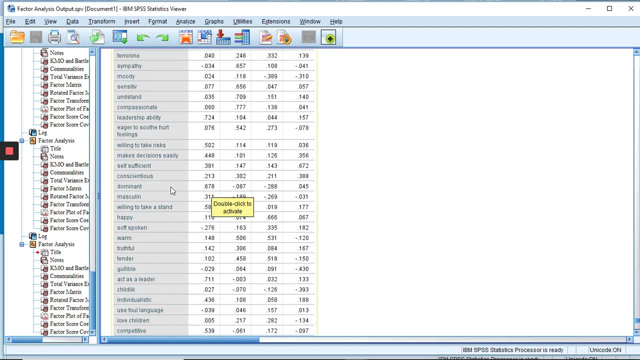 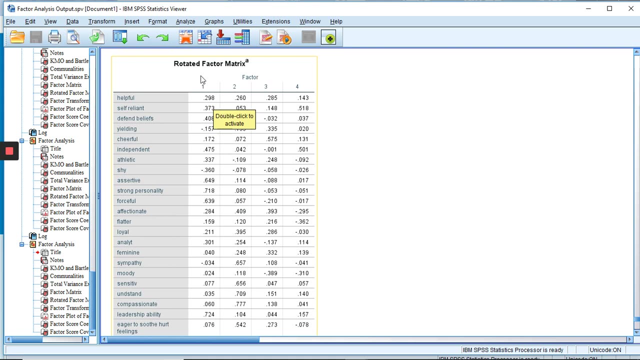 those lines and you definitely not something here. well, negative 0.276 is one of the lowest ones. You're not soft spoken And I know shy was another one: Negative 0.36.. You're not shy. So when you think about what to name this factor, 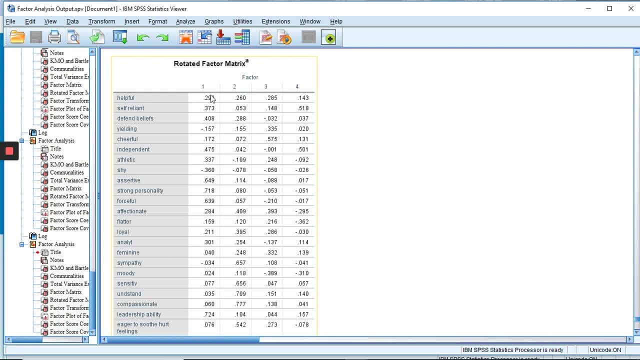 you, you want to kind of consider some theoretical basis for that and say: okay, if you're all these things that are above 0.45, and then you're not these things that are like negative down here, then what are you Right? And so that's how you begin to determine the. 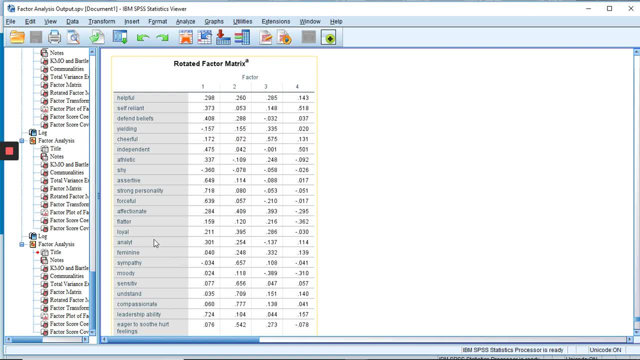 nature of the factor. And so, um, you would really want to probably make a chart that shows um, the, uh, the factor loadings, Um, and what I did. I did make a chart and I put them similar to how the. 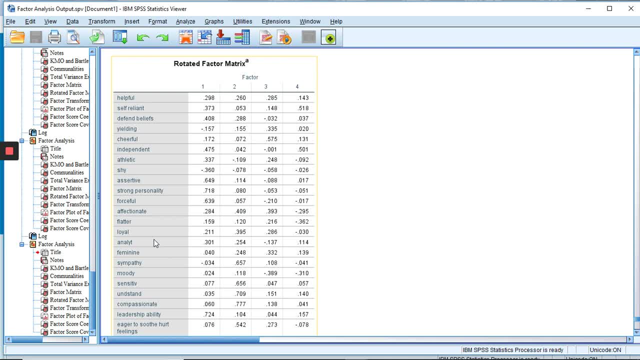 book had it the put the strongest ones at the top and then kind of work your way down, And so, um, that's what I did. And so for the second factor, um, the ones that are above 0.45. 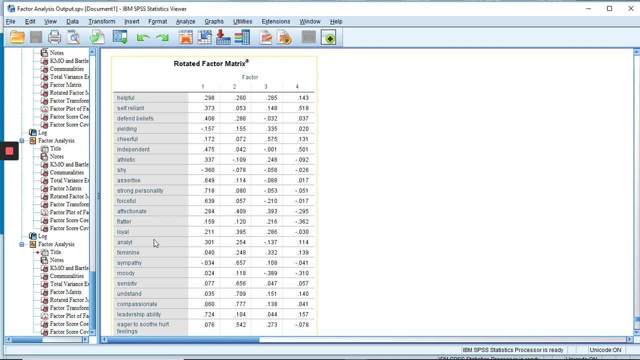 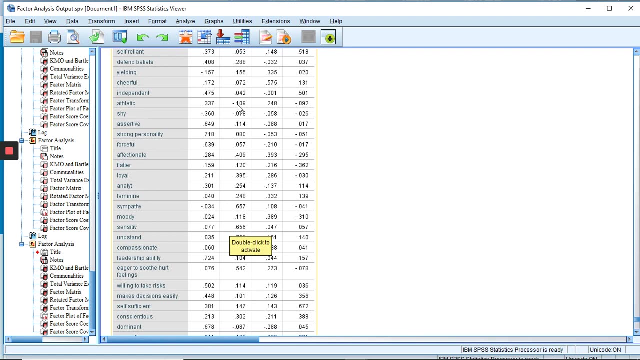 are sympathy, sensitive, understanding, compassionate, eager to soothe hurt feelings and gentle. And so, if you think about that and let's look at some of the negative ones, there's a negative 0.1 there- athletic- but let's see if there's any lower than that. 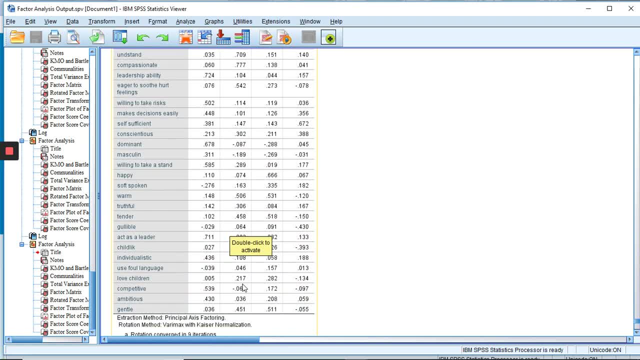 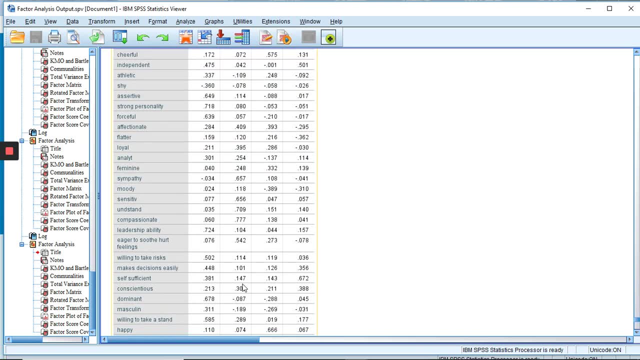 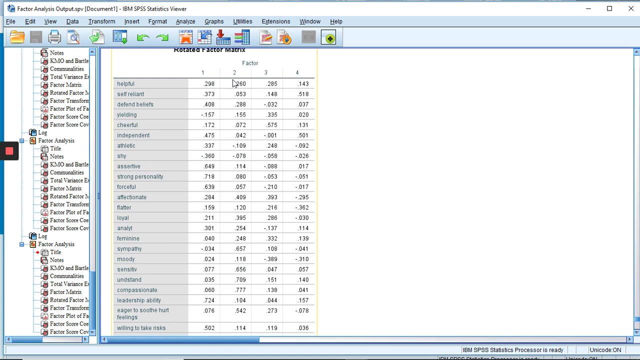 Negative, 0.189, masculine. So, okay, What? what would it mean to be, you know, sensitive and understanding? I think they? they phrased, the book called it empathy, I think I called it compassion. Um, so, factor three, um, the ones that are above 0.45 are gentle. 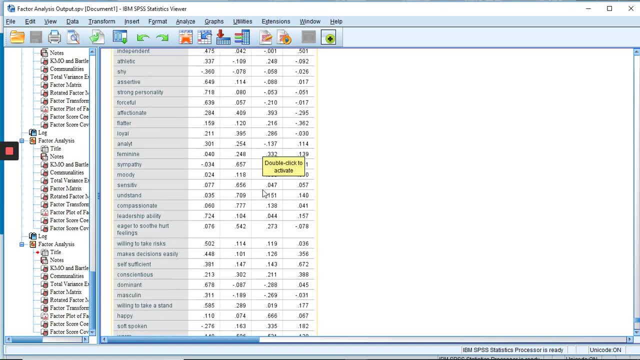 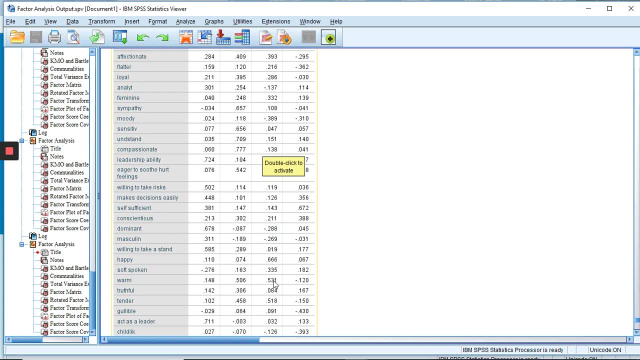 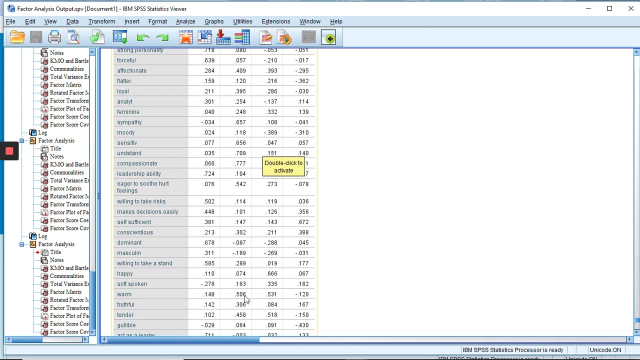 and I wonder: let me look down, They had warm also, but oh yeah, I did have warm. Okay, Where did they? oh, they had a warm showing up on factor two. Let me see warm. Okay, So I missed that one. 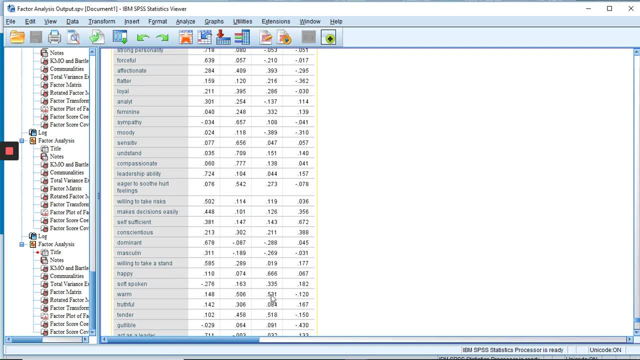 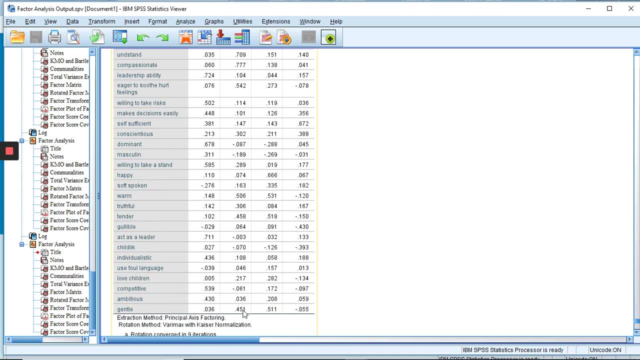 So notice that warm is on two is gentle. Okay, Yeah, Gentle is on two also. So this will relate to the complexity of the factors, which is one of the kind of like additional analysis you can do, And what that basically means is if there's any variables that are above 0.45 on two. 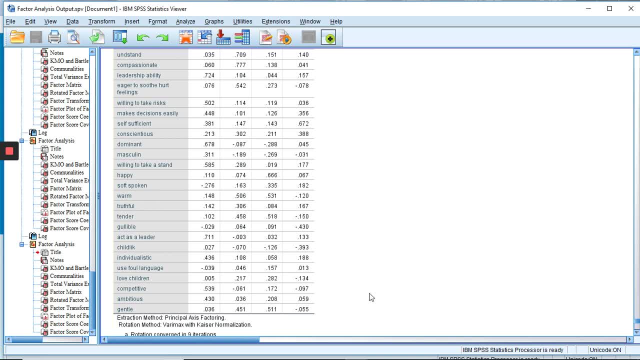 then it's complex, which means it's measuring too big of a thing, And so a couple different factors are picking it up, essentially. So you're gentle over here and you're gentle here. Well, how do you distinguish between that? It's not really great. So, um, I need to add that into my write-up because 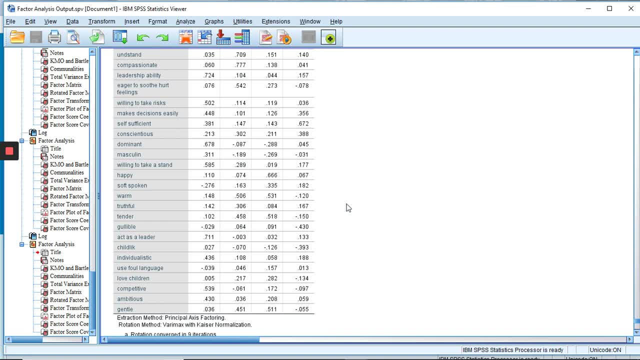 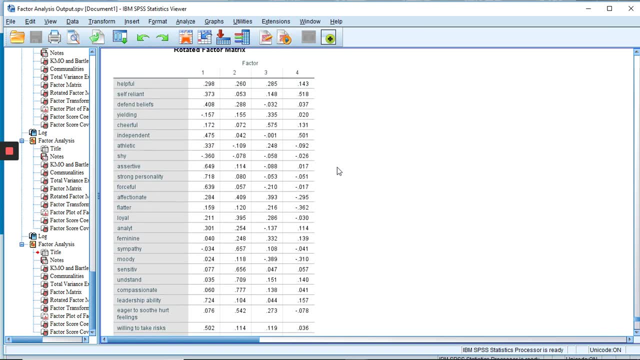 they had just warm and and independent and I had gentle and independent, but it's actually gentle, warm and independent. up here is 0.6.. It's 475 over here and 0.501 over here. So those are the complex variables, Um. 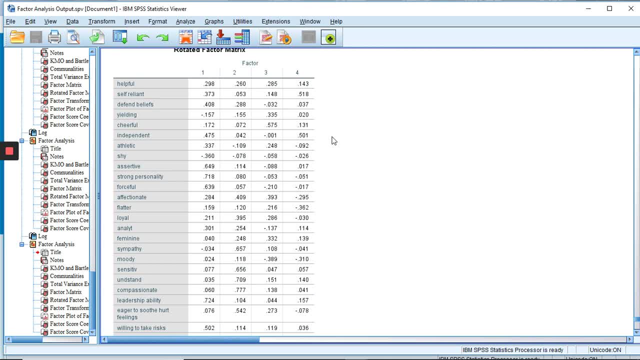 and so I'm going to have to update my chart a little bit. That's one of the things. like I said, that's been very hard is going through this whole entire chart of numbers and making sure you pick out all the right ones. I wish I could like print it out and highlight, but um, I I didn't do that. 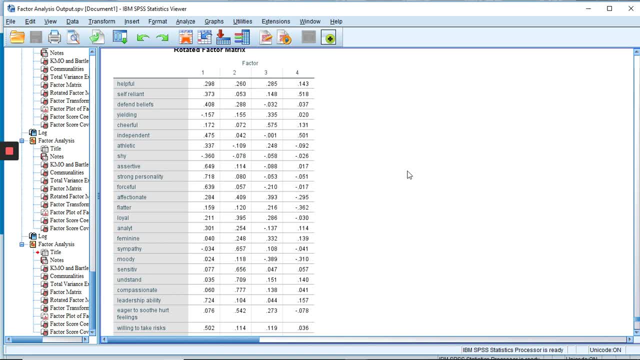 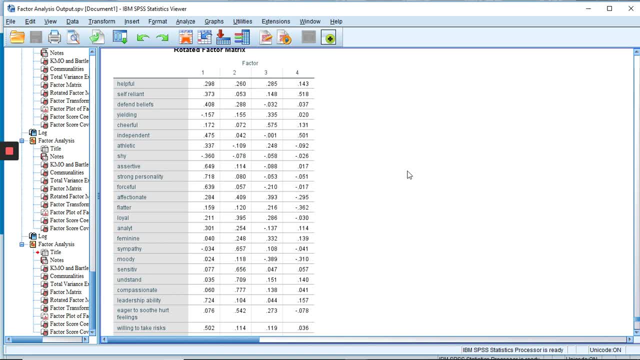 on the second factor, because I left out warm, So, um, add that one in. So, yeah, factor three is gentle, tender, warm, happy and cheerful, Um, and if I'm missing any others, comment in the comments. and then, uh, the fourth factor. there should just be three which we had found before. 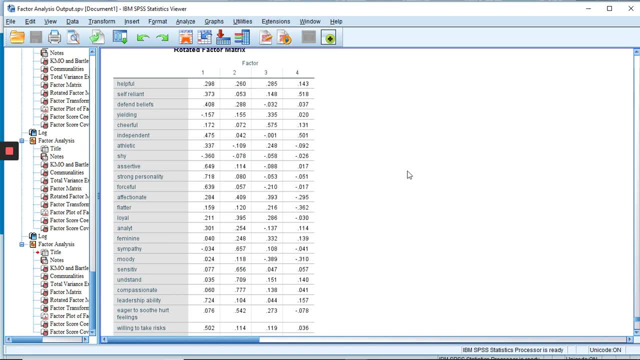 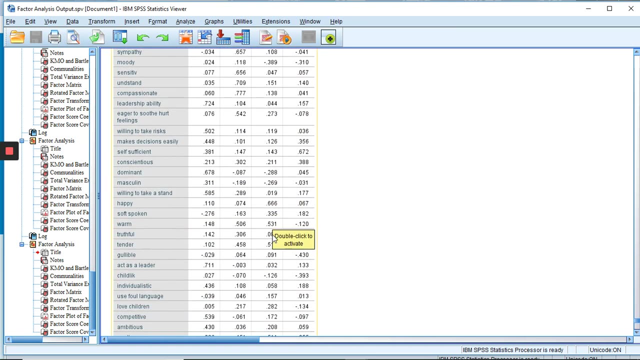 which was self-reliant, independent and self-sufficient. So, um, factor three. if you're thinking about what, what does it mean to be gentle, warm, tender, happy, cheerful? and then some of the negative ones. I think moody was like the most negative. Let me see Where's moody. 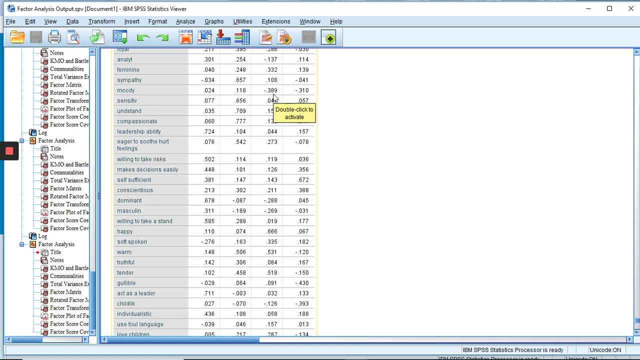 Yeah, Negative 0.389.. So you're not moody, You're just kind of a happy-go-lucky kind of person. I guess you're just got you know. it's the nature of what they're describing, right? So what would 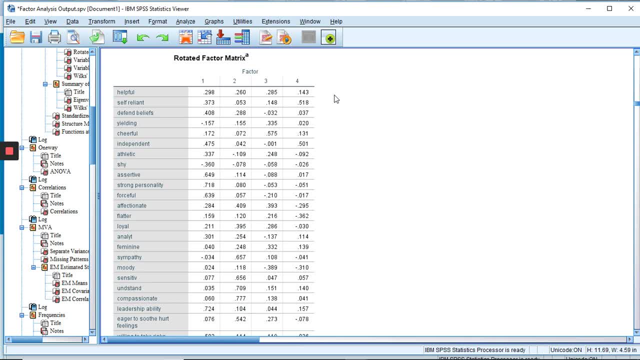 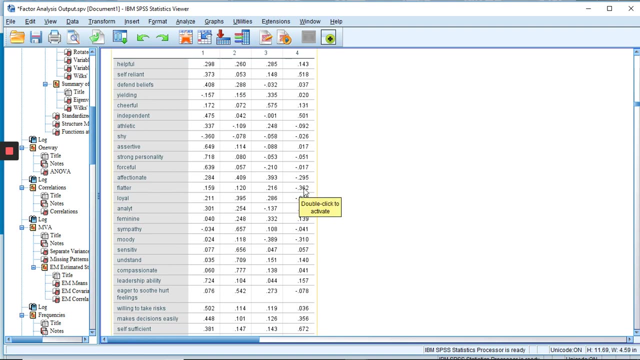 you call that. I think I put cheerful nature. I forget what the book called that one Um, and then the last one here, uh, the the three self-reliant, independent and self-sufficient. let's see what it's, what the opposite is: Flatter. I don't know if I don't know, if that's. 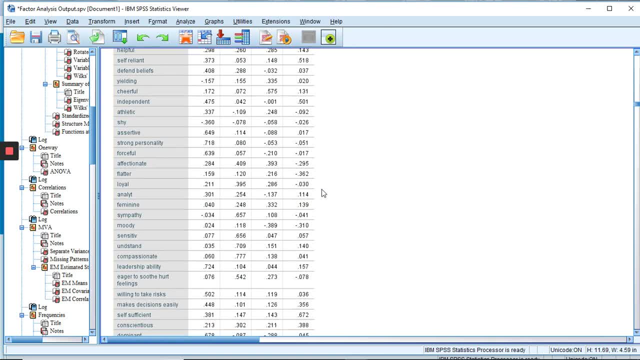 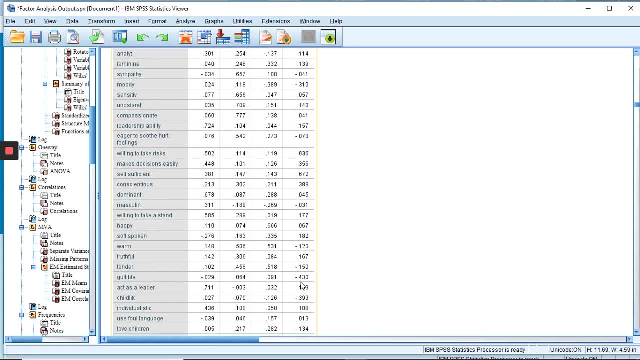 flattery, Like you're likely to be flattered by someone. I don't know what they're trying to say. They're moody, again as low um gullible, So you're kind of an independent thinker, right. 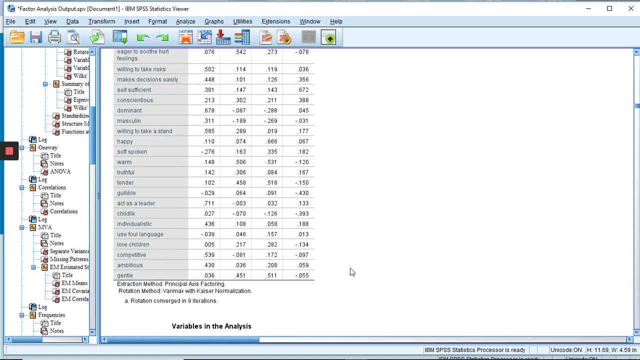 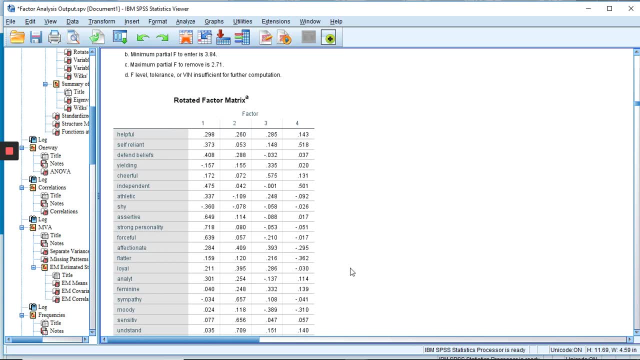 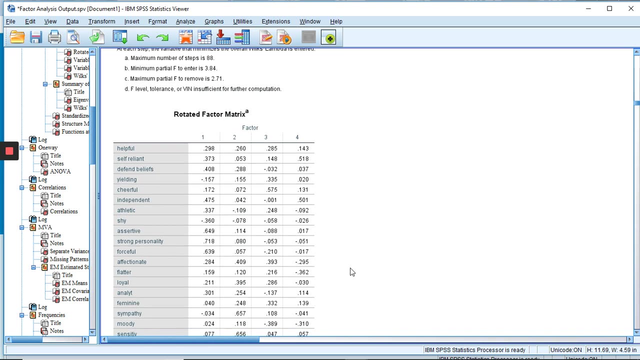 If you're self-reliant, independent, you're not very gullible, self-sufficient. so, um, what would you call that? I think I. I think I called it independence or independent thinker, or something like that. So, um, so yeah, basically, when you describe the nature of the, 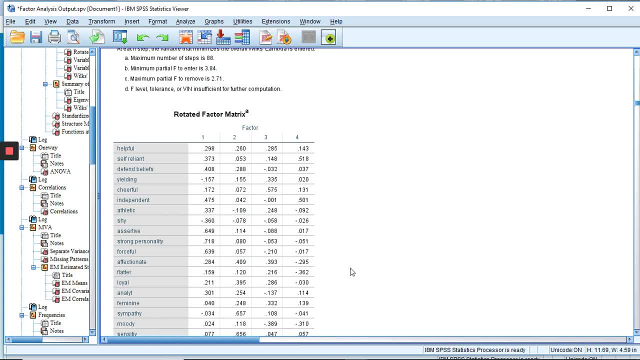 factors. you list out all these, you list out the factor loadings and you know, make it a nice APA table or whatever and give it a name and talk about why you gave it that name. Um, so, that would be great to do for you. Um so, yeah, that's that's. that's a great way to do it. Um so, 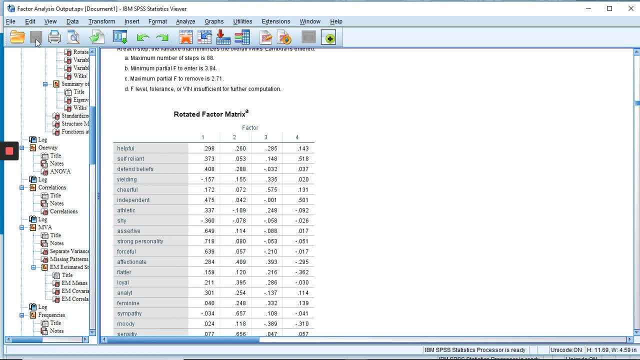 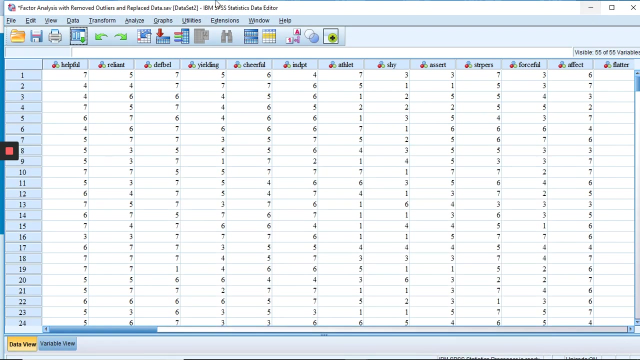 explaining the nature of the factors and then the rotation. this is where we need to decide between oblique and orthogonal, And so, basically, with oblique, it essentially um forces some correlations of on the factors themselves, And so it's it's good to use if you have um. 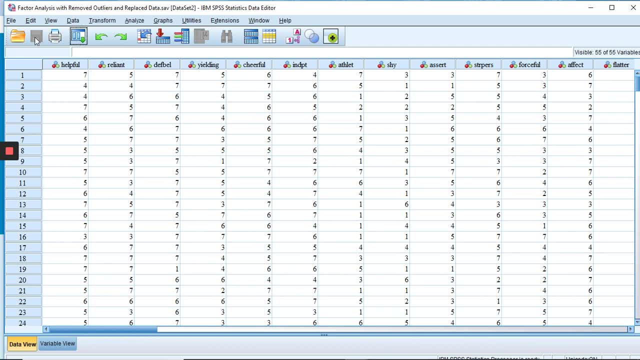 high correlations between um, oblique and orthogonal And so basically with oblique, between the factors already um, and it's not great to use if you're not showing um high correlations. So if you run it and the correlations aren't that great, 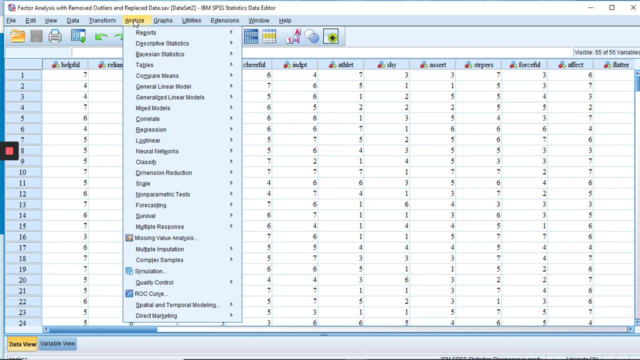 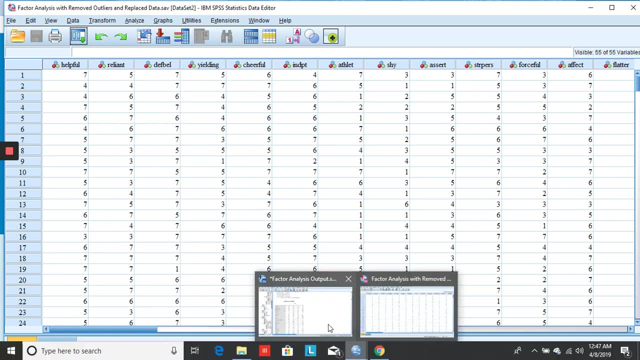 then that's kind of the indication that you probably um don't want to use it. So we already, if we go back to our output for one second, one more second, um what we did here. here's the factor score covariance matrix. We don't have a correlation matrix. 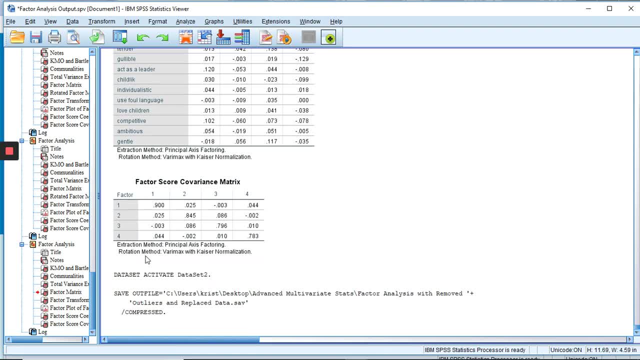 um, I think, because this one is, the is the very max, or um orthogonal one, And so here you can see, um there's, there's not particularly strong correlations, other than obviously one to one. you know that's correlated with itself, But other than that nothing is particularly 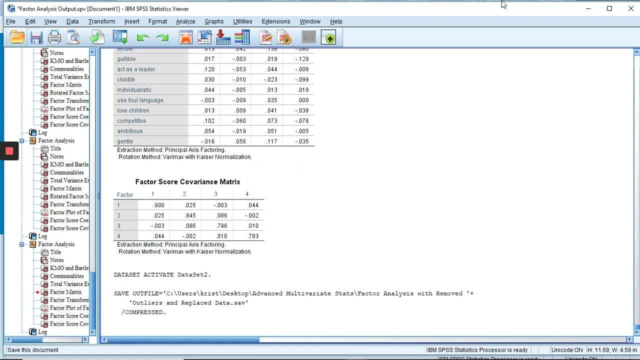 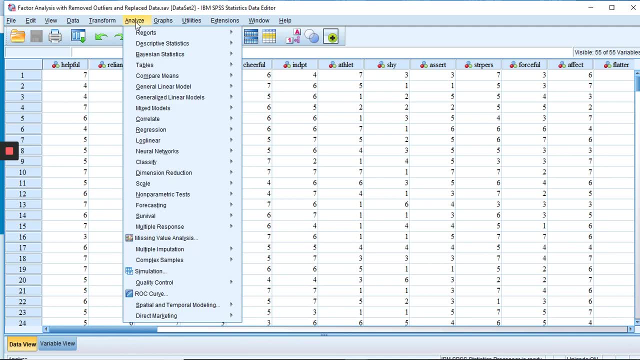 striking, and we can use that to compare um when we talk about which rotation to actually report on. The factor loadings will be different, And so that's that's why it matters Um, and so we also want to look at those um when we do this too, So go back. 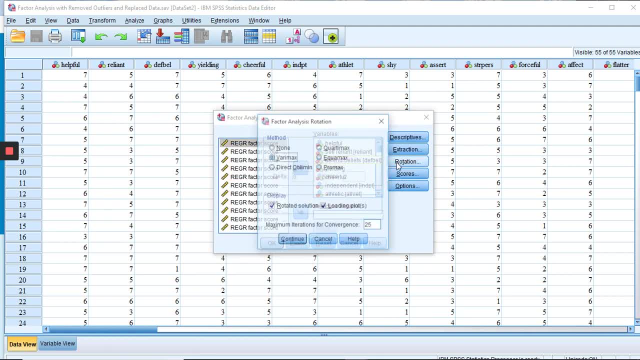 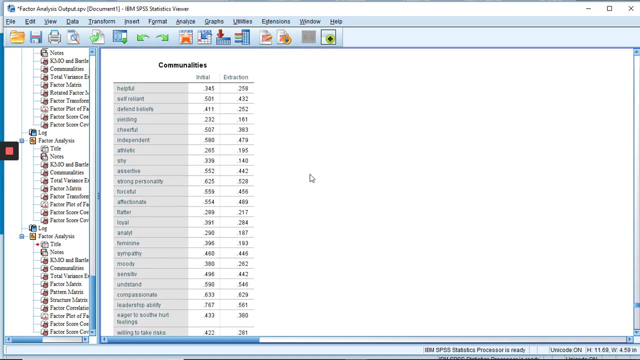 to your factor analysis here and in the rotation section. this is when we're going to do the pro max and two and we're going to hit, continue and go ahead and just pull that up Now, um, you know, these numbers don't change, That's all still the same. Um, and so what we are looking at here? 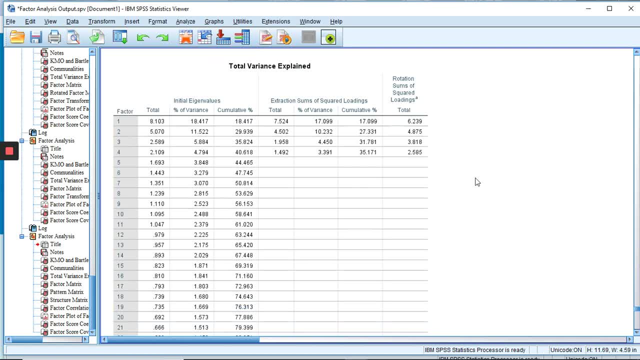 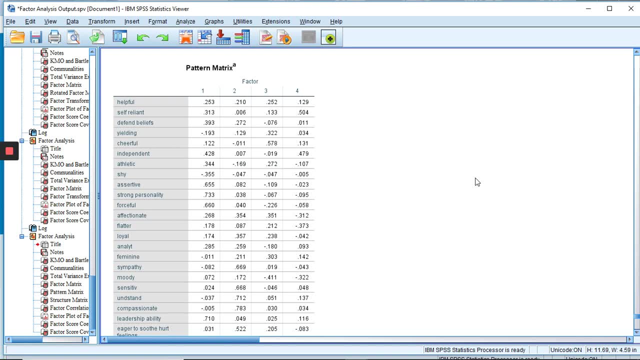 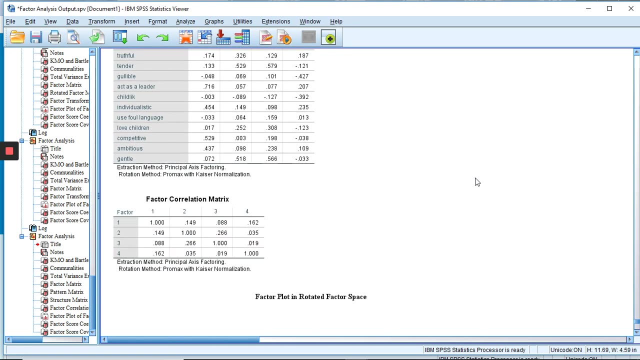 these numbers look still the same. Yeah, These are still the same. So the rotation really just changes. the factor loadings and um, the, the correlation. what is cause? it basically forces correlations, um between the factors Um, and. so let's look here at what the correlations are in the factor correlation matrix. 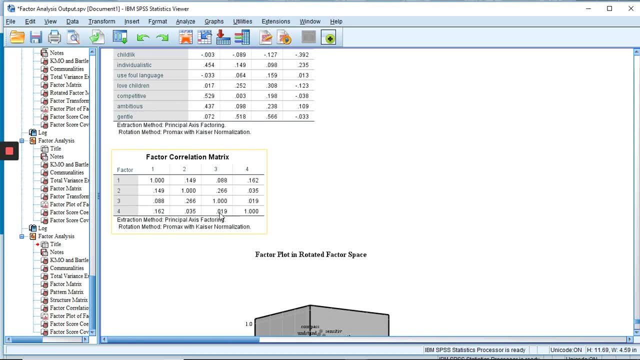 And you can see here there's not any like real striking correlations. The biggest one is between factors three and two, And so- and actually I um messed that up when I first did it, So now I'm realizing I'm going to. 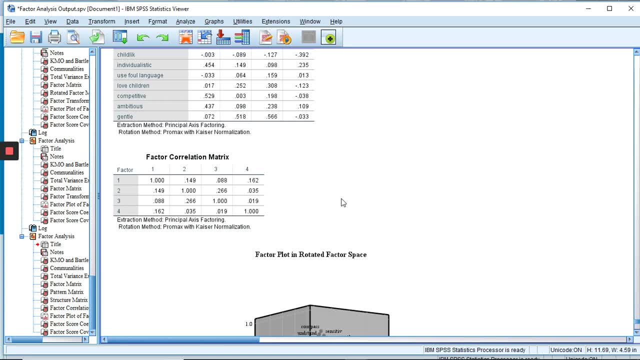 have to go back and fix that in my assignment, but um, that agrees with what the book says. They have a slightly different number again cause some of their calculations are different and they deleted a different number of outliers and whatever. So that's okay, It's pretty close. 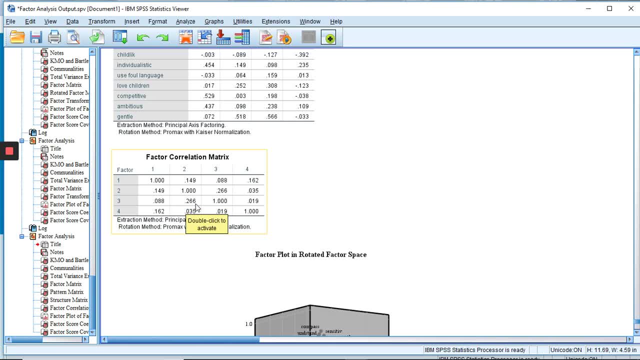 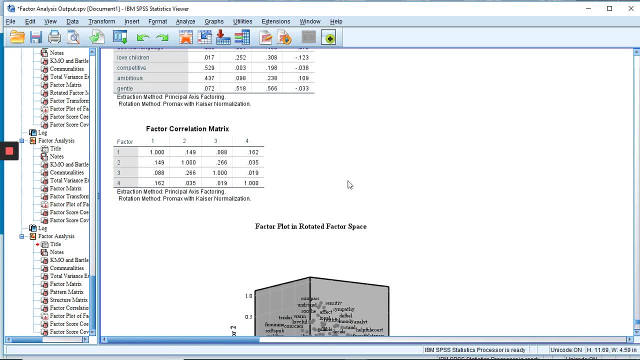 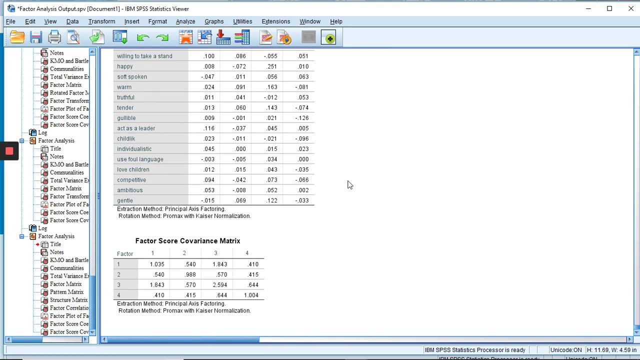 to what they were saying. Um, but it's, it's not the biggest correlation. What you want to look at is the, the scatter plot of factors. So it's not the biggest correlation, but it's not the biggest correlation, Um, and so we can do that in a minute And, in fact, our factor score. we should have saved those. 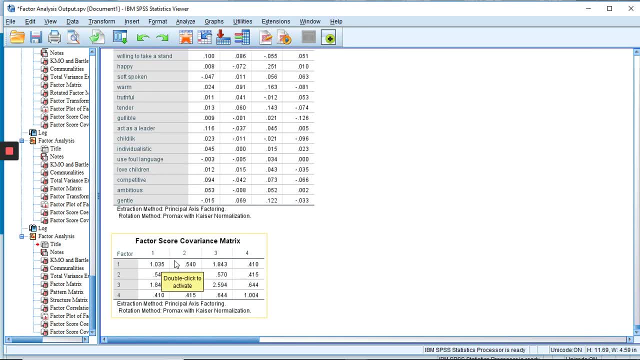 factor scores. What I was comparing here when I did my assignment was the covariance matrices for both, because that kind of shows. I felt like three and one, you know, was higher there. but um, let's see, Yeah, Three and two, Yeah, So I don't understand that fully. Um, but if we look 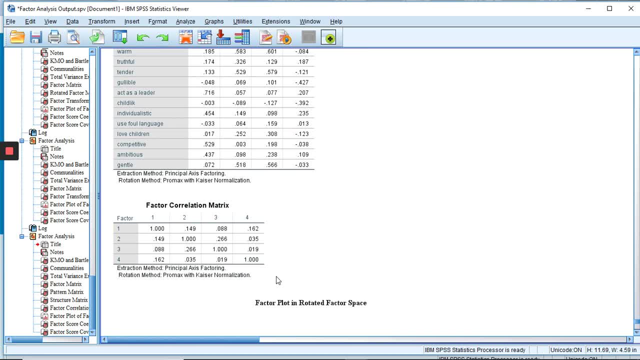 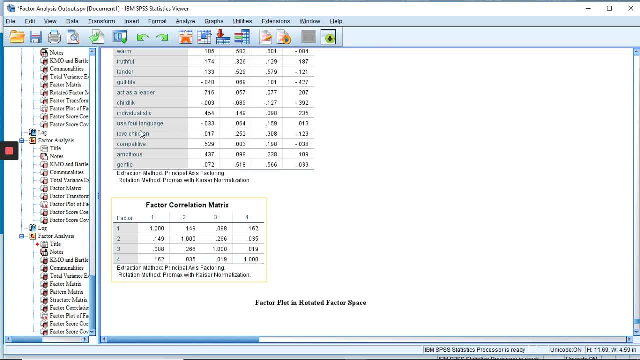 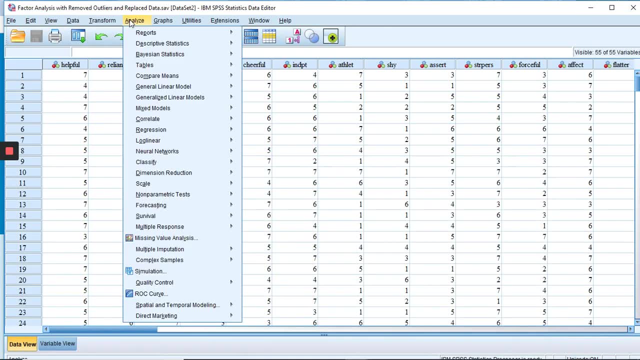 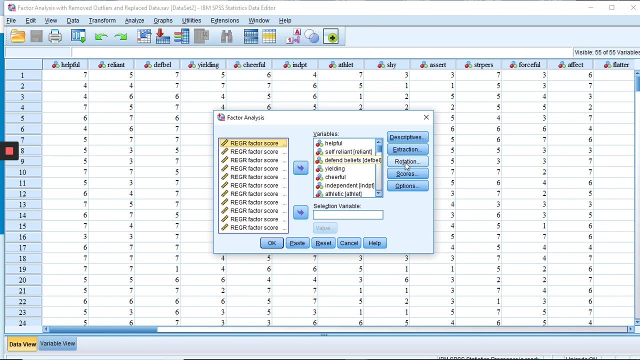 Um, not really, but let's, we're going to have to run it again and save those factor loading. I mean factor scores, So unfortunately I had unchecked that before. So let's go back to dimension reduction factor And we're going to do everything the same. We're just going to save as variables this time. 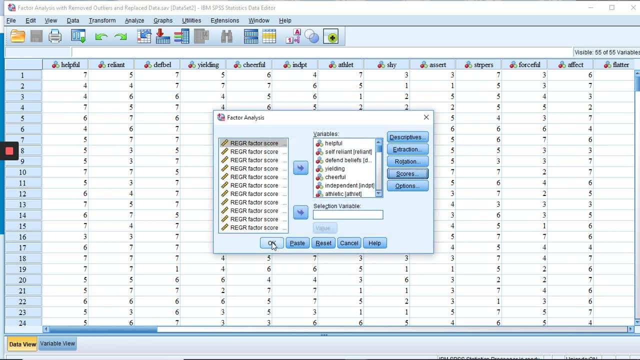 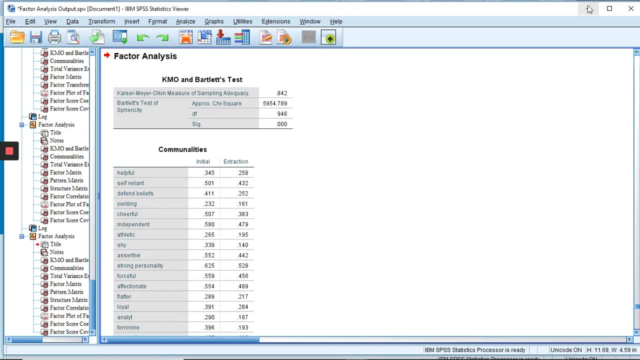 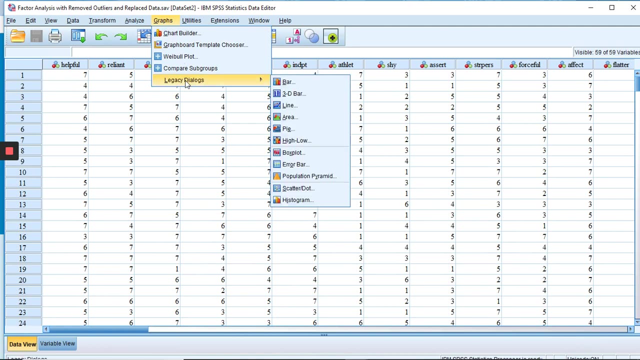 so that we have them. that way, we can do the scatter plots. That's what we need them for, So click Okay Again. your output's going to be the same, um, except you just have new variables in your data set here. So now we can go to graphs, legacy, dialogue, scatter dot. 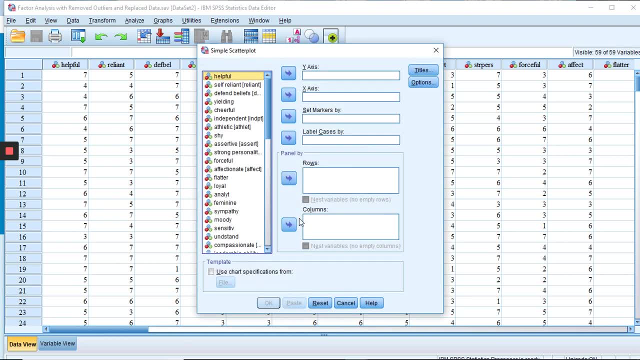 and we can do a simple scatter And we are going to go down Here all the way. the very bottom ones are going to be the last four here And we're going to want to plot: uh, two by three. So you see, that says score two, score three. That's all we need to do. 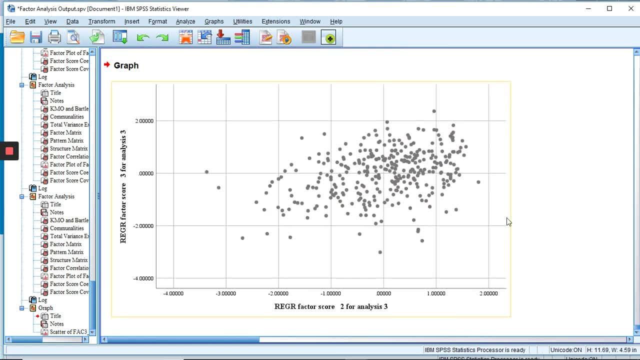 Click Okay, And here we have our scatter plot, which is a pretty nice oval shape. It's okay, Um, but I think ultimately they decided, um that it wasn't really worth it to do the oblique, because it's not. 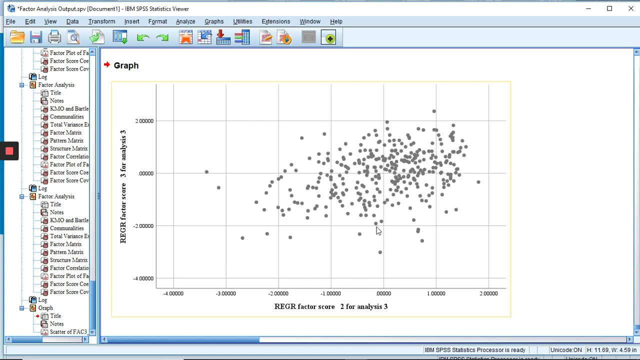 perfectly correlated and it's not. it's not strong enough And this is the most strong one that there is. So I think that's kind of how you would show that. Um, maybe you could argue for: okay, yeah, the, the oval is here, but look at all these ones kind of way out here. 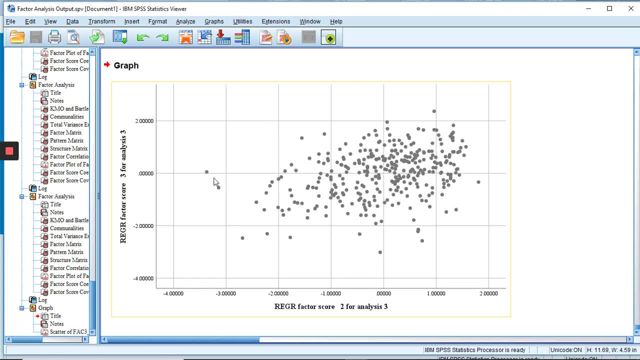 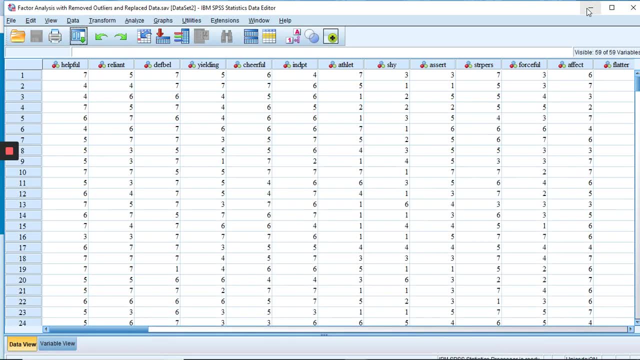 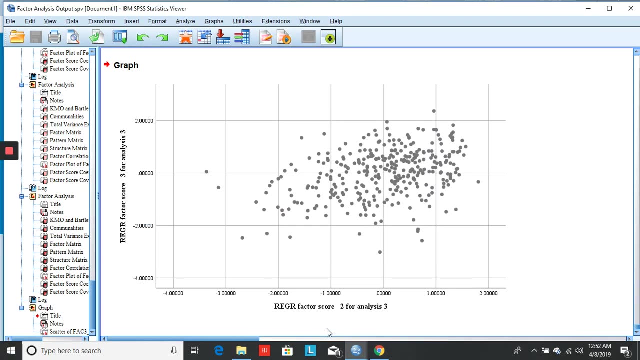 It's not the most strong case for highly correlated factors that would benefit from an oblique rotation. So that is why we chose to um. we will analyze what we already did. We don't have to run it again. It's already in our output, The um. it's going to be a mess in our output because we have to find it. 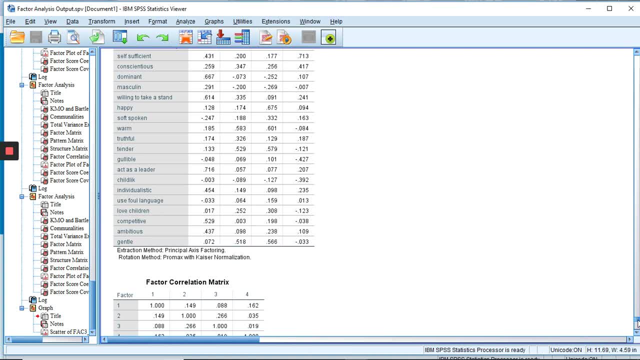 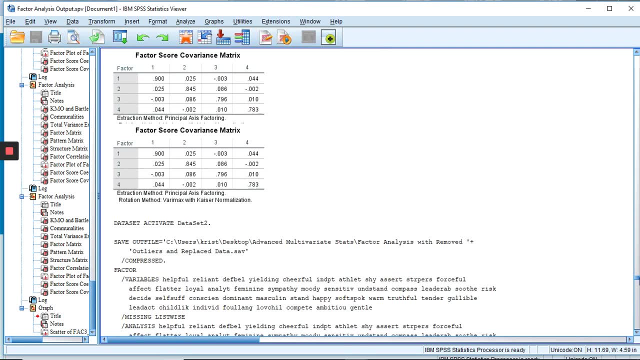 Uh, so sometimes I run it again anyway because it's easier to find it. finally, but ultimately it's in here, Okay, Okay, It's in here and you can scroll up and look, for it will show you. you wanted the principal axis, factoring with the very max. 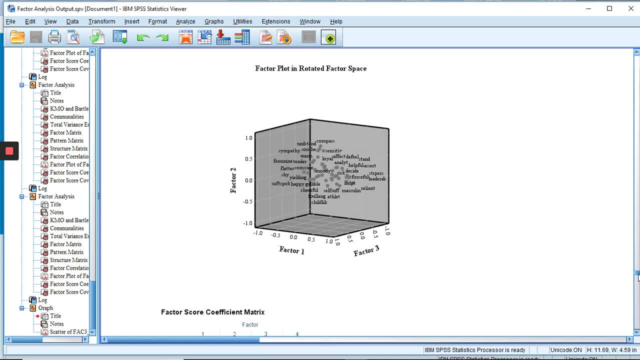 So if you have that, then you're looking at the right thing. OK, so we've already talked about the nature of the factors And when we were doing that, we were looking at: oh, that's the other thing we can look at. 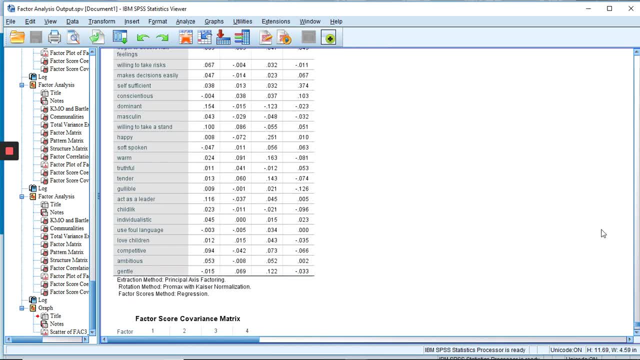 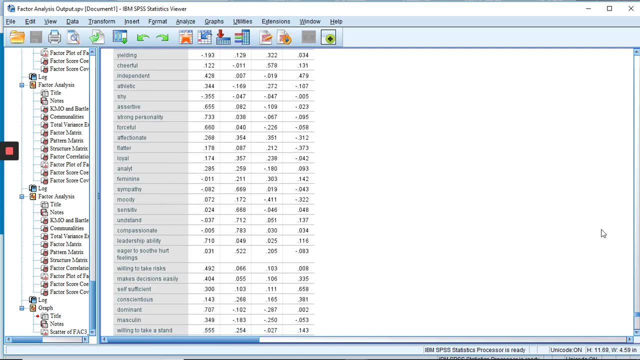 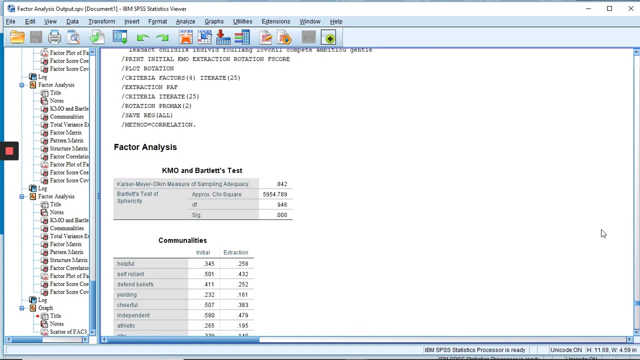 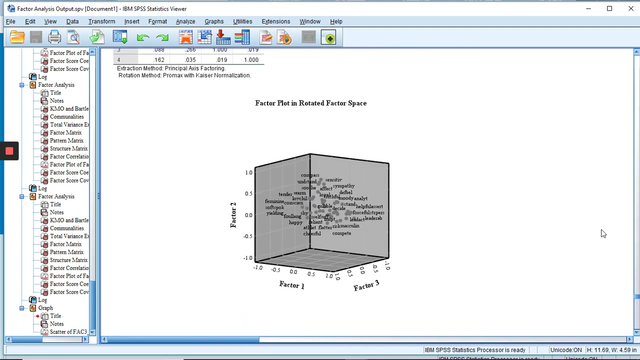 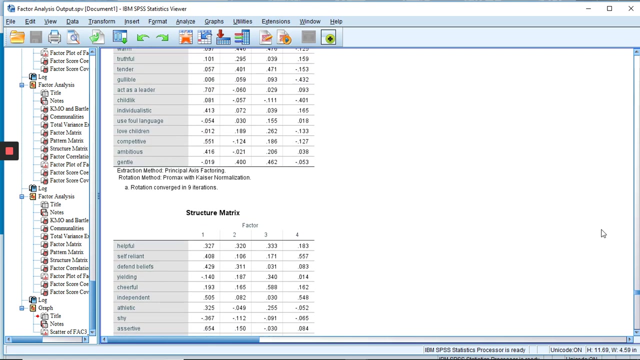 OK, so in the one let's look at the factor loadings, which is not the factor score, It's the rotated factor matrix. Oh, do you not get that? Where did I have that? I thought that I compared. Was it the structure matrix? 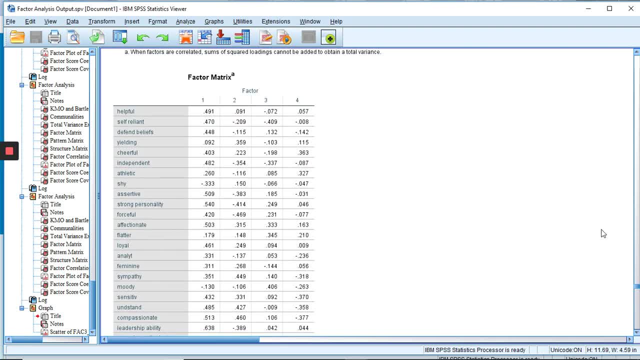 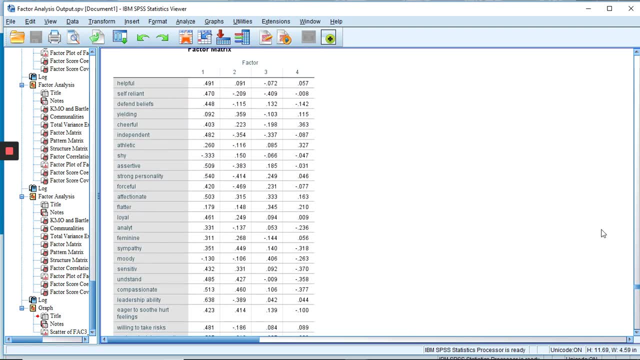 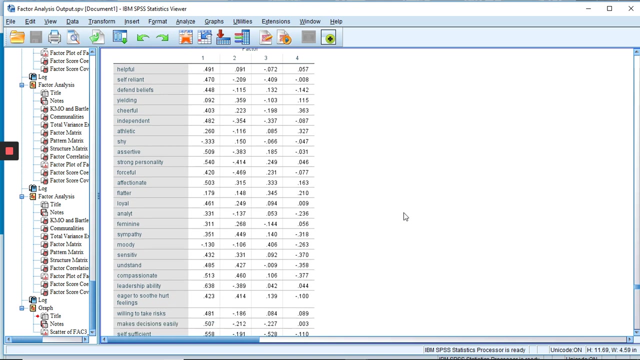 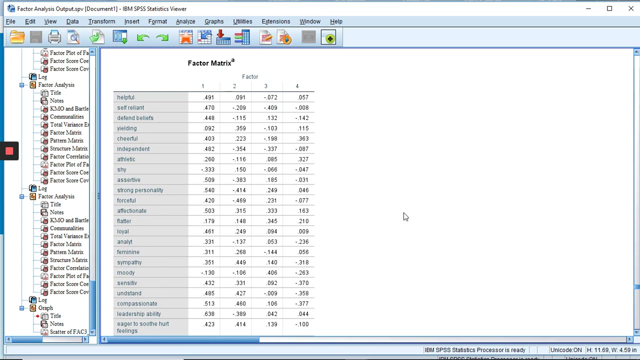 Oh boy, Sorry guys, I guess it's the factor matrix here. What does it say at the end? OK, so I guess here is what I, what I compared. Let me see, Yeah, that's what I did. OK, this factor matrix here. I basically compared these numbers to the rotated factors on the orthogonal one. 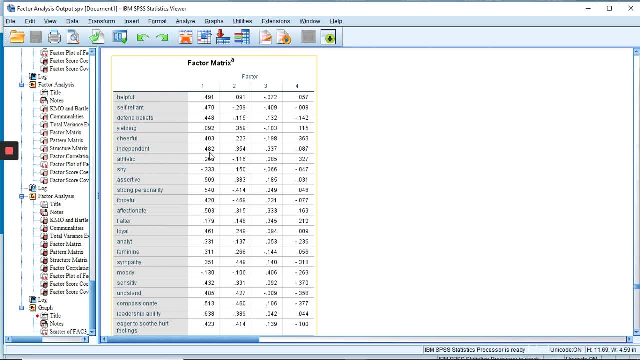 And like take independent, for example, here it's 0.482 and in the other one it was 0.474.. So actually this is a little bit stronger but, like all the others were not so assertive, here is 0.509 and it was 0.648 before. strong personality is 0.540.. 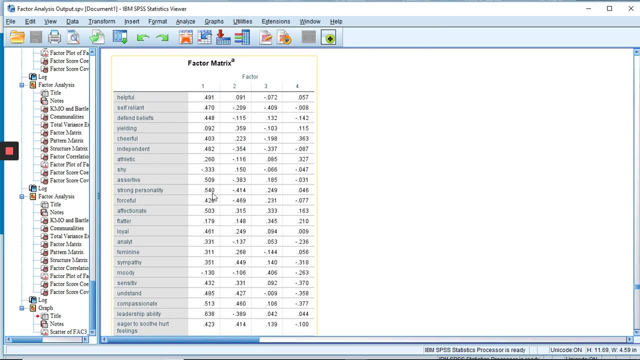 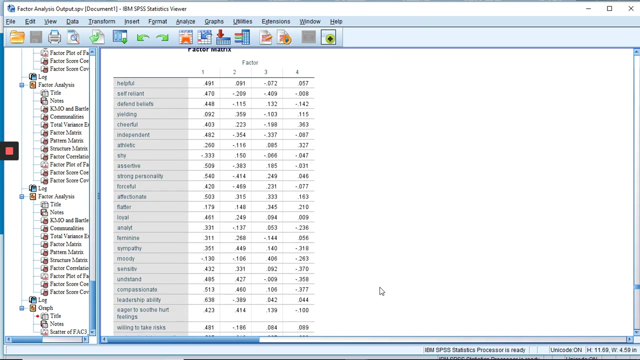 It was 0.726 in the other rotation, Forceful. Yeah, Yeah, Yeah, Forceful is below. Now this changes it. It was it's 0.420 and it was 0.625.. So I think I made the case for the fact that the factor loadings are also not as strong, but that that could be not quite right of an explanation, because this is the factor matrix. 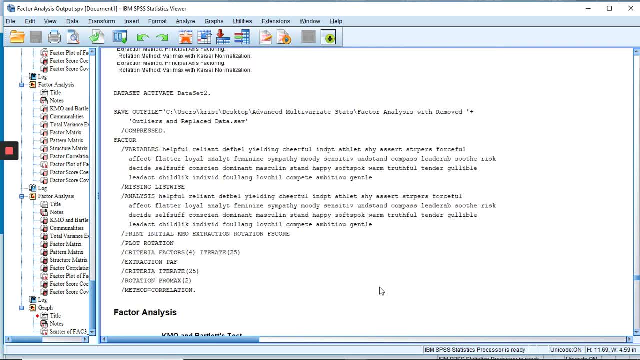 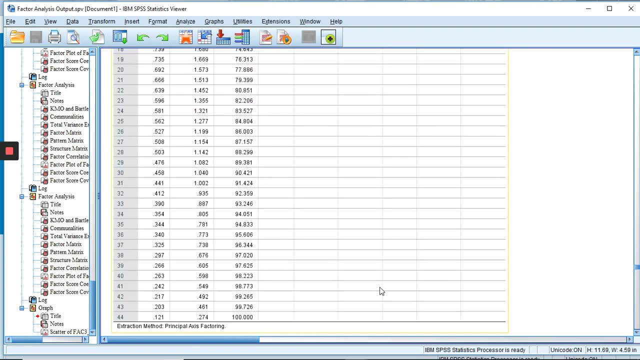 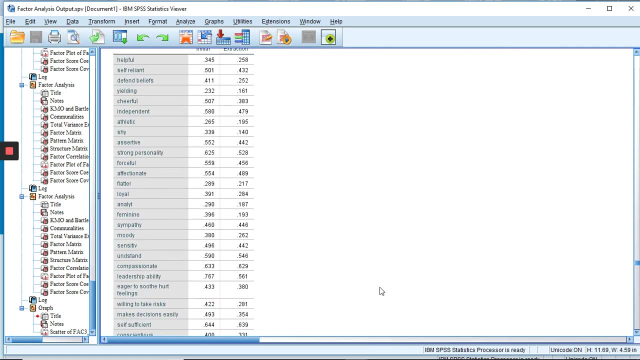 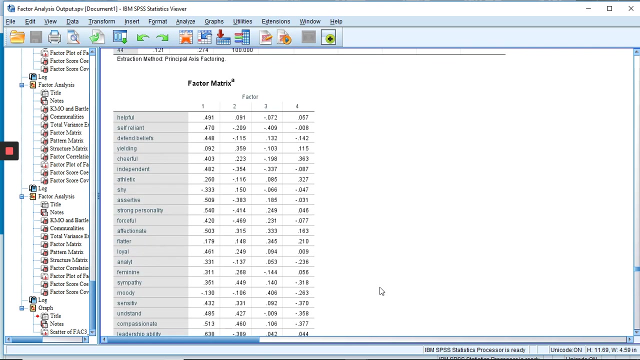 And the other thing I was looking at, if we go up to our other one, that was: Let me see, is this the? where did we get it here? Rotation varimax: Yeah, Okay, That's our factor matrix. Yeah. 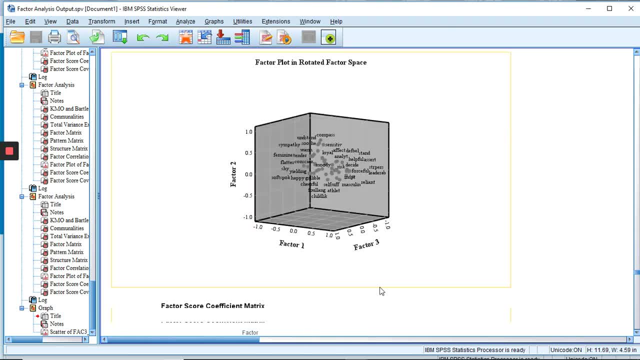 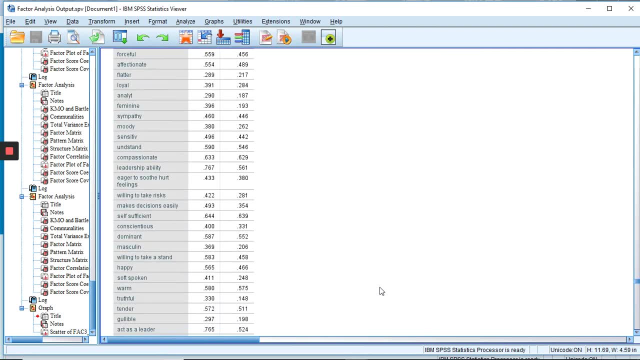 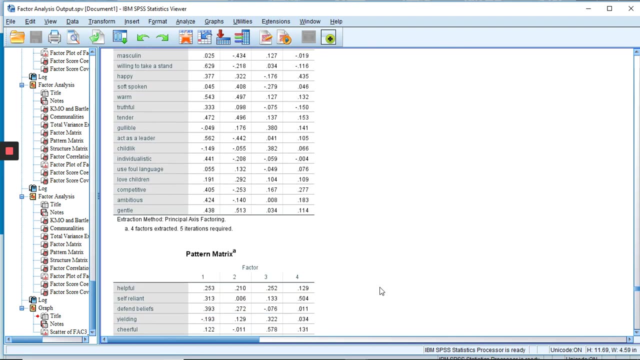 So those factor matrix matrices are the same. It's the rotated factor matrix It's different. My goodness, These outputs are so difficult to find anything in. I I really find it difficult. Where was that Rotated? Yeah, See, this is the ones the pro max. 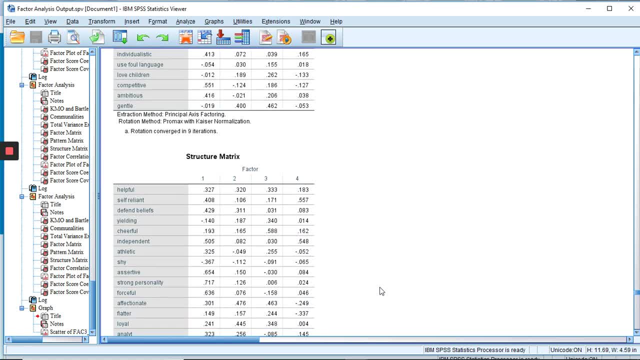 Oh my gosh, You might want to, And this is what I did when I was making my assignment. Oh, here it is. Here's the rotated factor matrix. Okay, But this was for Okay, So be careful, This is for the five factors. 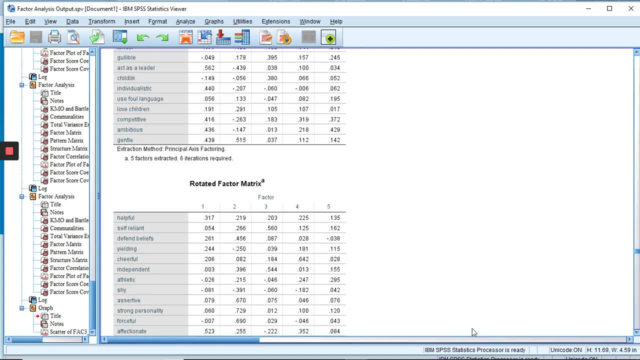 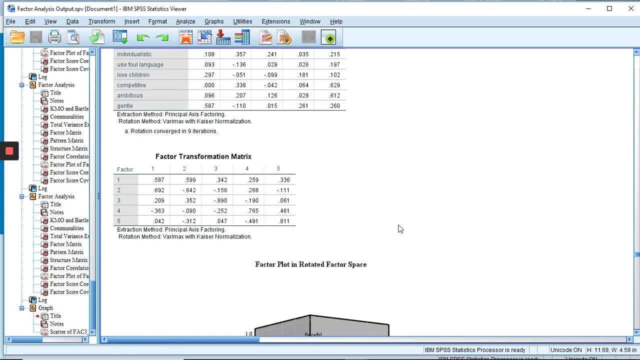 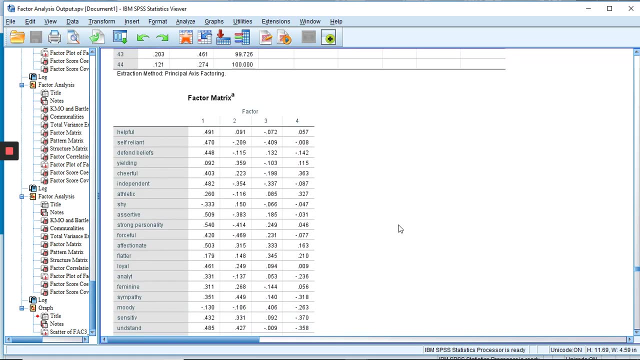 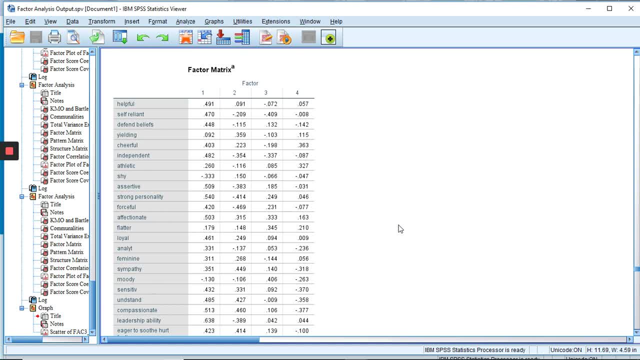 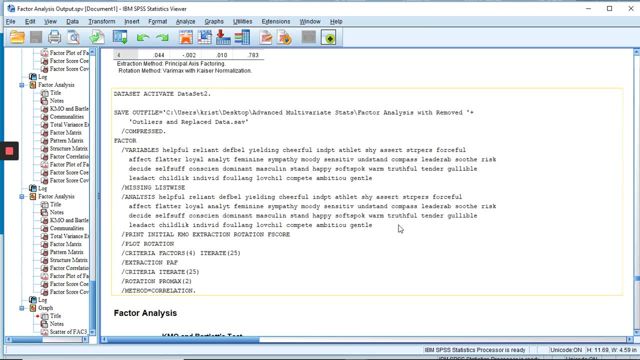 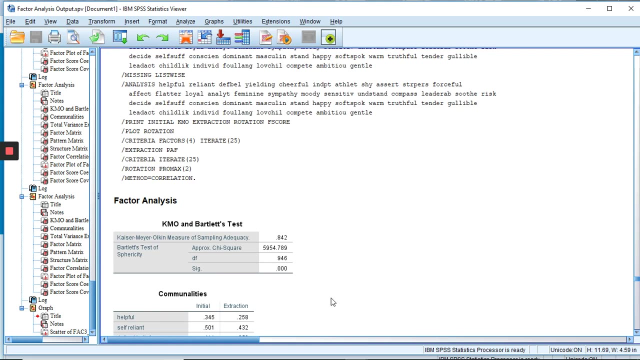 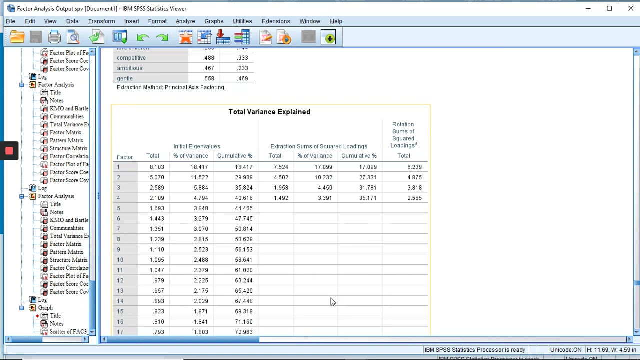 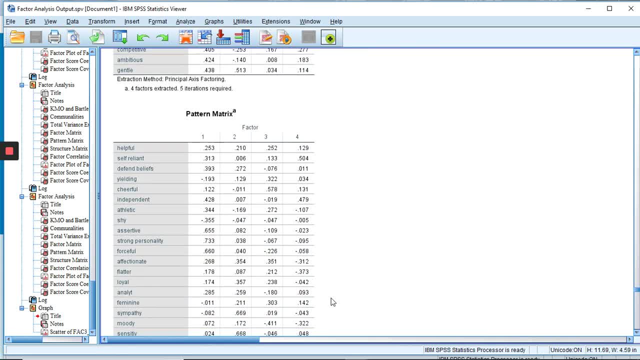 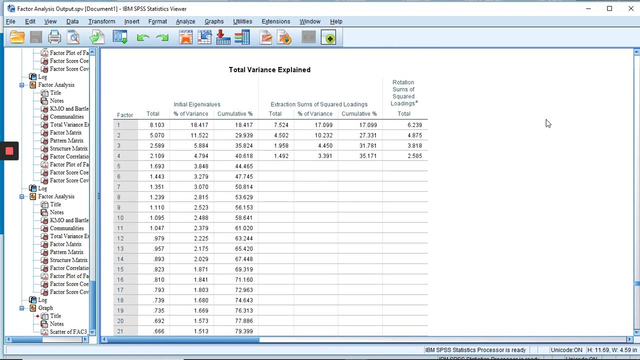 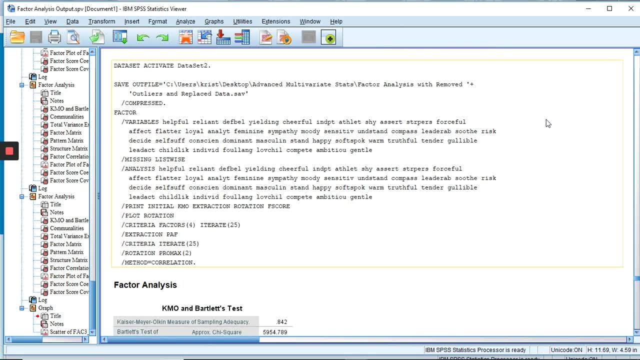 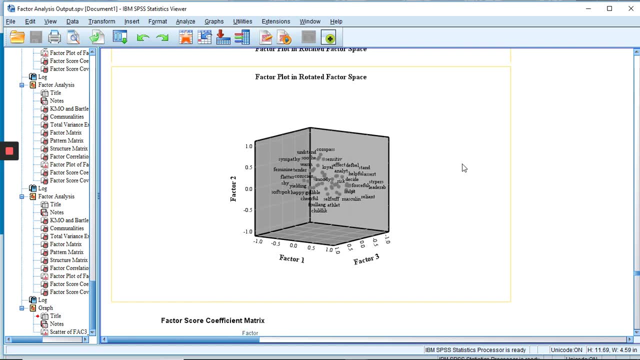 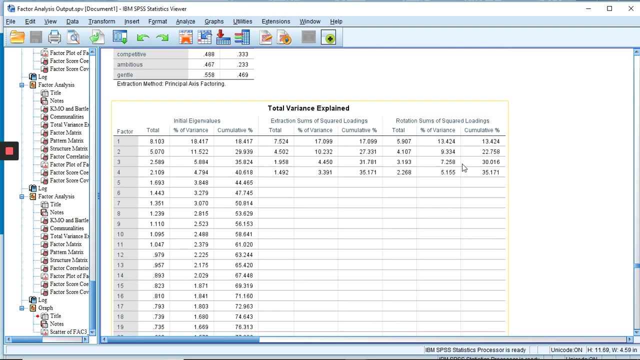 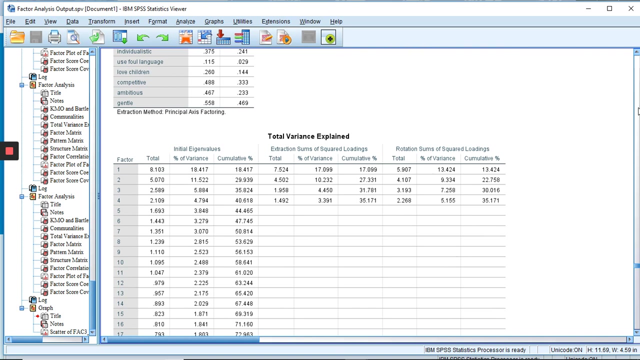 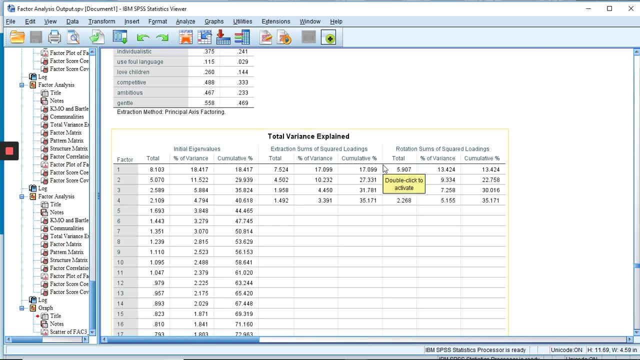 Okay, Okay, Okay, right here, And I wonder. I didn't write out all my calculations, but let me just confirm that I have it right. All of these should add up to 17.53, if I did it right. So let's. 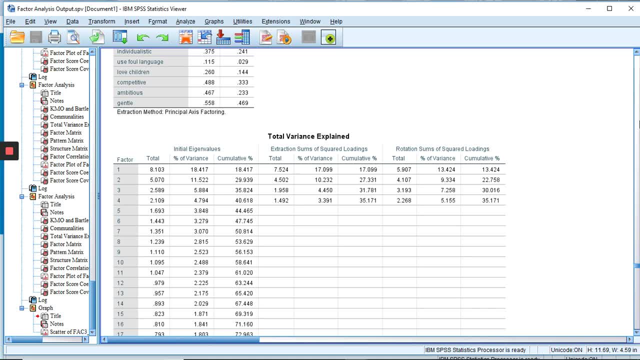 see 5.907 plus- you're going to need this too- 4.107 plus 3.193 plus 2.268.. Hmm, Okay, I'm going to rerun this because I'm sick of trying to find the thing in my output. 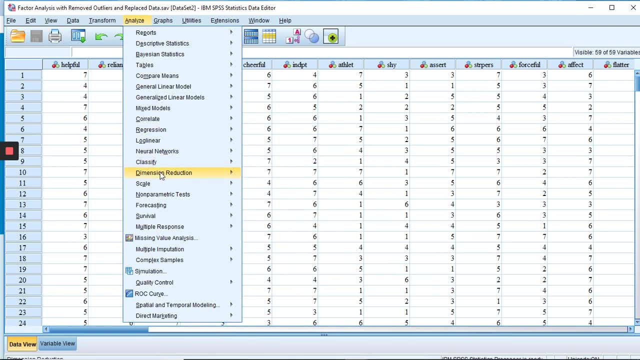 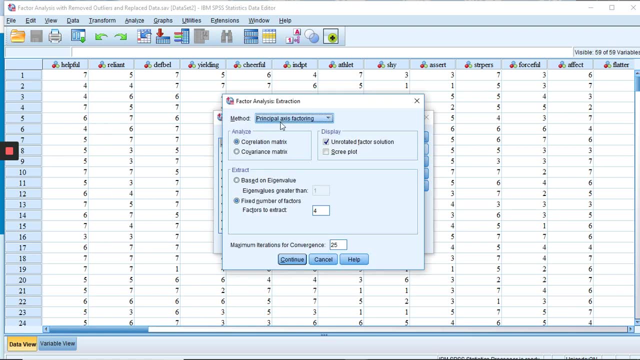 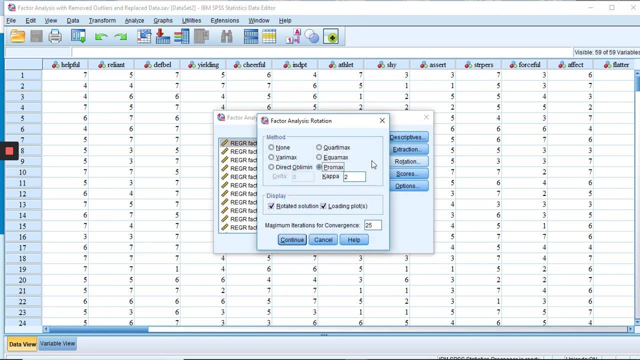 So run this again for the for real this time. This is our final real one. we're interpreting. Let's make sure we did it right. Extraction: principal axis factoring: We've got that Okay, Based on four factors. Good Rotation: We are going back to the very max We want. 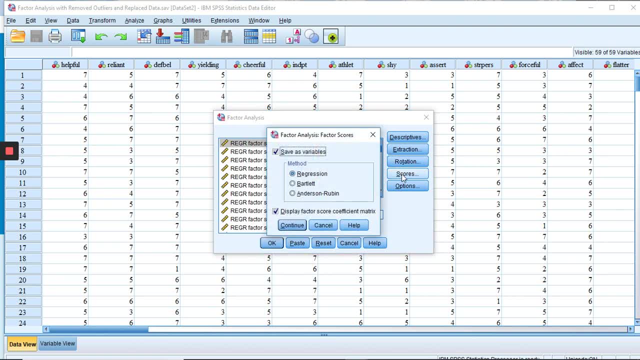 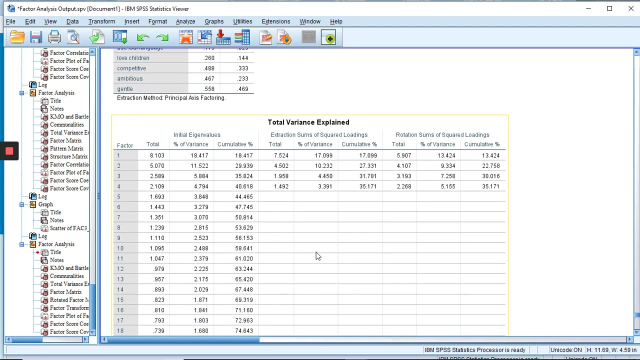 um scores. I don't think we're going to need this again And let's click Okay, Now we have it as our last output. All right, So here we are, and is that what I just came up with? 5.907 plus. yeah, this is the same 4.107.. I'm just trying to. I just don't understand. 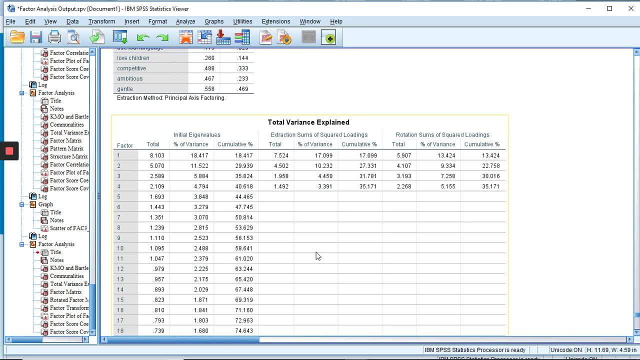 why this is different than what I calculated the first time. This is like so maddening. Don't you just love statistics? Okay, so for some reason I added wrong the first time, which is like so dumb. So when you're looking at the importance, you want the percent of variance explained by each factor. 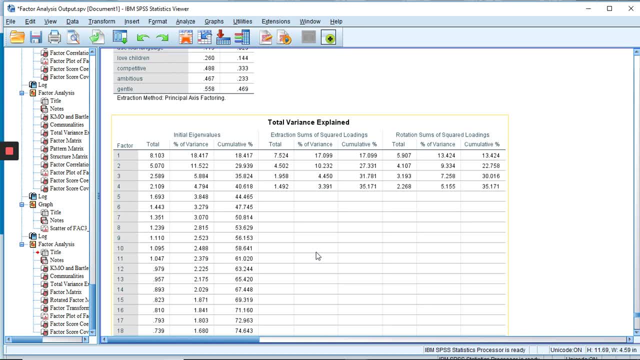 which is the sums of square loadings divided by the number of variables, which is 44.. So I made a handy dandy chart, which actually you know what. Let me look at my chart, because this will tell me where I got my numbers from. 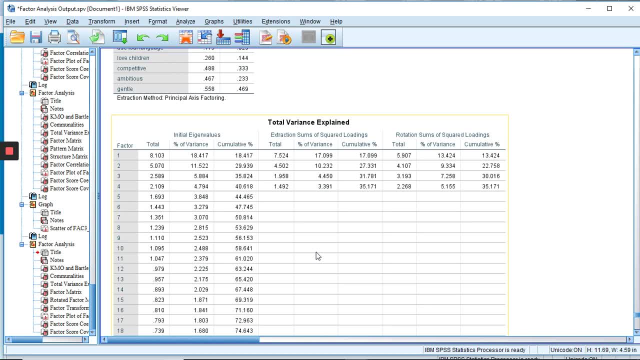 Believe it or not. I read this whole thing over. I had it all done. It looked great And I don't know why my numbers are different. Oh my gosh. So any who, what you want to do is basically use these numbers, which I can't now tell you because my numbers are slightly different. 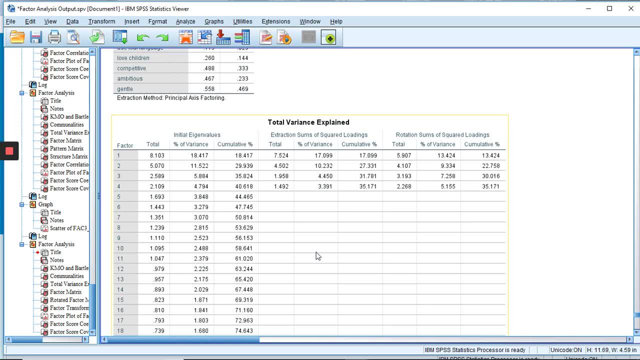 But basically divide each sum of square loading here by 44. And that is the percent of variance explained by that factor. And then the percent of covariance explained by the factor is the sum of square loading SSL divided by the sum of the SSLs, which in this case is 15. point something: 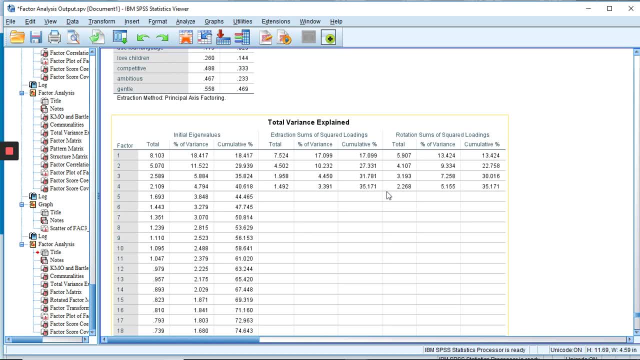 I cleared out my calculator. I'm not adding those four stinking numbers again. But yeah, and you want to use? Yeah, because I didn't use. it wasn't like I use these numbers either, So I don't know how that happened. 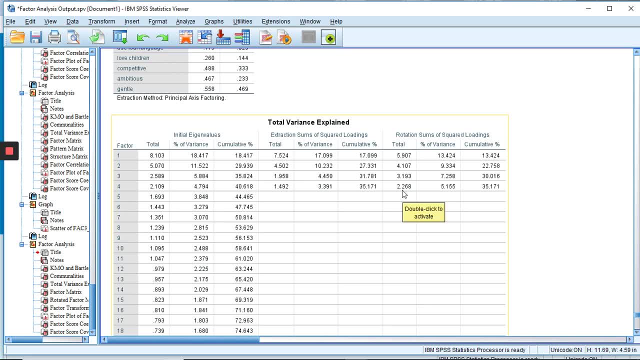 But anyway. so add these numbers up- It's 15 point something for it, or something like that- And so divide each of these numbers by that total, And that's the percent of the covariance explained by that factor. That will show you the importance which I will tell you, even though I maybe need to do the calculations again. 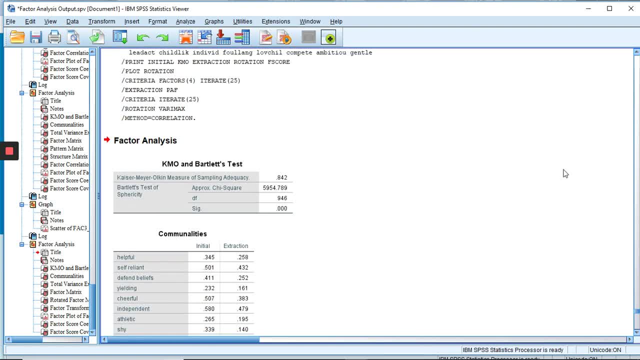 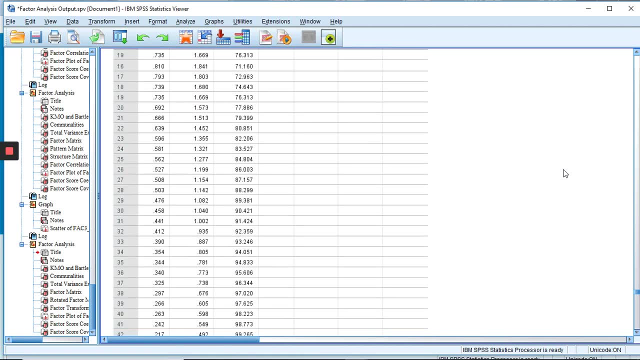 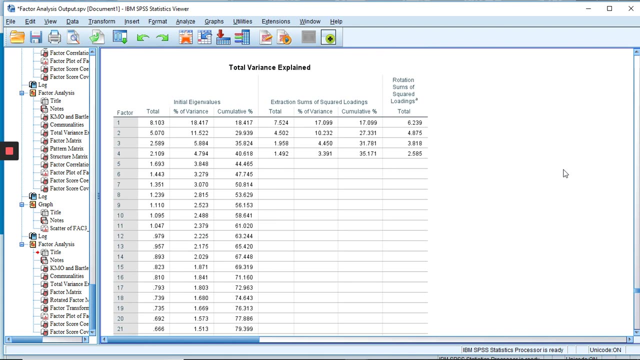 Or maybe you know what it's possible. I looked at the wrong thing, I wonder. let me just compare real quick my values to the oblique one, See if that's what I was looking at. No, that doesn't quite match either. 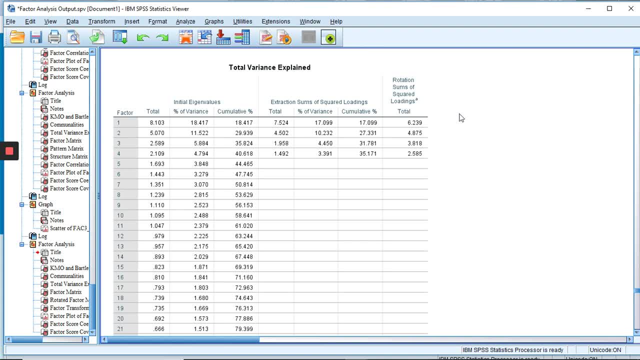 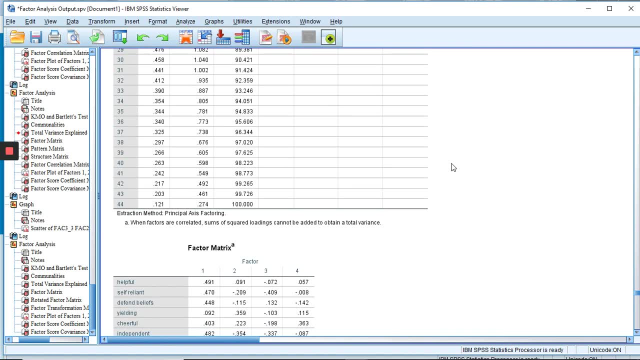 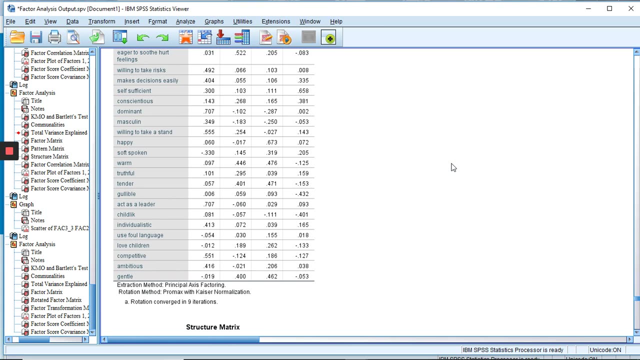 Does it? Oh, yep, it does Here, these are the numbers that I looked at. Don't make that same mistake. All right, was that? This was the one? that was. That's what I did. Okay, so I pulled numbers from the oblique. 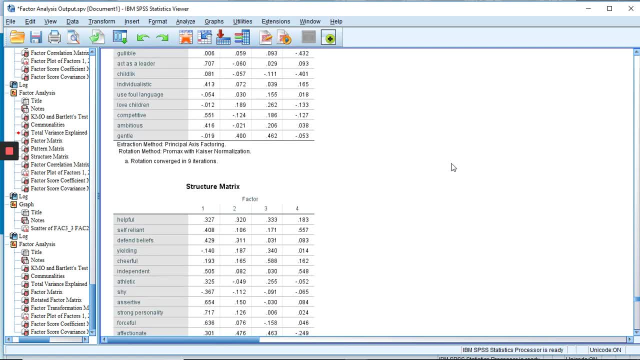 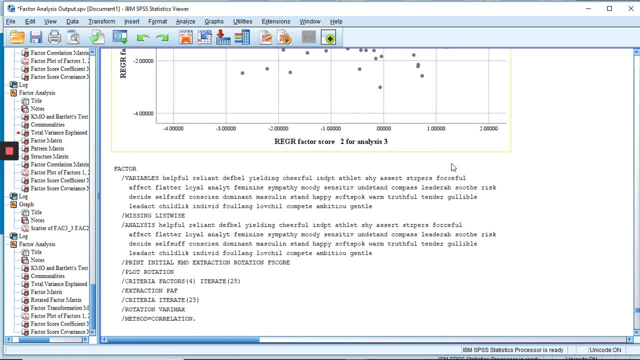 Oblique one: Yeah, okay, so good catch for me. I need to fix that, All right. so yeah, do go get those numbers. But basically it's not impressive. The percentage of the variance explained is not great. 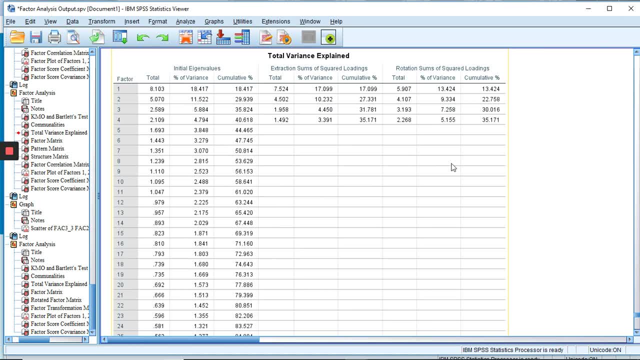 It's between like 4 and 16%- I think the book said So. they're probably right- And the percentage of the covariance explained is like 38% or so. according to the book, I had 35% And my other calculation. 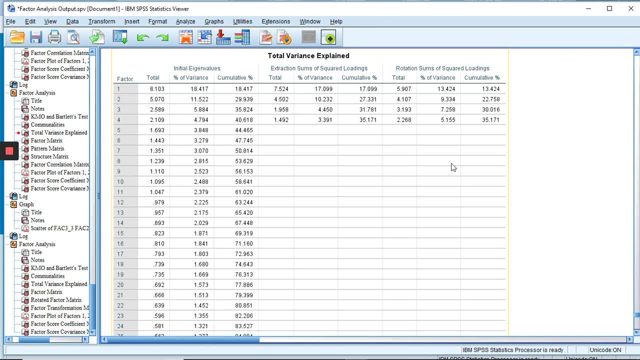 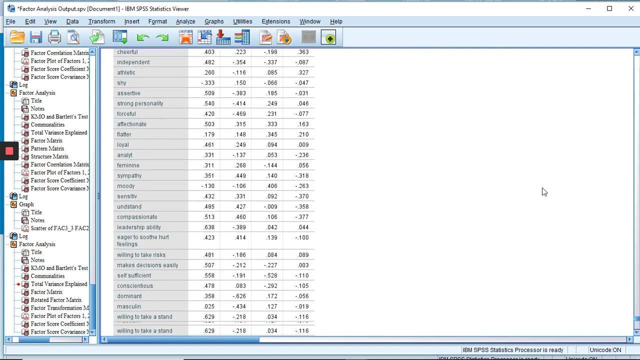 But you know, it's basically not super amazing. The book seemed okay, with factor one's covariance explained as an important thing, But that's it. So that's how you would write that up and make a little table- APA table for that. 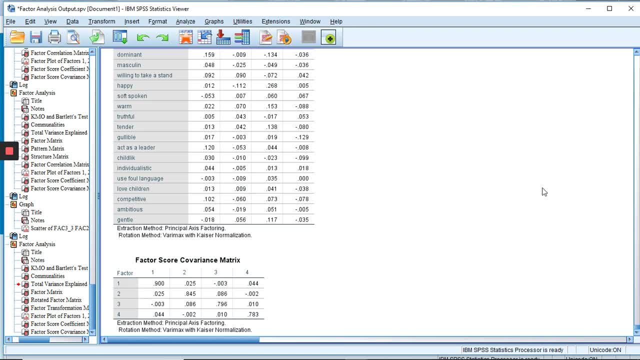 And that's it for the main analysis. So now we're just talking about a couple extra. And in the book it talks about internal consistency of factors. Ignore every single other thing the book says about it, because their way of finding it is totally different than an SPSS. 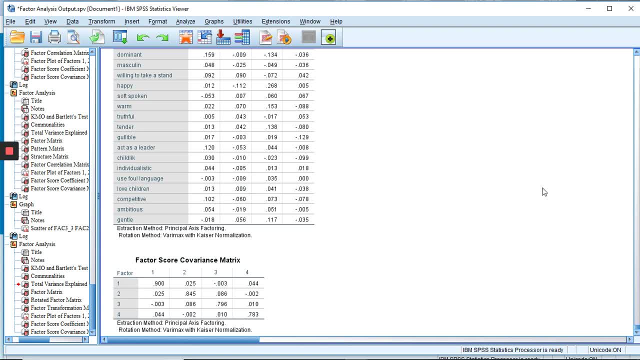 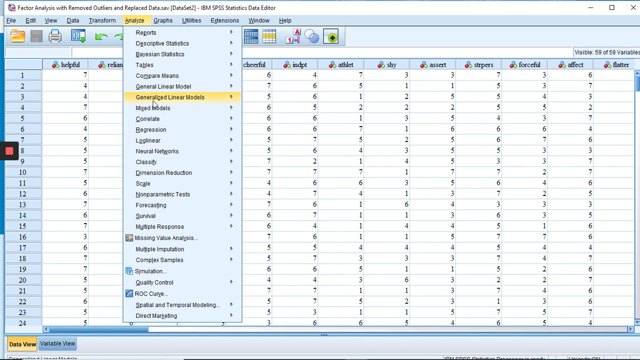 So I have a different book- It's called SPSS for Psychologists. that talks about how to find internal consistency in SPSS. So we are going to do that. So you're going to look for analog Size Scale Reliability analysis. 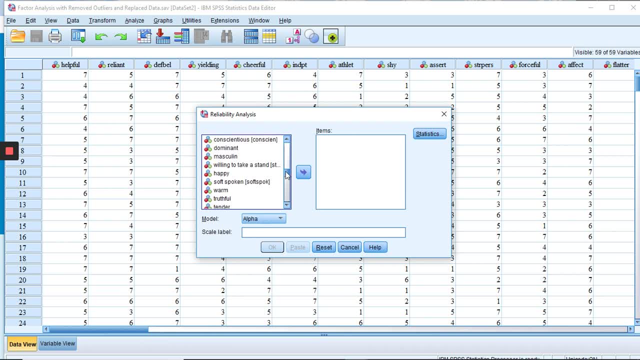 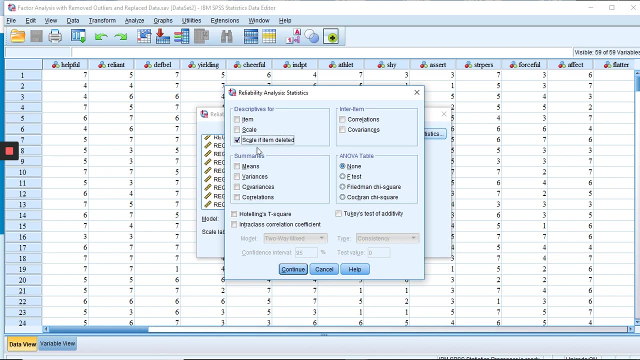 And we want to choose all 44 of our inventory items: Shift click. There we go And it's set to alpha The statistics we want, We want the scale if item deleted And we want inter-item correlations And that's all. 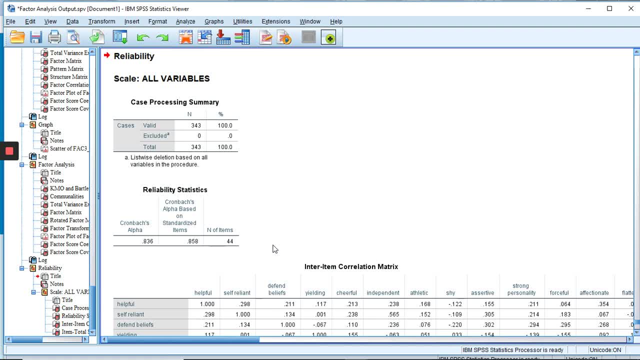 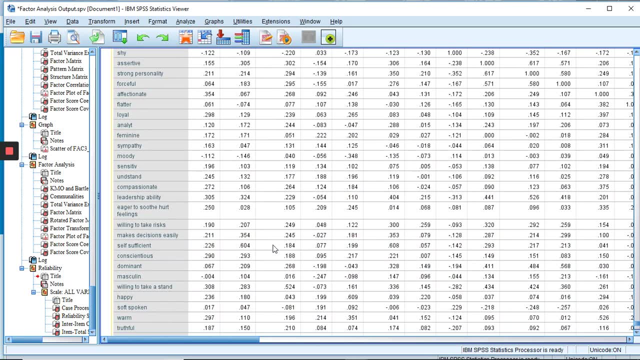 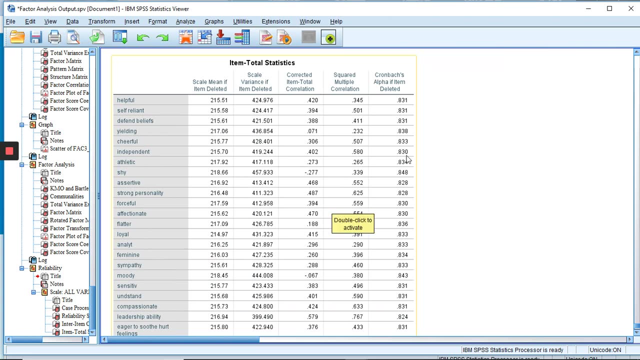 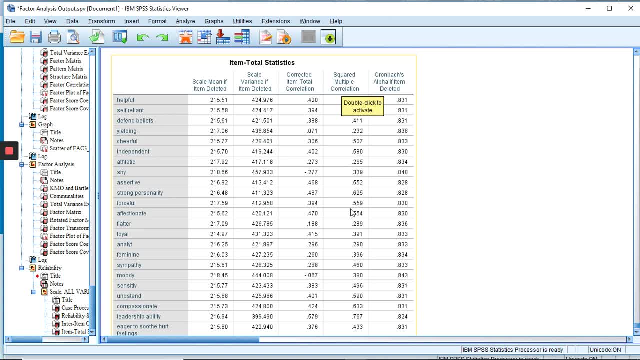 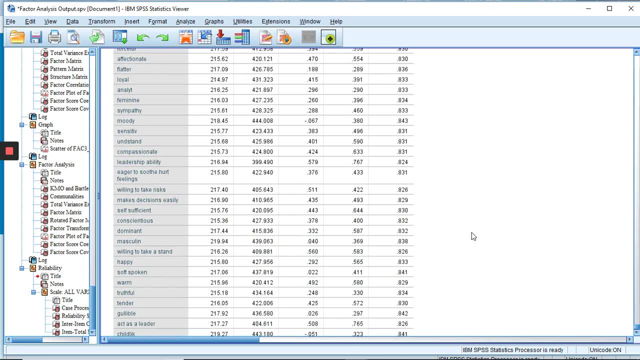 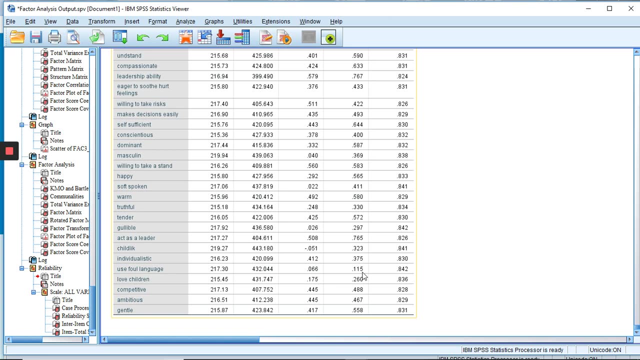 Here's the squared multiple correlation, which maybe that's a way to get it for the other thing, I don't know. I don't know if that works as opposed to the tolerance, but you see, this one is the lowest here. So basically, for the reliability or the internal consistency of factors, higher SMCs indicate well-defined factors. 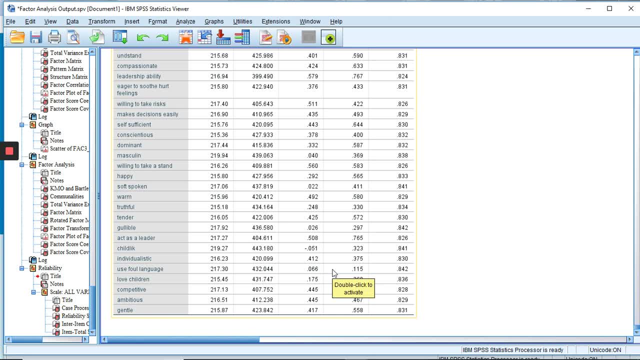 So this is our lowest one use of foul language, which I think is the lowest one. So this is our lowest one use of foul language, which I think is the lowest one. So this is our lowest one use of foul language, which I think is the lowest one. 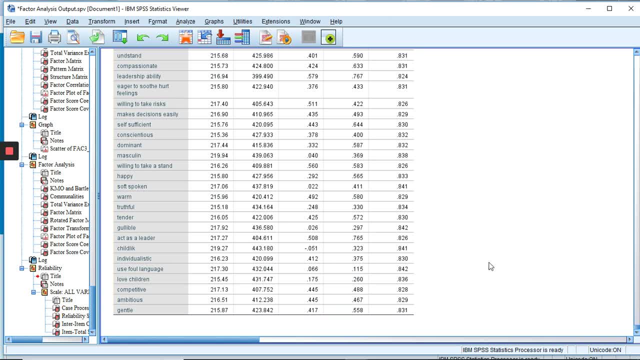 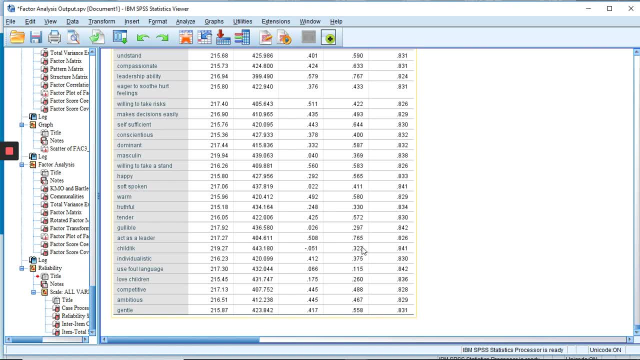 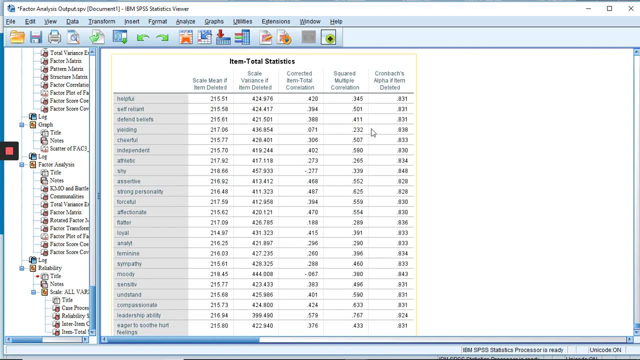 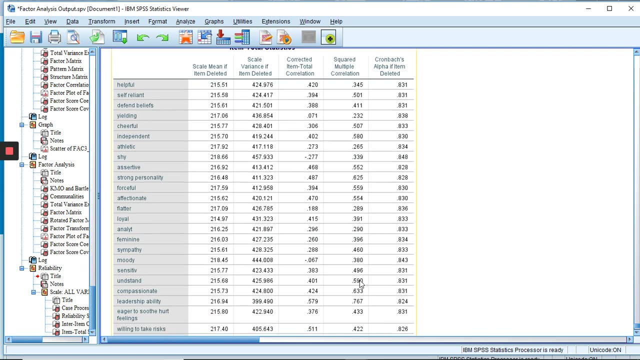 But let's look at all the other values and nothing else looks particularly low. You got a couple point two something, but you know otherwise it seems to look OK. So that's your evidence right there that there's some internal consistency, And you would just paste that output in to show. 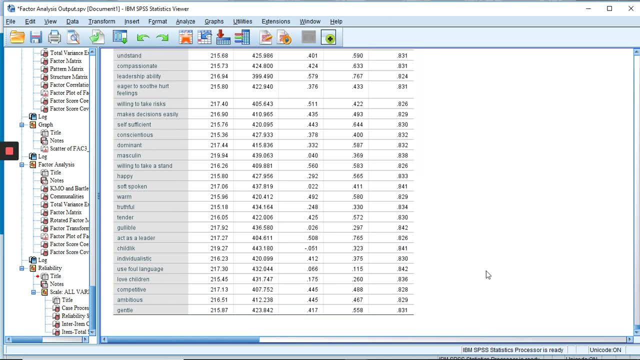 that you found that, so that would be a good sign. and the other thing you can mention: I think in the they also talk about the complexity of variables in in Part C, there on the on the list of the checklist for factor analysis. so if you wanted to talk about complexity again you could mention the specific variables. 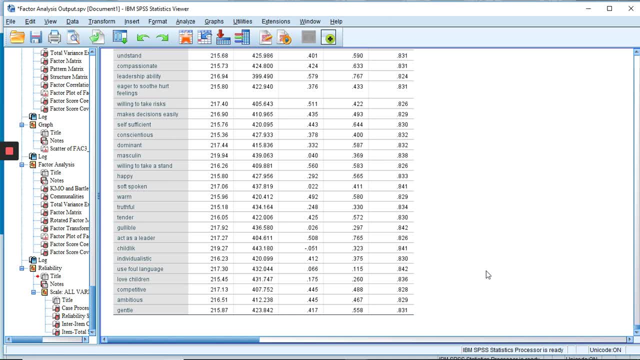 I think we said warm, gentle and independent that came up for us, that were on more than one factor, so you could mention that those were too complex and would need to be kind of reduced in some way to maybe make a better inventory, and that's it. so yeah, I don't. I didn't do any other of the 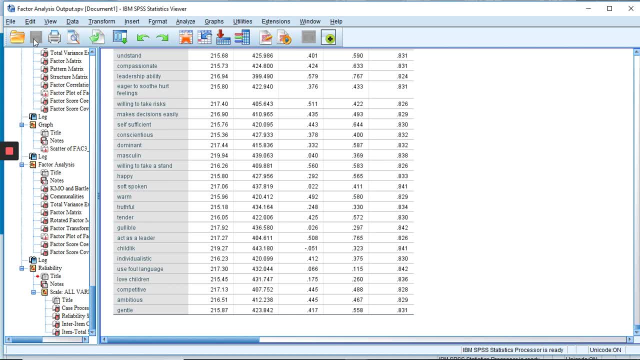 additional analyses so I can't explain them to you. um, if you look at the write-up, it's pretty short and I actually wrote a little bit more about what I did in the beginning to you know: delete the outlier cases and look for normality and all that stuff. it's getting late now, so good.